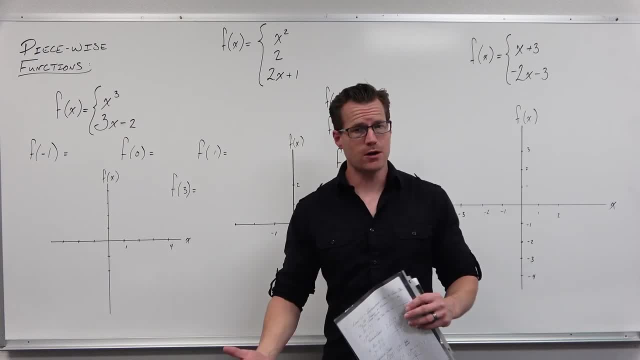 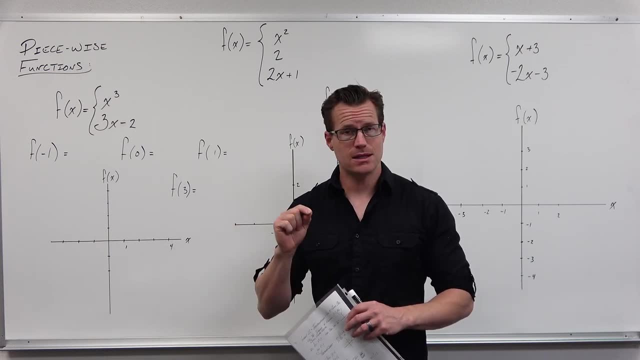 so what a piecewise function is? a piecewise function number one? it's a function which means for every one input you get exactly one output. that's key. that's an important thing. so how piecewise functions look is a little bit funny. we see a function. we have this little curly bracket. 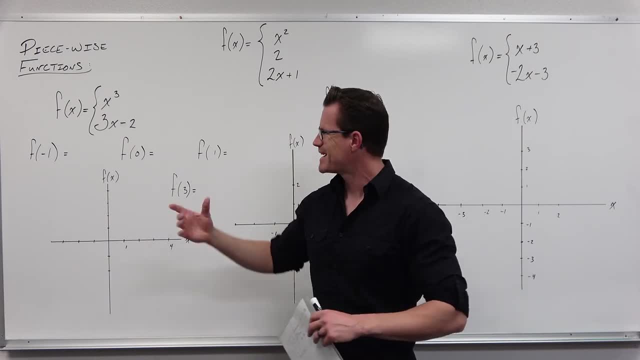 saying: hey, it's, uh, it's both of these things, oh great, so i'm just gonna take numbers, plug them into both of them. no, no, don't. no, don't do that, because if we take any sort of an input and plug it into both of these little pieces of your function, piecewise functions, it's going to give us two. 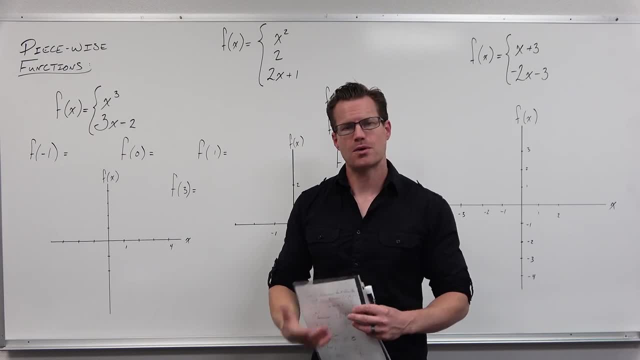 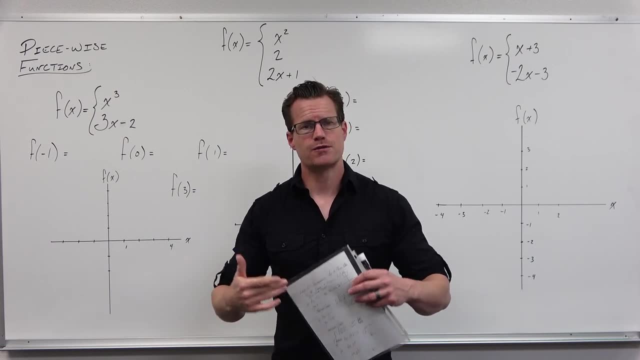 different outputs from one piecewise function to another piecewise function. it's going to give us for most of our inputs that's a problem. so every one of the piecewise functions i've given you right here is is really not defined fully. so what a piecewise function says is sure you got this. 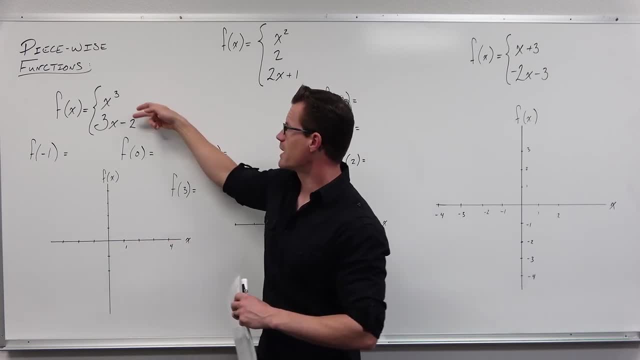 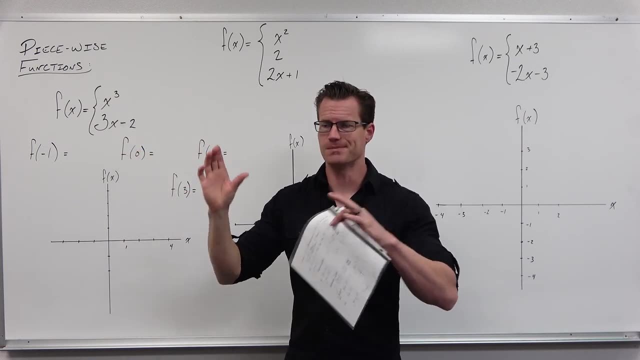 thing. that's a function. it's going to give me one output for every input. i'm going to give you directions on what to do, but then also directions on how to use each piece of it. so a piecewise function gives you a function in pieces. you can only use one piece for certain. 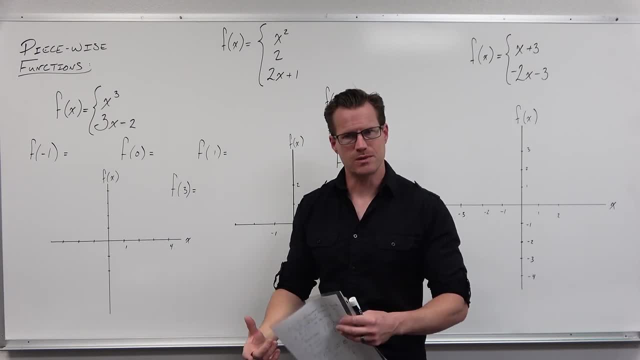 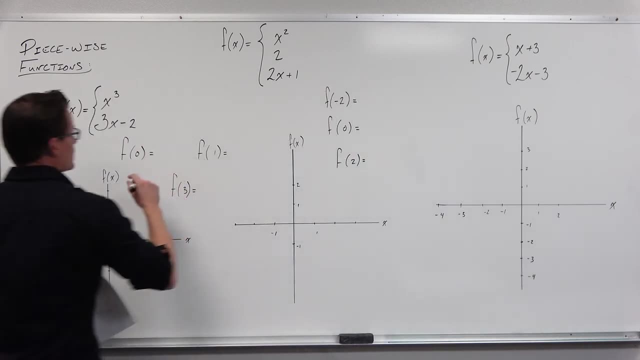 sections or intervals of your x-axis. that has to be defined for you. you don't just get to make a make it up, so i'm going to tell you what these pieces are. so here's the the domain for these functions. it says this function is going to be x cubed. that's the piece of it. but you're only going. 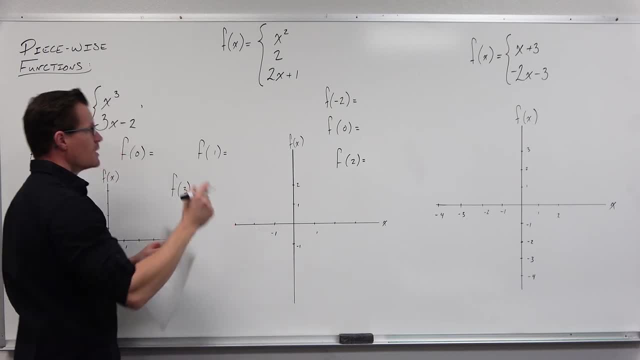 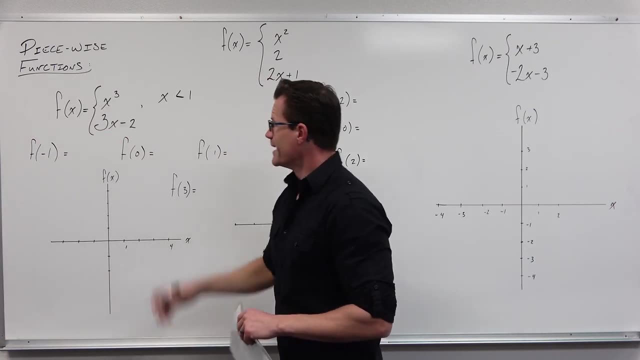 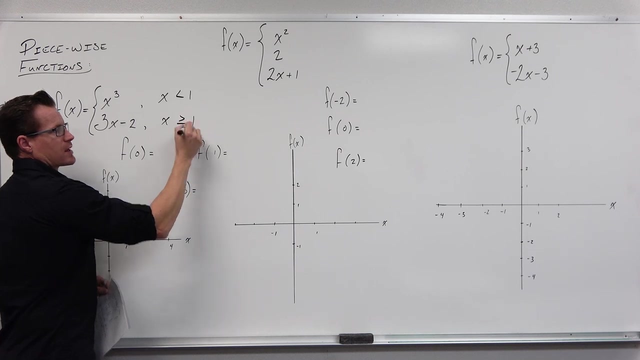 to use it for a little bit of this graph or some some interval of this, this x-axis when your x's are less than 1.. that's when you get to use x cubed for this function. it's going to say: i also want to use 3x minus 2.. it's going to use 3x minus 2 anytime your x's are greater than or equal to 1.. 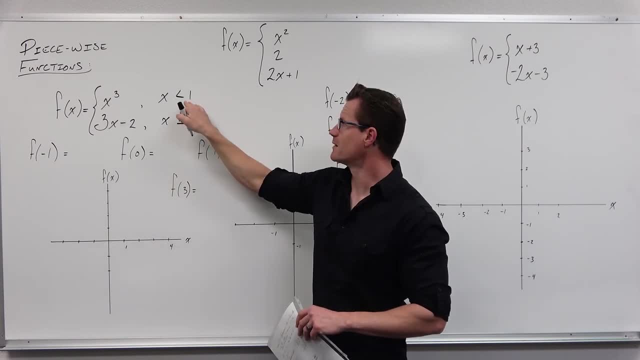 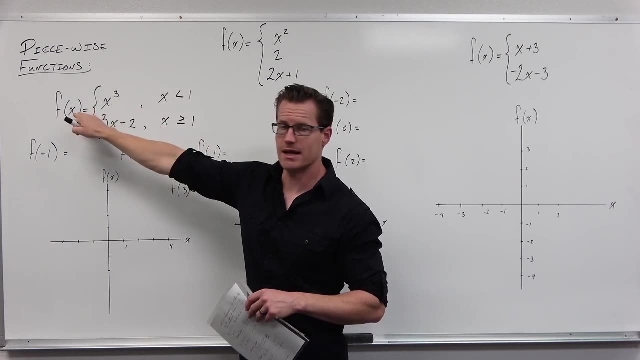 separating value on your x-axis. this says: for anything less than one, strictly less than one, you're going to use this piece, this thing, this function, to define f of x for any value, one or more, so any x value that's greater than equal to one. you're going to use this piece to define that. 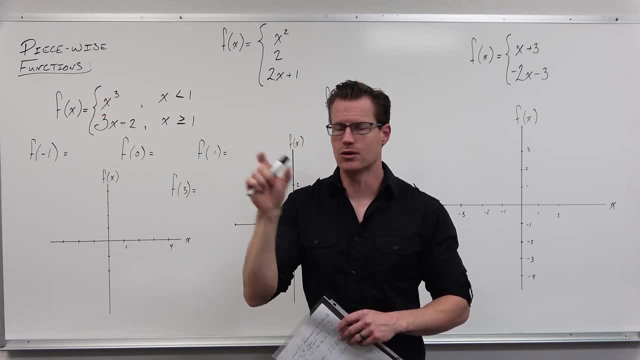 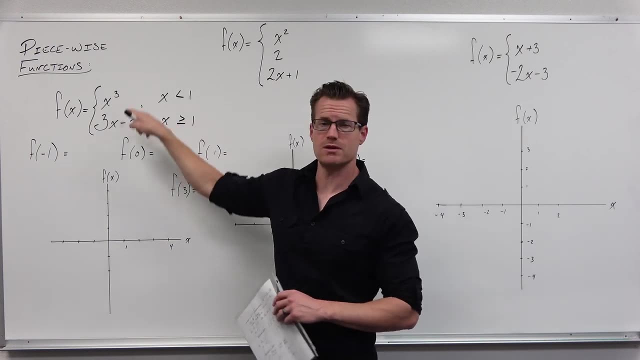 function. that is how piecewise functions work. it gives you the function in little pieces that are not the same piece. the main thing here: please don't ever take a value and plug in one value to both of these pieces. what that's doing is that's breaking the fact that this thing is actually a function. we need one output for every input. 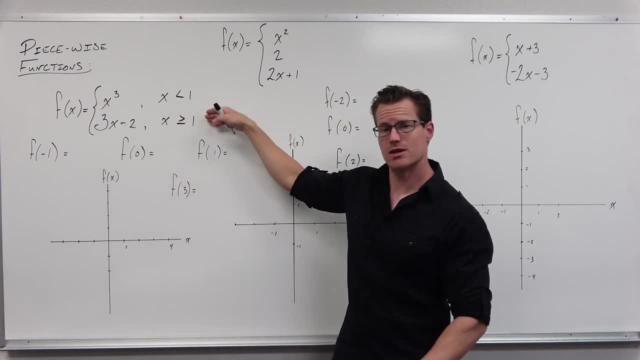 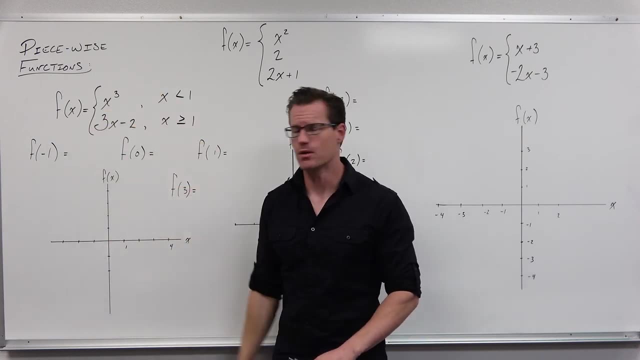 so here's the what you do, here's the when you do it. this right here, this is your domain. this is, this is where this function is defined. more than that, it tells you when to use each of these pieces. let's try it. we're going to plug in a couple values. i mean four values. we'll do the. 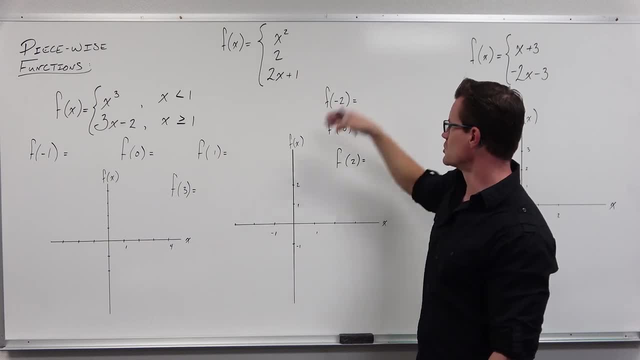 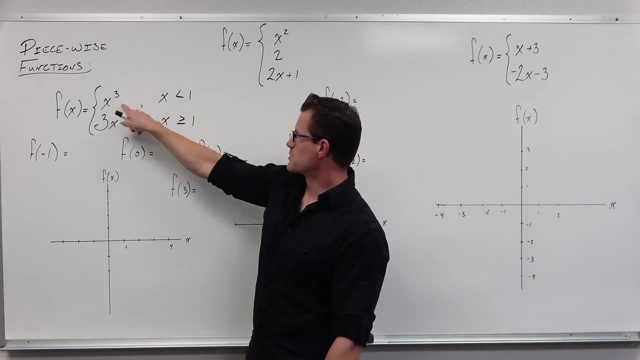 same thing over here. i'll give you some directions of the domain for a piecewise function. we'll plug this in and then we're going to go back, we're going to graph them and that's. that's pretty much it. so if we use this piece, whenever our x is greater than or equal to one, we're going to. 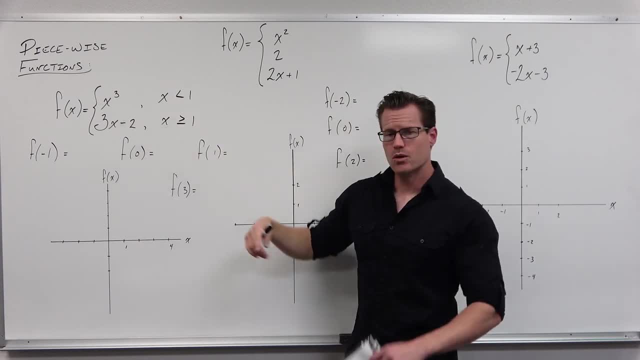 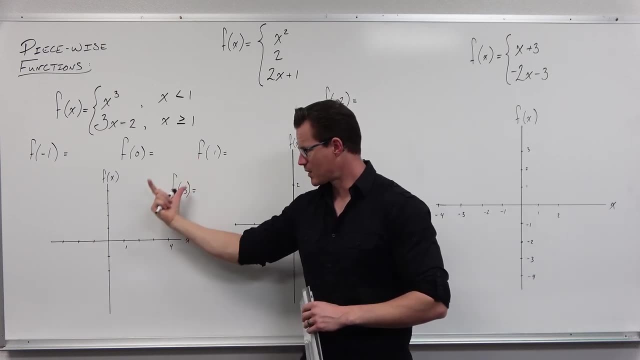 use this piece whenever x is less than one. we use this piece whenever x is greater than equal to one. we should never, ever have a time when these cross over. graphically, that means our graphs will never cross. we'll never have the same p, same graph. sorry, never have two different graphs on the same. 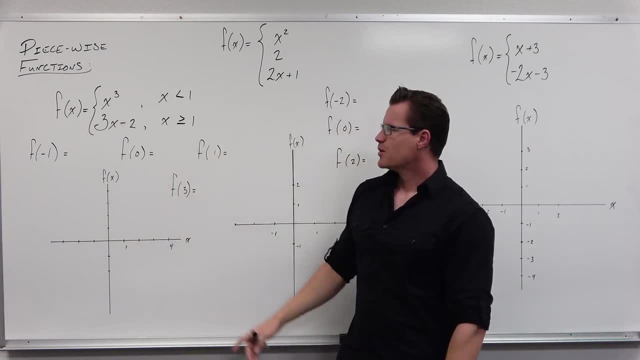 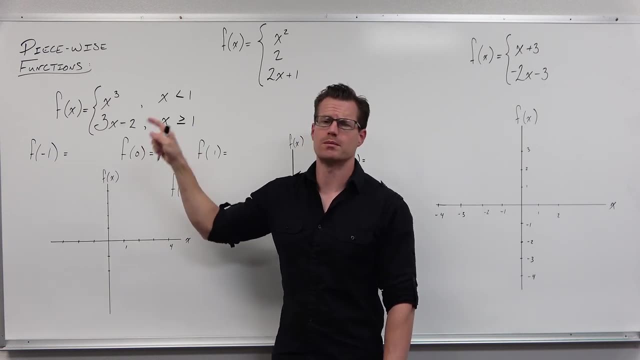 interval over x-axis, how we use it practically to evaluate. we just have to understand that these are the values, that are our inputs. we need to notice where they go and then plug them into one and only one piece of that function. so let's look at it. f of negative. one asks you look at the function f. 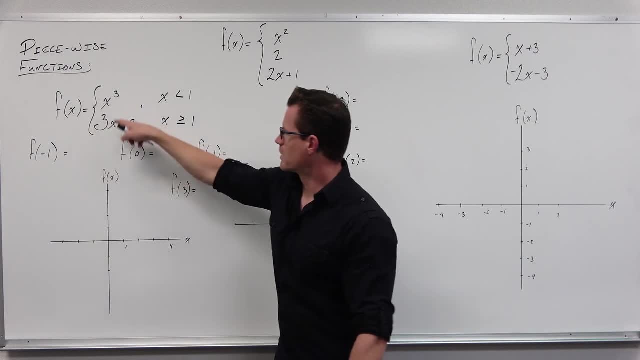 got it? uh, i want you to evaluate negative one. you go: okay, eeny meeny miny, no. no, eeny meeny miny, no, don't do that. we look at negative one and we say: where does negative one fit in our domain? negative one fits. 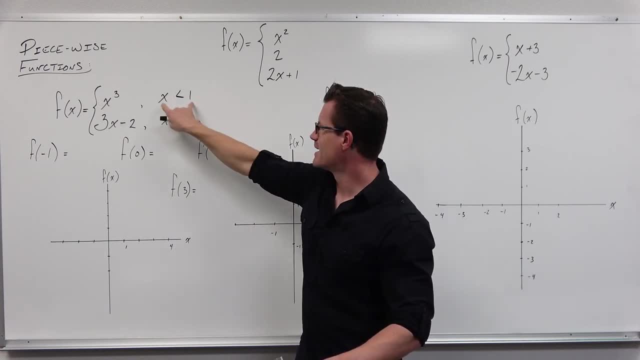 in this part of our domain negative one is less than one. it fits that. that direction, that well, this interval of your x-axis. so it says i'm going to plug in negative one where it actually works, i'm going to plug it into just this piece. it doesn't qualify here, it's not fitting that. 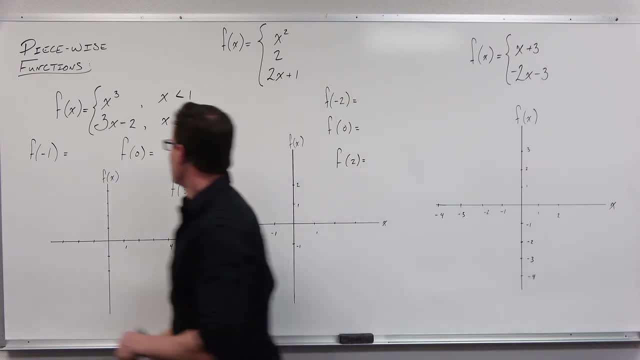 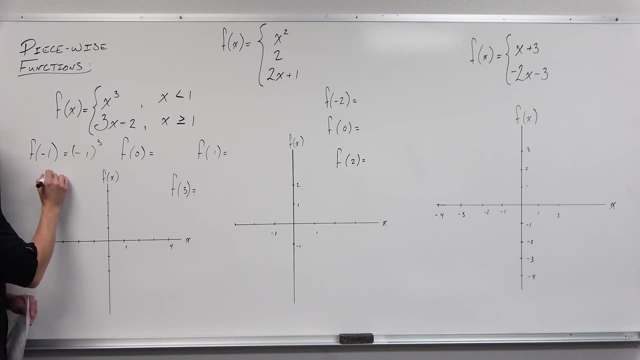 condition it doesn't fit this domain, so we say one fits here. that means that i would have negative one to the third power- i'm using just this piece- and we would get an output of negative one. that means you had an input of negative one and you had an output of negative one. that's a point on this graph that needs to make sense to. 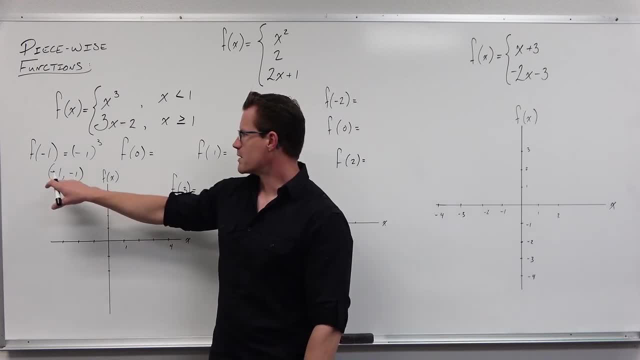 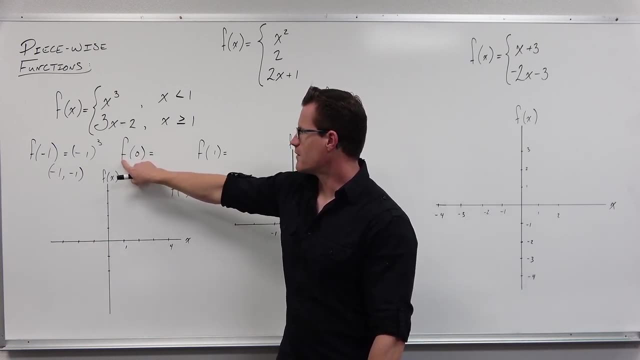 you when we graph this thing in a little while we're going to notice that that point is going to be on that graph. how about f of zero? f of zero says all right, well, look at your function. says: look at your function, f got it plug in zero. that's your input. okay, how do i do that? i use one of these. 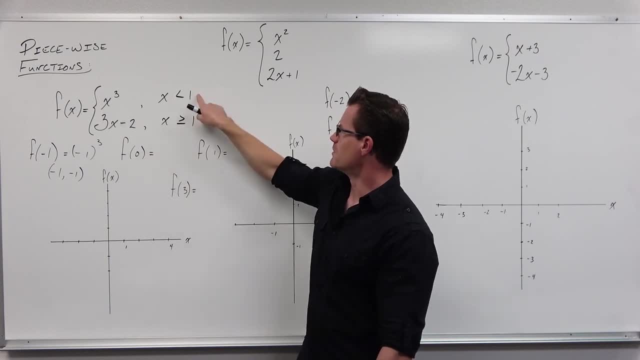 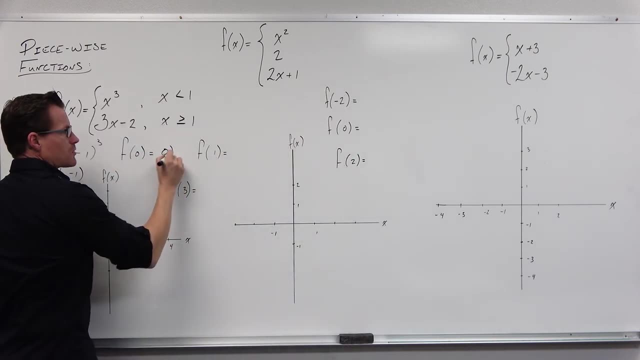 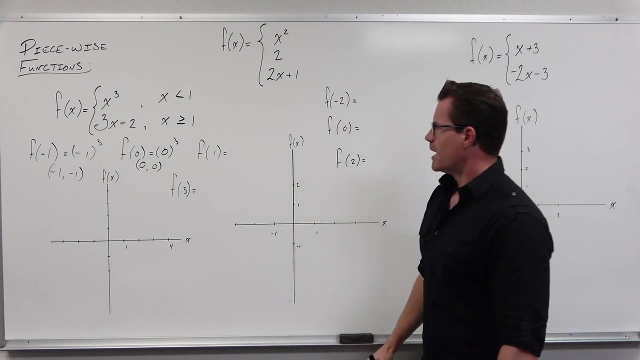 depending on where it fits. in my domain, zero is still in this interval of the x-axis- less than one. so i would still use just this top piece, not both. that means that i have zero. to the third power: i plugged in zero, i got out zero. that's another point on our graph. how about one? well, you know. 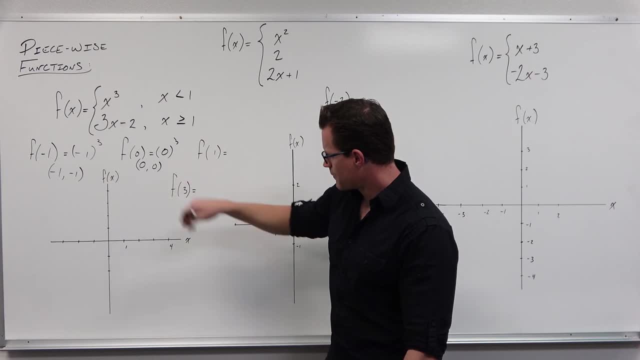 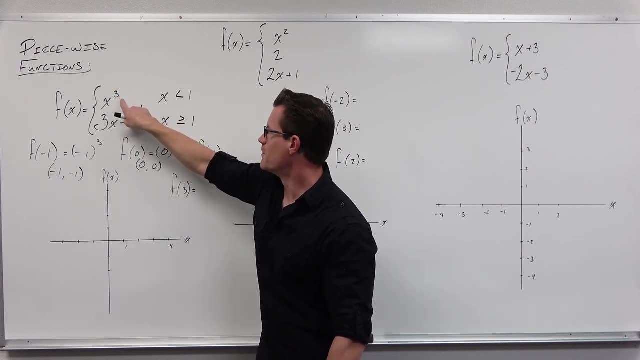 let's skip that one, let's skip, let's go to three. so f of three evaluate the function for three. here's our function f. our input is three. i'm going to be using these two things to define my function. is is given over here, so i'm going to look at three and say: is three on this interval of the. 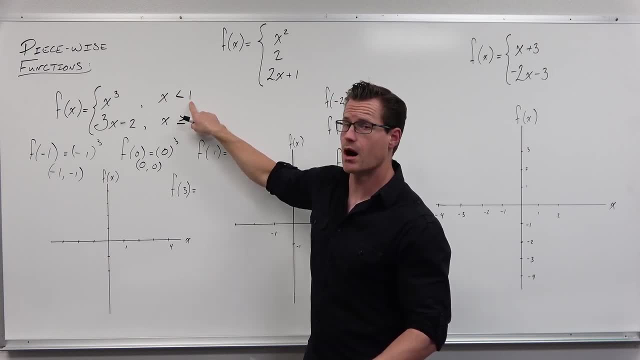 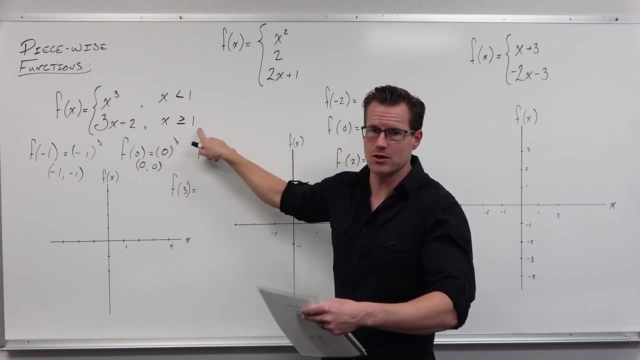 x-axis is three in this domain? no, three is not. three is not less than one. is three in this interval? the x-axis three in this domain? yeah, three is greater than or equal to one. it's, it's namely greater than one. so it says: you are defined. this, three is defined for this, this domain, this. 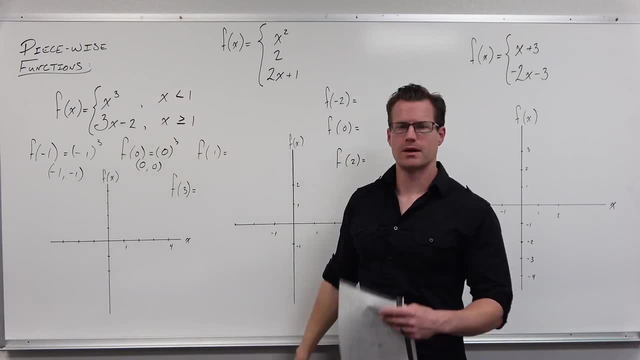 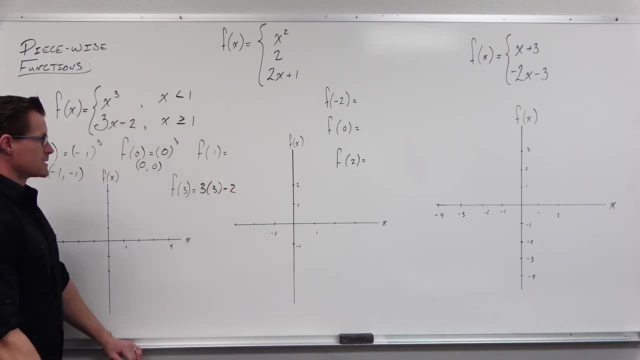 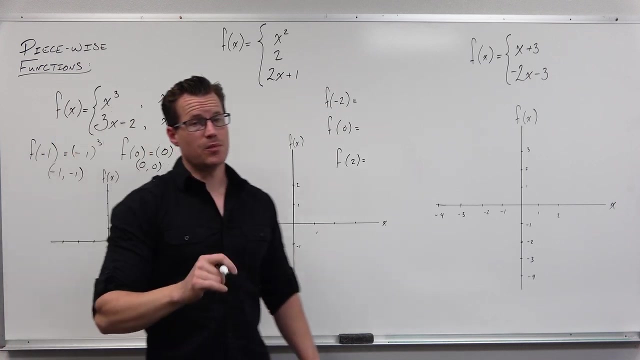 three says you would use this function, which has this domain, plug in three. so when we have three times three minus two, let's see: uh, three times three is nine. nine minus two is seven. we've plugged in three, we evaluate for three. we got an output of seven. that is a point that is going to be on this function. that needs to. 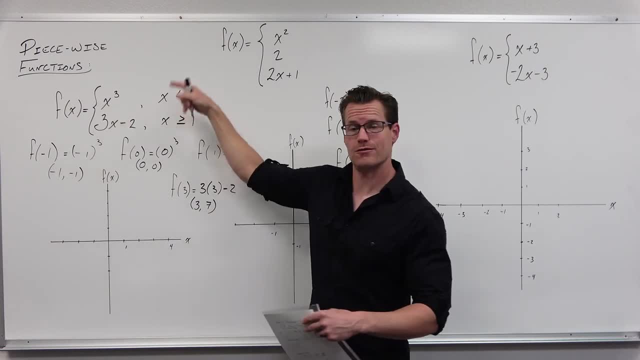 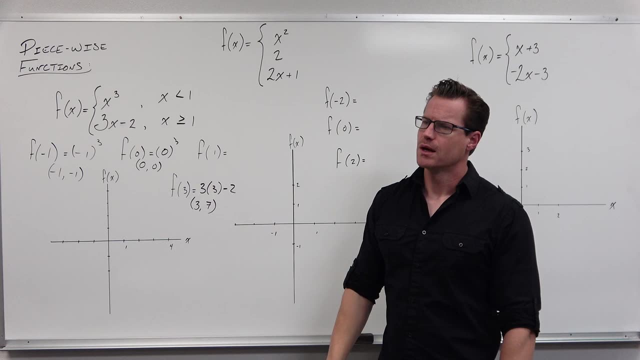 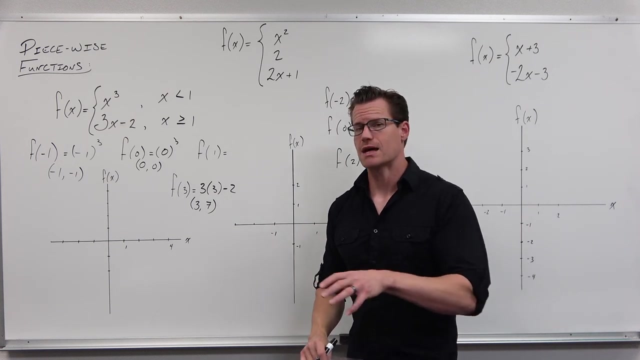 make sense. notice how you're just taking one value, finding out where it fits, and plugging in to one of those pieces. never, ever both. well, you know what about one? doesn't one fit in both? no, it can't, and and you will never see an equal sign on more than one of these intervals. you don't even have to have. 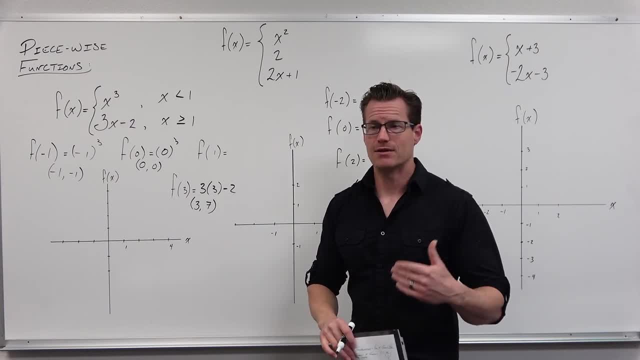 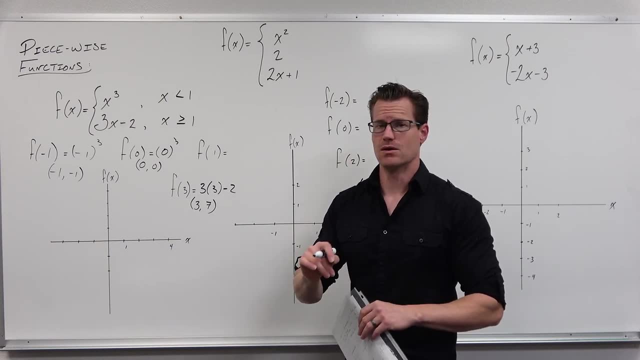 an f of one. it doesn't have to be a continuous graph. this won't be. it doesn't have to have an output. sorry, it doesn't have to have every input on your x-axis. that doesn't have to be the case there. if it does, though, if it does have an uh, this, this interval, the x-axis, for which you have 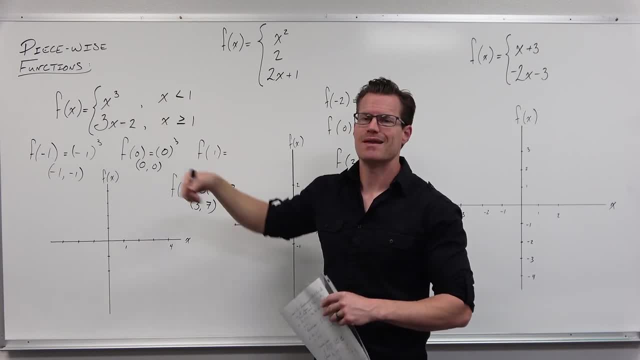 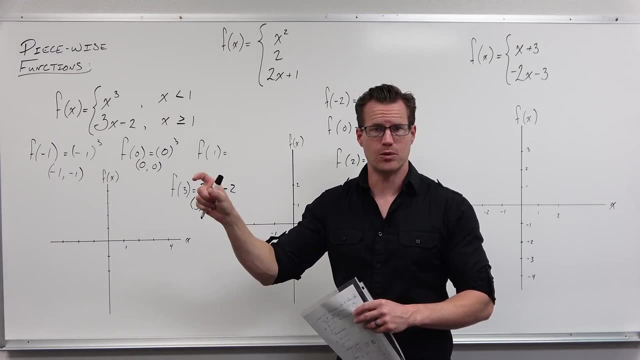 every single input. you can't ever have an equal sign on both of those domains. that would disqualify that from being a function. that would say you could plug in one or evaluate for one and have more than one output. that's a problem. so when you see this f of one, it's got a function that's going. 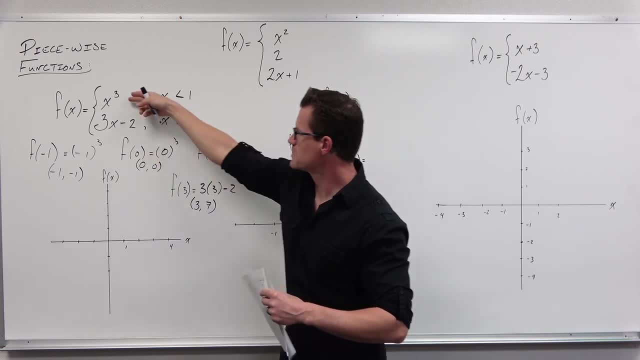 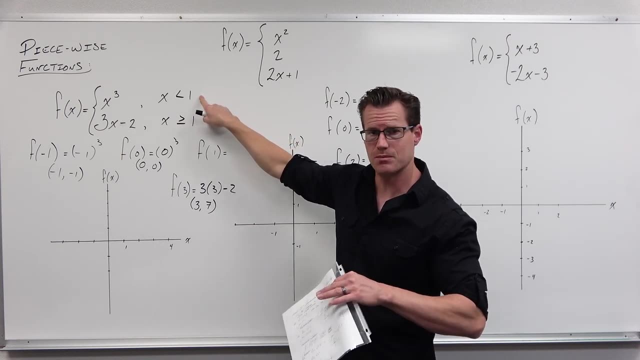 to fit in only one spot. so look at your function f, plug in one, no problem, use these pieces, but how? you use them as your domain. so let's say where's one fit. is one less than one? no, no, it can't be. it will never ever be the case on a function where you will be able to plug in one value to two. 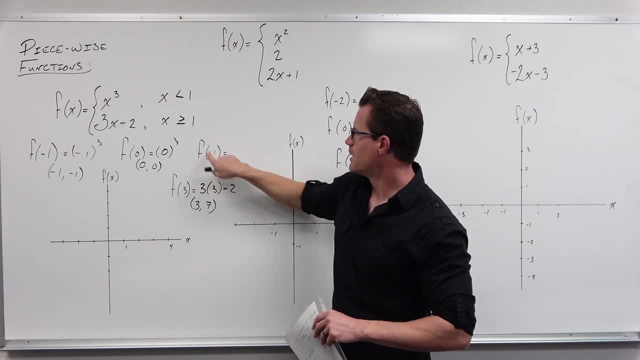 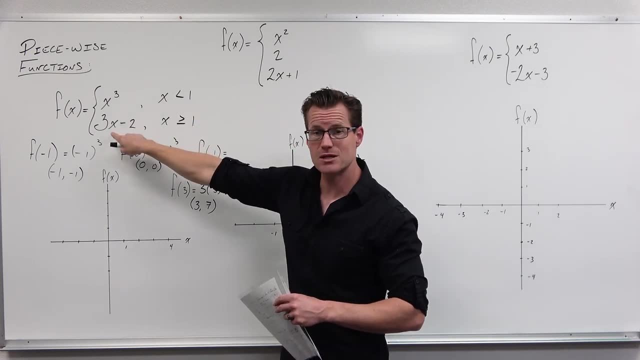 different pieces, it won't happen. so plugging in one says one is on the interval of x greater than or equal to one. this is specifically equal to one that says: oh hey, i fit in this domain, let's use that piece for which the domain is defined. that would be three times one. 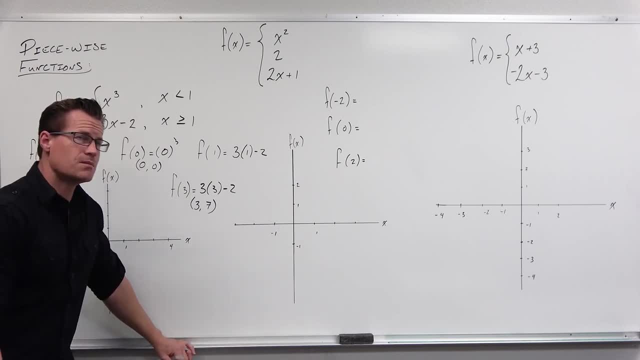 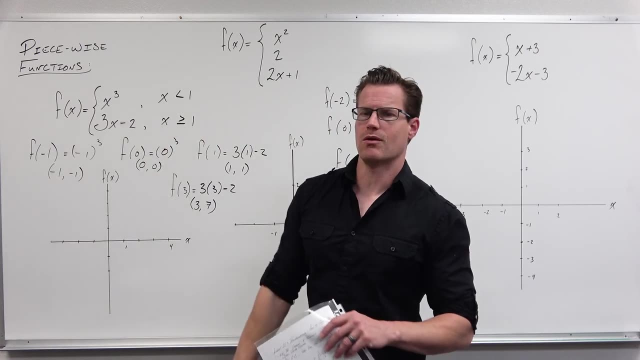 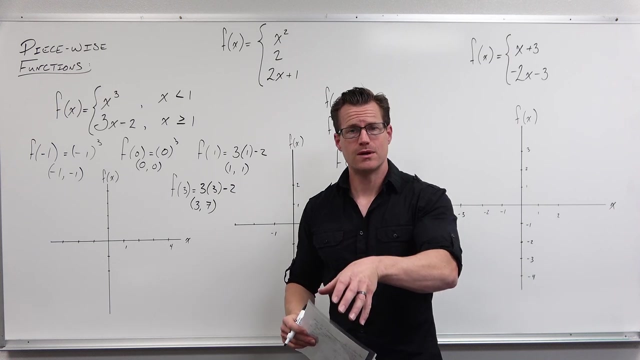 minus two, let's see three times one's. three minus two is one. i evaluated one. i got an output of one. these are giving me points on my graph. that is exactly how evaluation for piecewise functions work. just figure out the domain. we'll figure out where your input fits in your domain and use that. 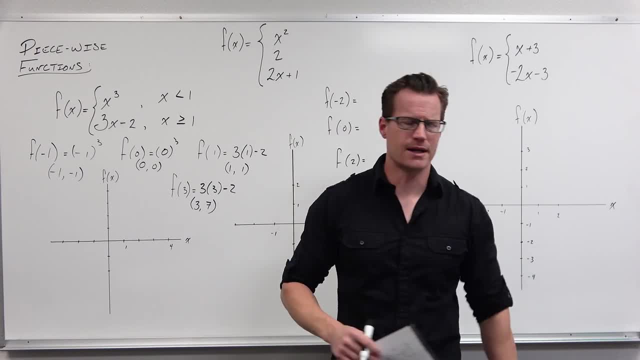 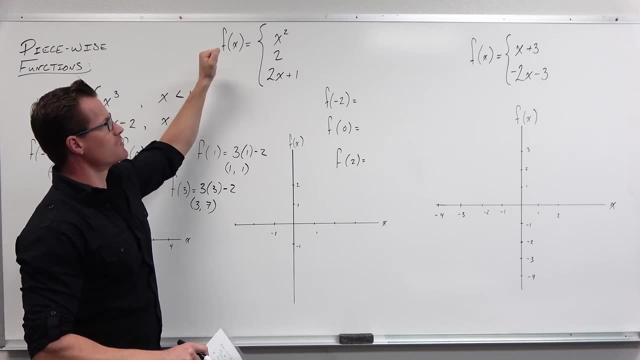 piece of your function for which that, that, uh, that domain is defined. next one: obviously this is incomplete. this is wow. i've got three different pieces that define this particular function of f. uh, i have x squared, i have two and i have two x plus one and it has to be given to you what um. 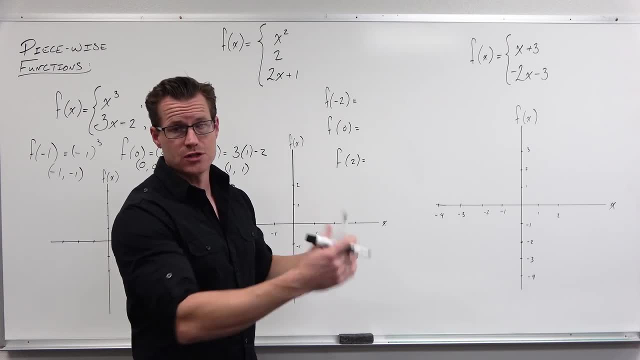 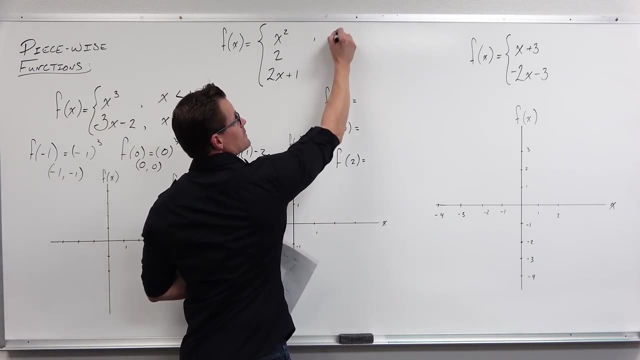 for what interval? the x on the x-axis that this piece of the function is defined. so basically what your domain is. well, let's say that x squared is defined anytime x is less than zero. that's an interval on your x-axis. mom, pause right here. can you look at your x-axis right now? you should be. 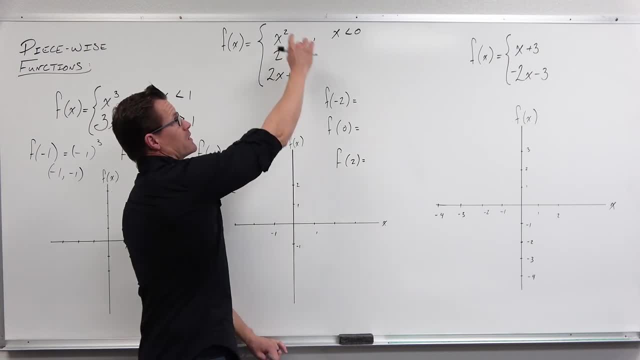 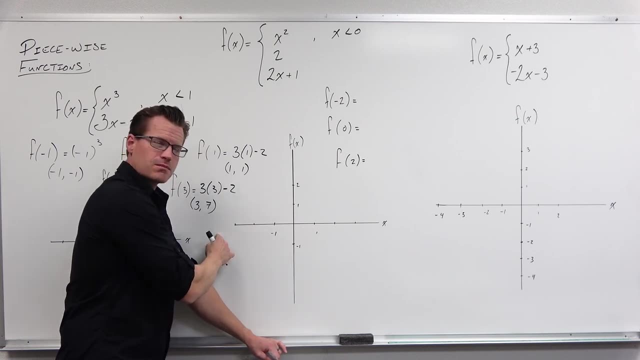 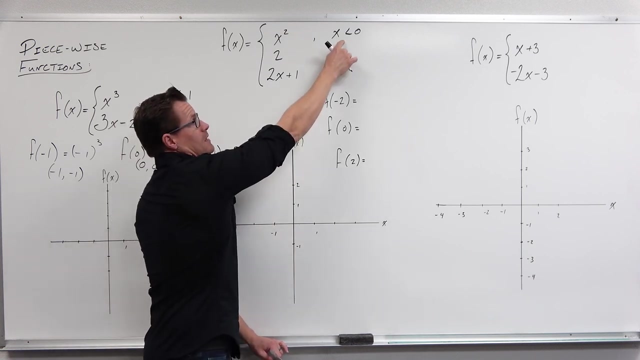 able to and say: the interval of my x-axis, for which this piece of the function is defined, x, is less than zero. that's this entire interval of your x-axis. that should be pretty clear right now that i'm looking here. that means when we get to graphing, we're going to look at this. 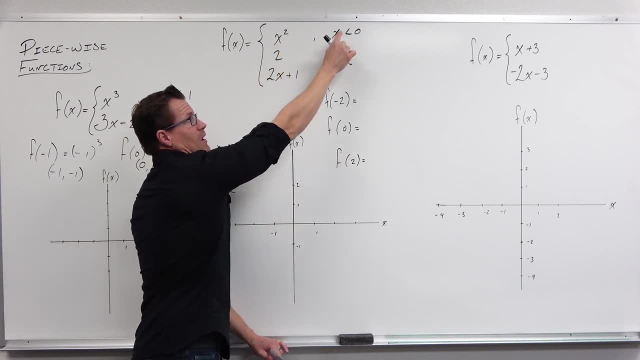 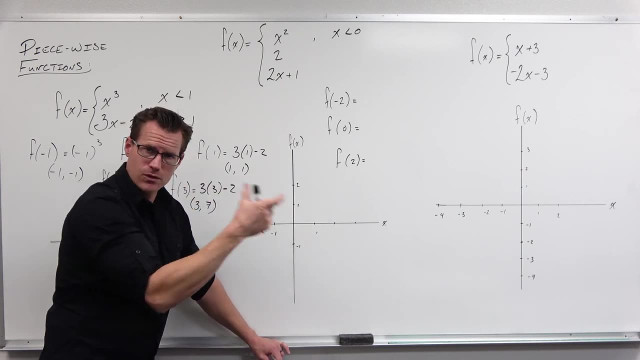 we're going to make a little separated line and say this piece is on that interval- and that's probably the best way that i know how to graph piecewise functions is separating my x-axis into intervals for which my functions are defined. my little pieces are defined and 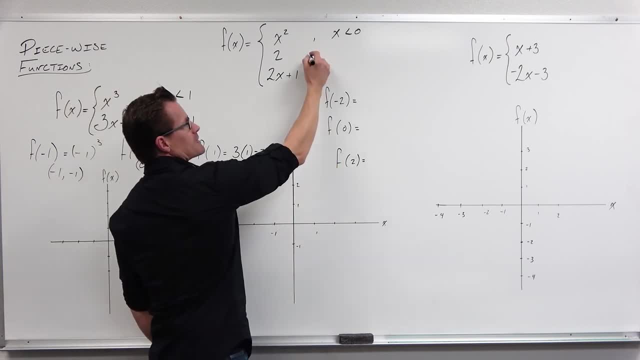 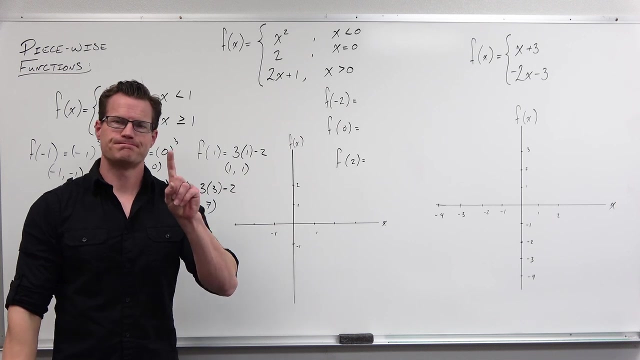 then graphing those pieces on those intervals. all right, moving on now. this says that you're going to have the output of the function be 2 anytime x is just equal to 0, and you're going to use the piece of the function 2x plus 1 anytime x is greater than 0.. notice: real quick, i only have 1 equals. 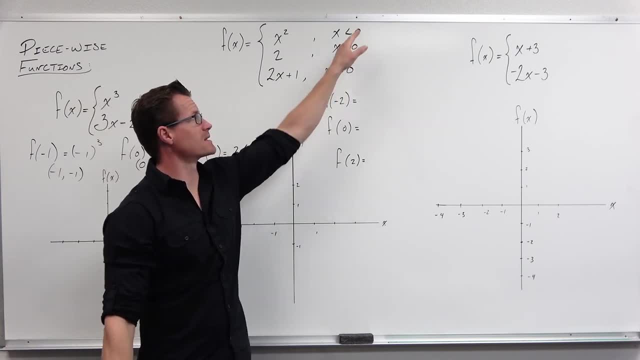 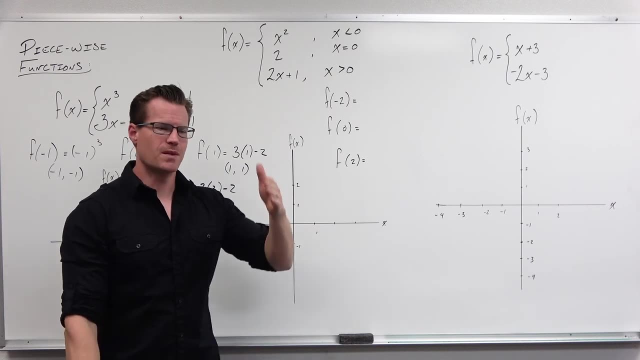 only 1.. i'm using the entire x-axis. this is less than 0, equal to 0, more than 0. therefore, i can only have one equal sign. now, could you have it like something kind of weird where you went from maybe negative 5 to negative 2 and you skipped a few points and then defined it again from like 7? 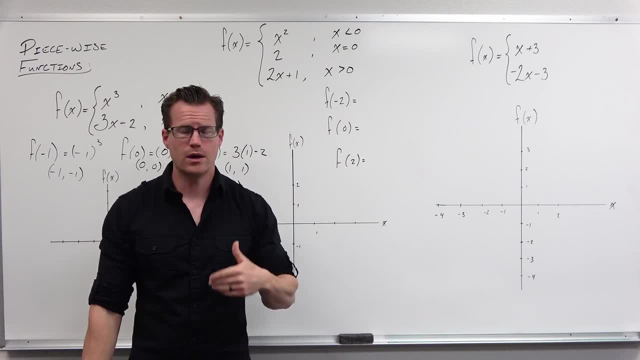 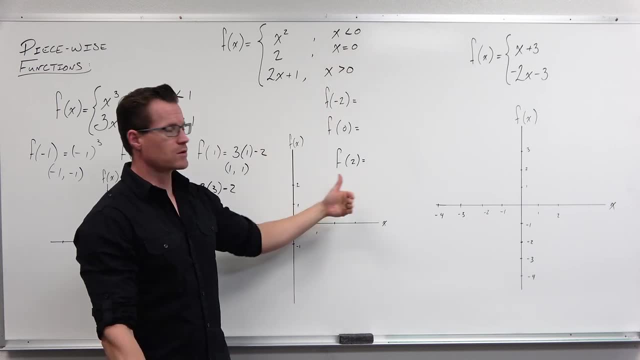 to infinity, sure, and then you could use more than one equal sign. but if you are having the same number, your same, i call it separated number, boundary number, whatever you want to do on your, your x-axis, if you have the same number here, you can't ever let one input give you more. 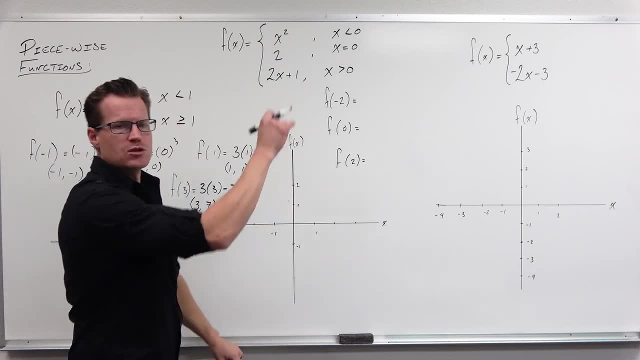 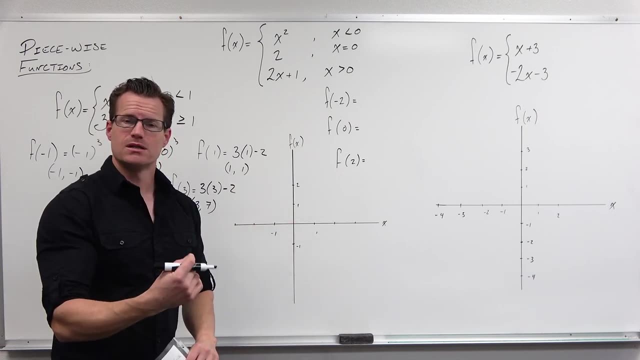 than one output. just check for that. make sure you're not plugging in one value to more than one piece. that should never, ever happen. so let's see negative two. this is: look at your function. plug in negative two and just see where it fits in your interval and x-axis- your domain- negative 2. 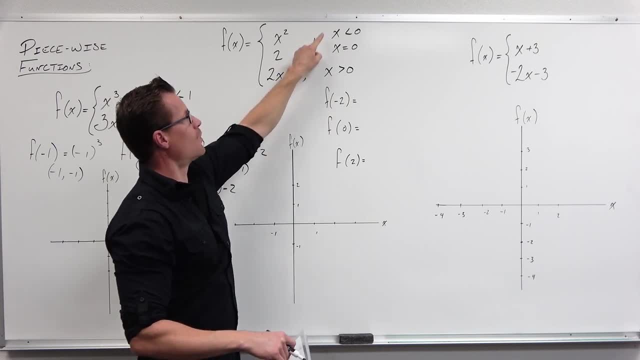 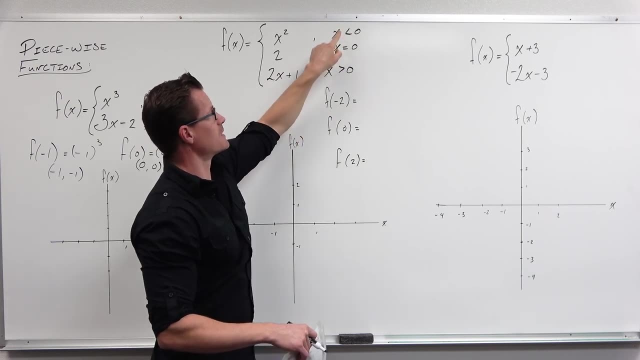 let's see, it's not equal to zero, it's not more, it's less than zero. i'm going to use only this piece of the function for which this domain is defined and my input fits in that domain, so i'm going to plug this in here. say: negative 2 squared. 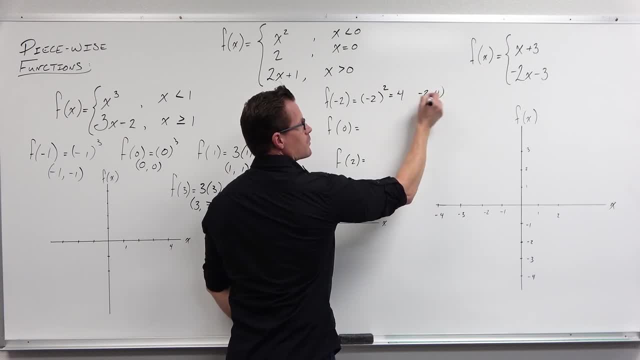 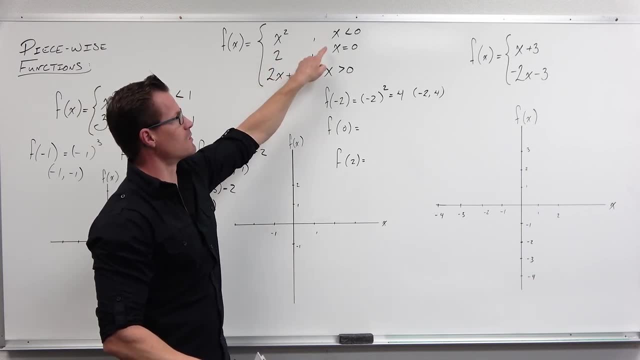 is 4.. that means i have a point, negative 2 comma, positive 4.. that's going to be a point on this graph. i'm going to graph a little bit: zero. well, zero doesn't fit in this interval. it's not less than zero, it's not greater than zero, it's equal to zero. and this gets a little funky. it says well: 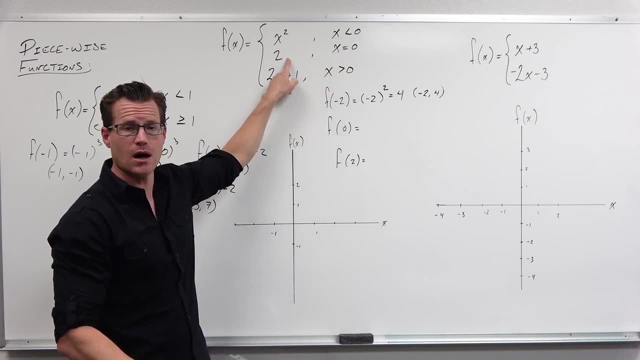 what do i do? i have nothing to plug in for. yeah exactly, it's called a constant. it means: no matter what you plug in, you're going to get out two. well, specifically it says: if you plug in zero, you're going to get out two. it's only defined for. 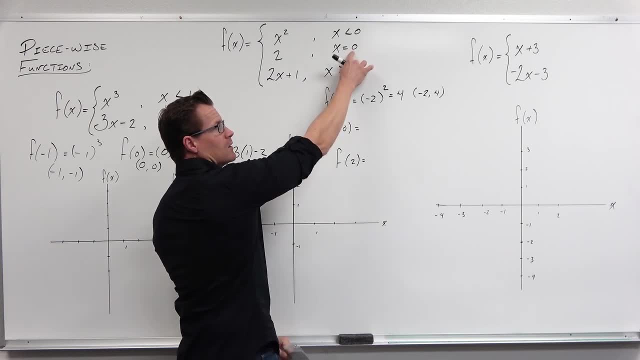 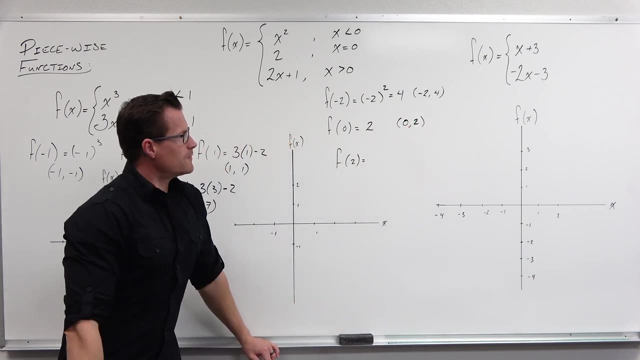 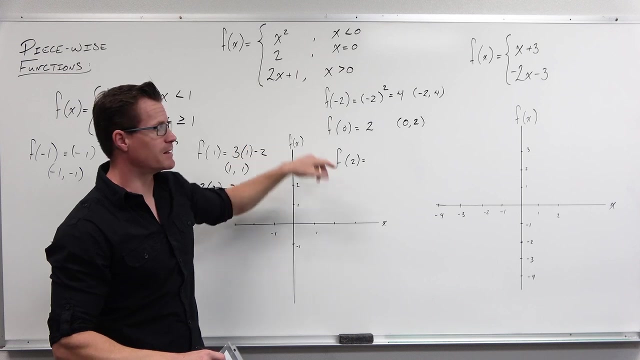 one input value. this is defined for the input value of zero. hey, i have an input value zero. it means i get out two. that's a point zero. comma two for f of two it's not less than f2 is not less than zero. it says my input values have to fall in one of these intervals. in x-axis, my domain says 2. 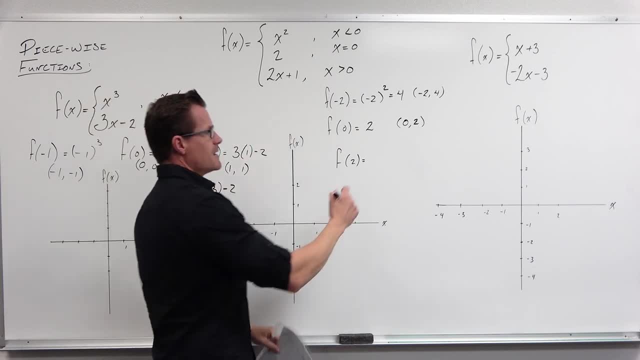 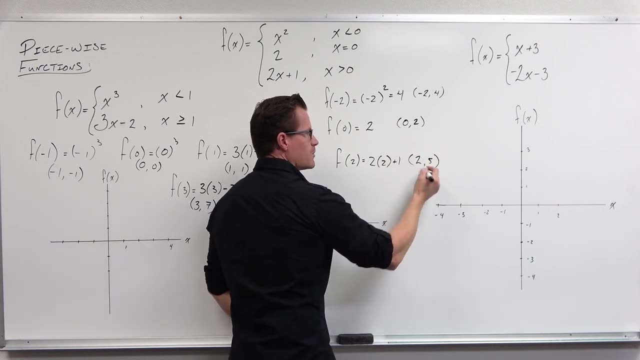 equal to zero. two is greater than zero, so i would use just this piece. this is two times two plus one, that's five. so we're going to plug in two or evaluate for two and then give us an output value of five. every input must have one output value. that's what a function means. right now we're 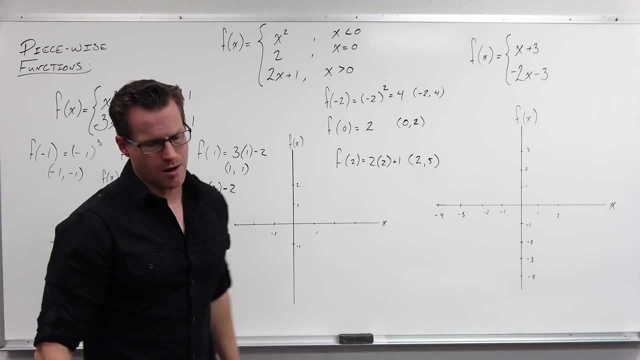 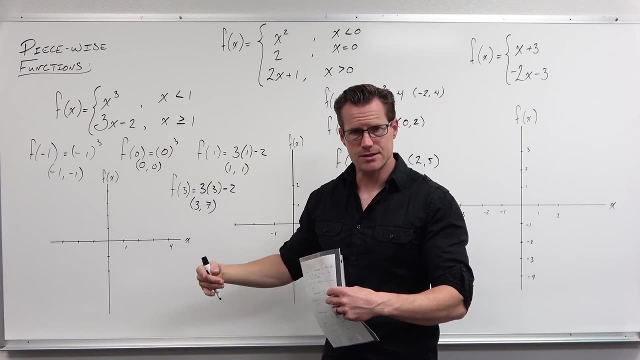 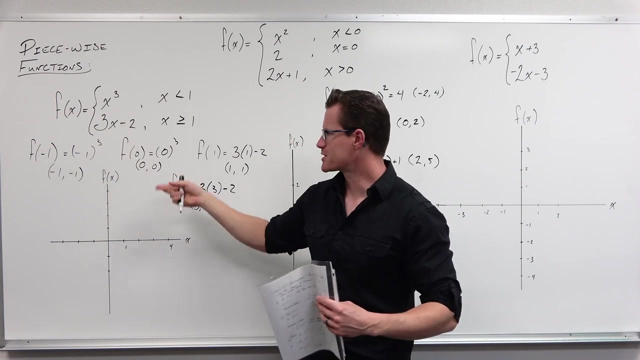 going to transition to a little bit. we're going to graph these, so what i'm going to talk about when we graph them. so i'm going to talk about how our domain is always based on the x-axis. well, we're going to do that. if we separate our x-axis into intervals. we kind of did that when we were 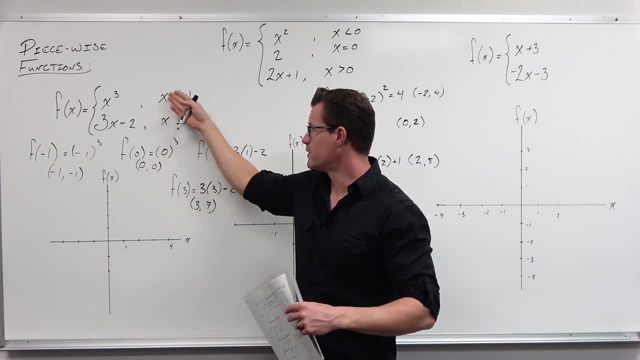 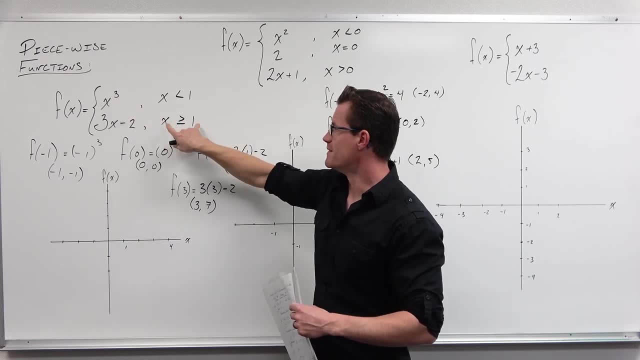 evaluating right? we just said, yeah, it separates it: x number, x value and input can only fit in one of those intervals. we're going to do the same thing. so we're going to say, because this is the domain for that piece of the function, and this is the domain for that piece of the function, if we 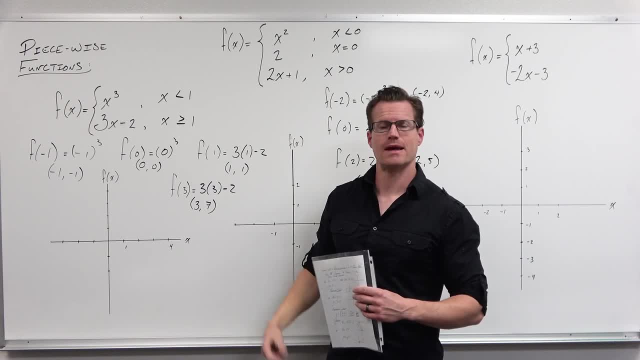 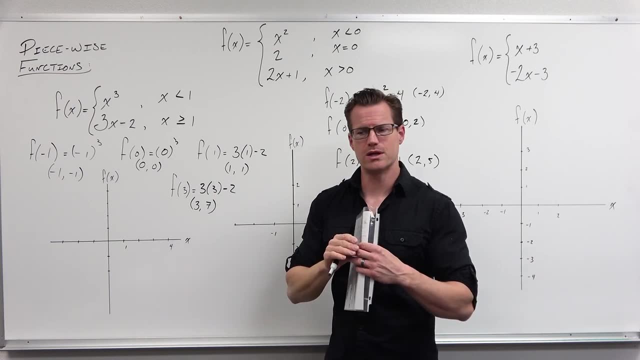 separate our x-axis and say: that function is only defined on that domain, that interval, this function is only defined on that domain, that interval. then we have a very clear marker on our graph for when we use one function versus the other, one piece of the function versus the other. so i'm going to 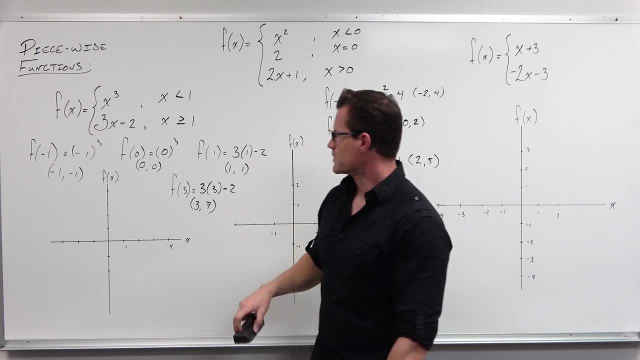 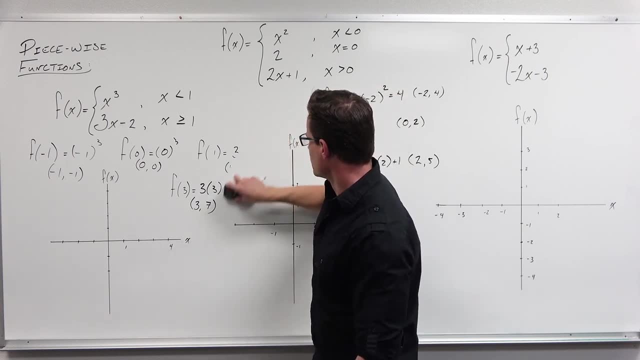 show that to you right now. um, i'm going to erase the our values. we really don't need them all that much. i want to keep. i don't want to keep any of them, so let's go ahead and erase those. now. what we're going to do is i'm going to show you the kind of lettered way to graph a piecewise function. 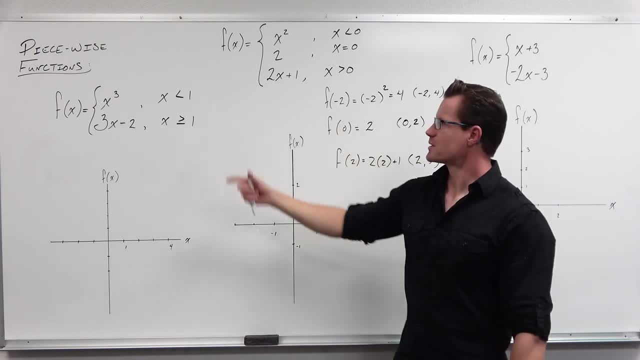 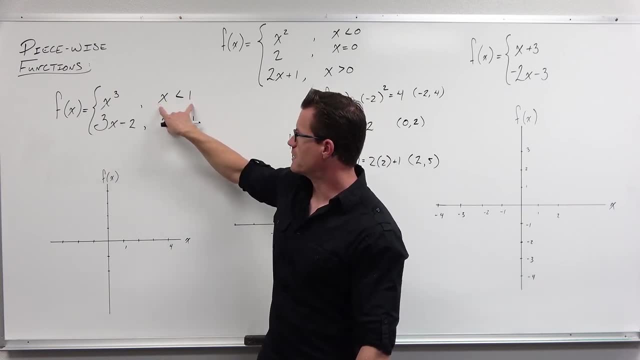 so here's- here's what i do. here's how this works for us, because our domain separates our x-axis. domain is always an x-axis idea. our domain shows us that if we separate our x-axis from our domain, for what interval we use each of our pieces of our function. so what i like to do is i'll take our 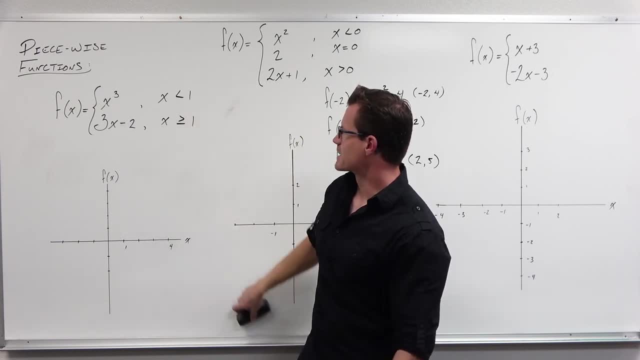 what i call a boundary number or separating value, and i go to my x-axis and, all right, this is defined for less than this value this function is defined for, or this piece of function is defined for greater than that value, but they have the same value. so i'm going to go to every single one of my 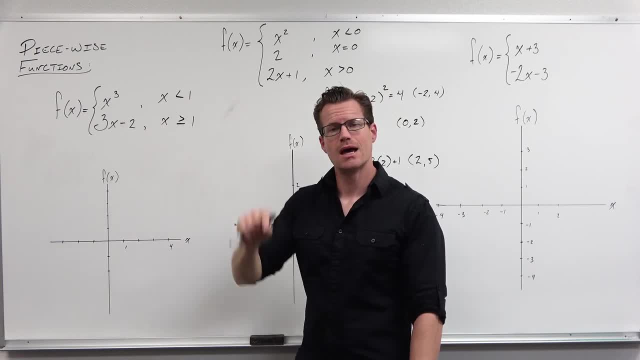 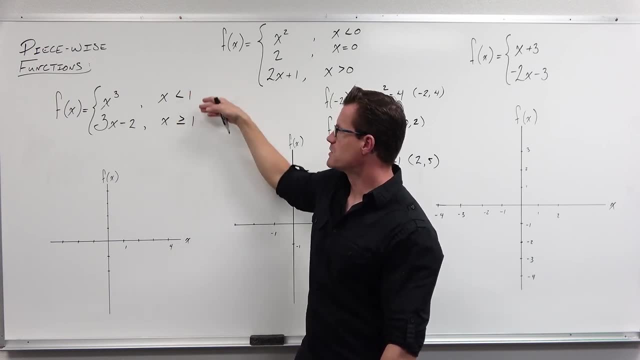 values that's given in my domain, my domain, for each of these pieces. i'm going to put a little vertical line, so i'm going to look at one. one is the only value on our, on each of these, uh, these domains, for our pieces, so i'm going to go to one, all right, 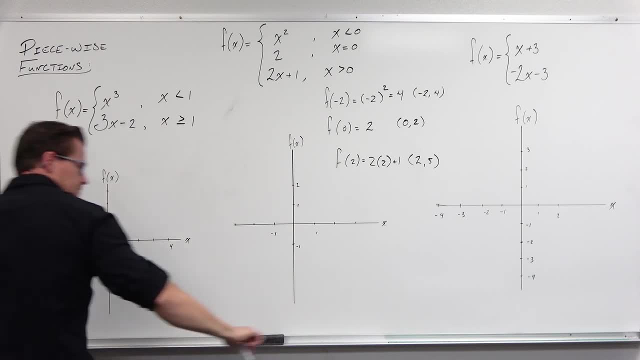 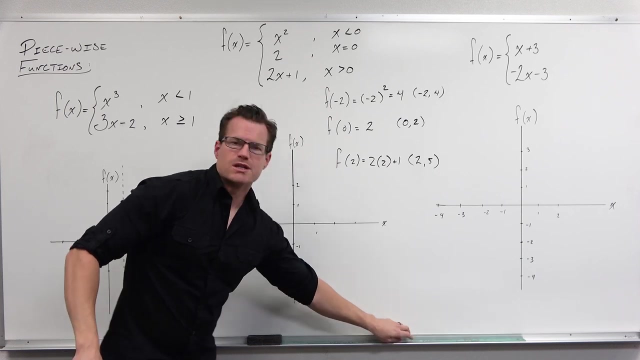 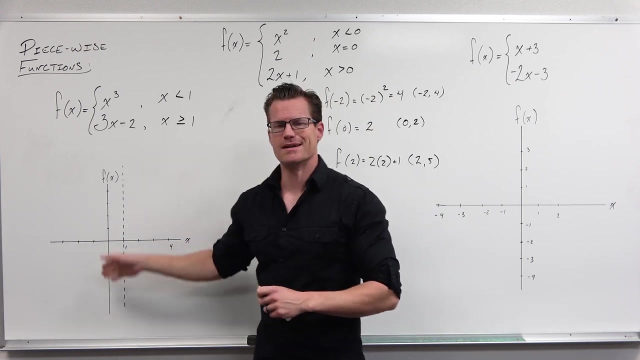 well, one has this kind of, this idea of separation. it's a foundry for which these pieces are defined. now, here's the next thing i'm going to do: i'm going to look at that and i'm going to understand what that does practically. it's not in your graph and please, please, don't get this confused with 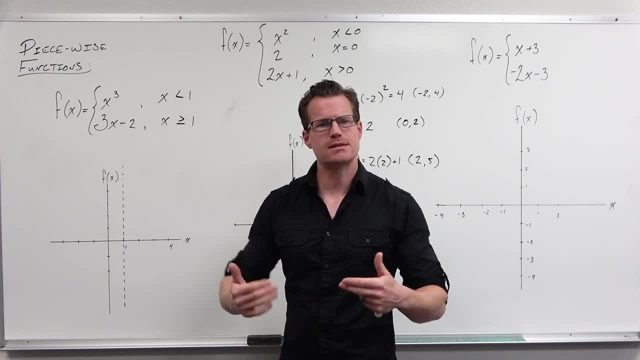 like a vertical asymptote idea. it's not a vertical asymptote and that's the same sort of a line that we use for vertical asymptote. so i understand that, but in the context of what we're doing we don't have a vertical asymptote here. um, that comes later we will talk about. i'll give you. 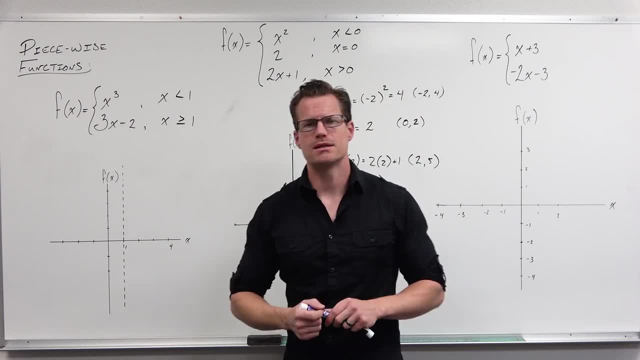 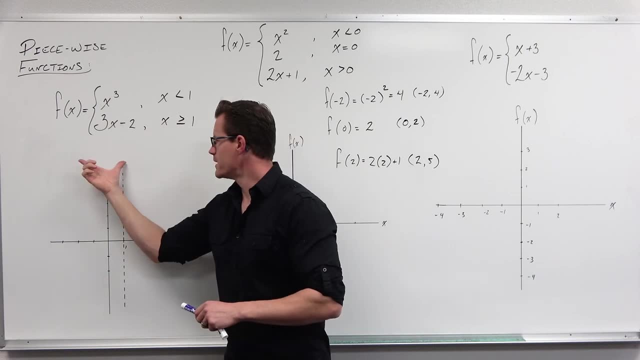 everything a vertical asymptote is and show you how to use them. but all this does practically it separates your x-axis and it says that your pieces of your graph will be defined on either this part to this part, but never both. You will never, ever have a piecewise function where you have two. 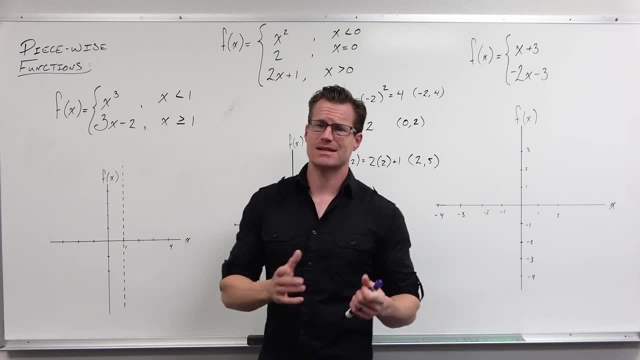 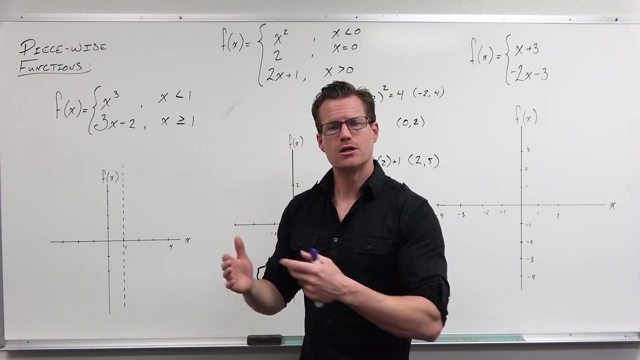 different graphs on the same interval of your x-axis. That's got to make sense. We know that domain says: for all of these inputs I'm getting one specific output. That's all that. that says You can't ever have an interval where you have two outputs. That means your graphs can't cross. 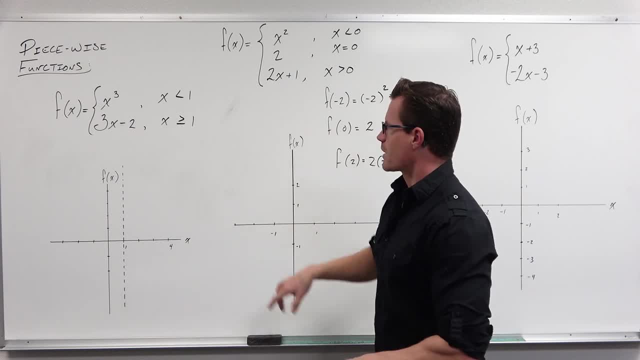 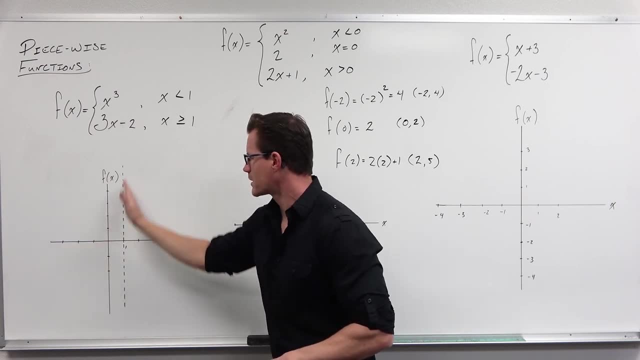 Your graphs can't overlap at all, So we're going to look at this All right, for x is less than 1,. x is less than 1 on this interval, not up to the y-axis, up to the dotted line, up to this. 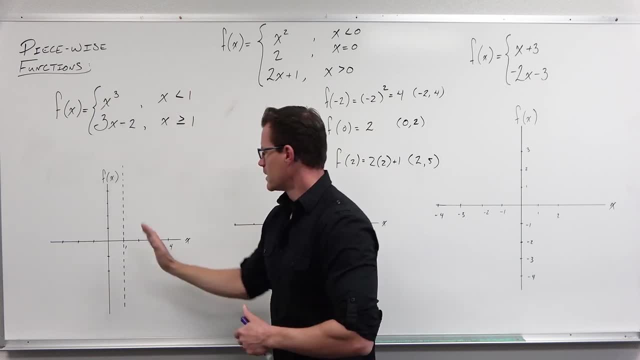 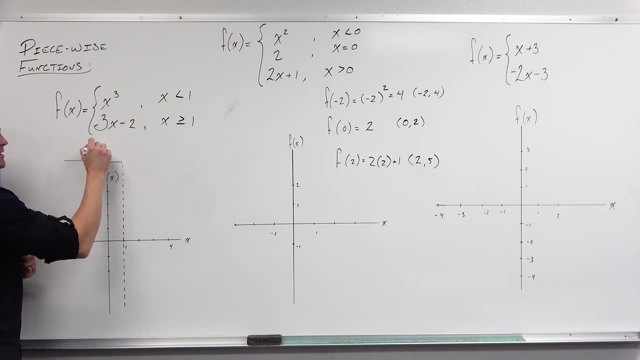 x equals 1, up to that boundary line I'm going to have x cubed. So I'm going to make a little mark over here that up to here I'm going to have x cubed. The graph of x cubed is only on. 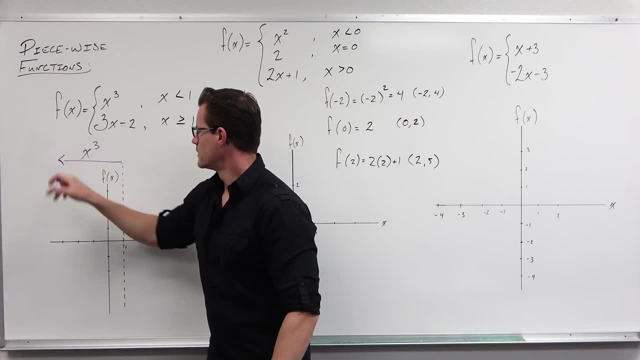 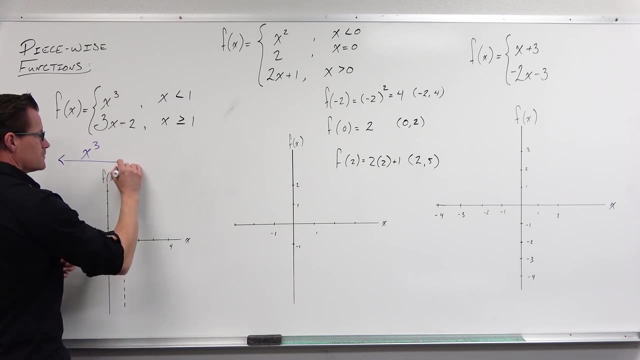 that interval of the x-axis all the way going to negative infinity On the right-hand side. so for x is greater than or equal to 1, so at this one we're going to have 3x minus 2.. So what? 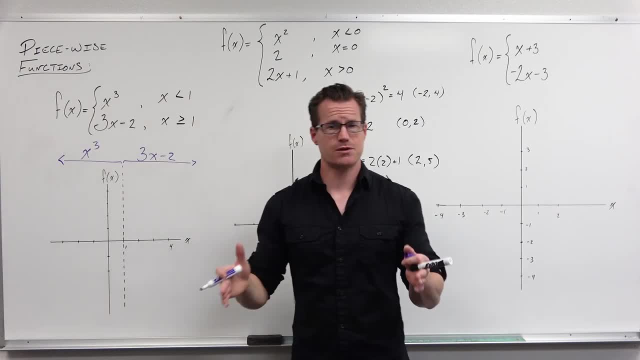 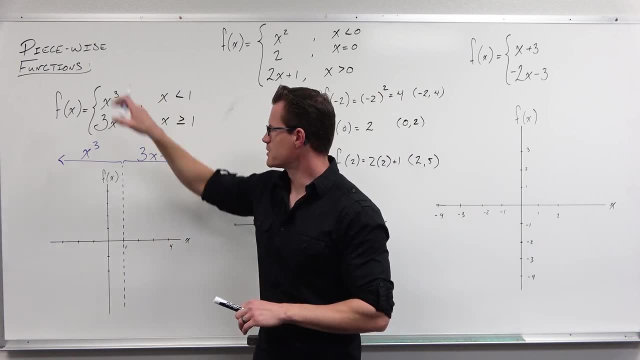 we're doing is we're taking our domain, we're separating our x-axis into intervals of that domain and we're understanding that these pieces will fall into one or the other interval. Just follow the directions. This says: for x is less than 1, use an x cubed For x is greater than. 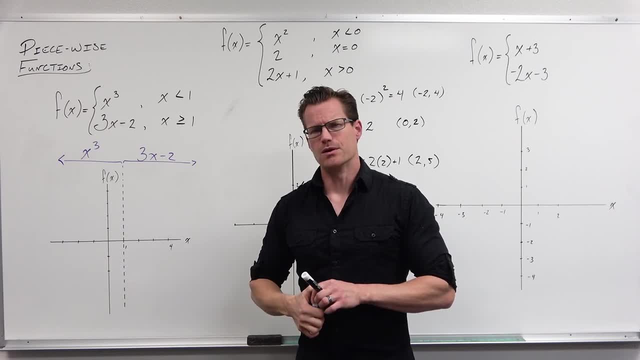 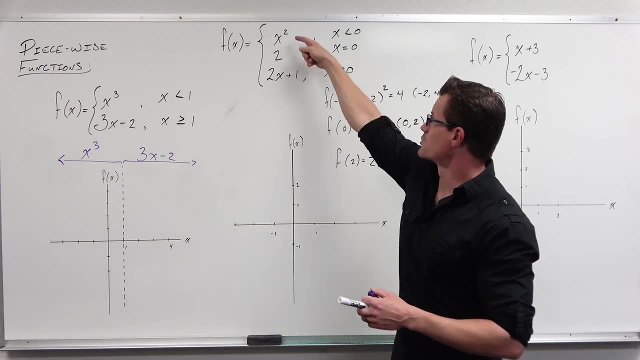 or equal to 1, use a 3x minus 2.. Now the next thing that we're going to do, we're going to review what in the world lines and cubics look like, What in the world quadratics and constants and lines look like- Same thing two lines over here. So when we're 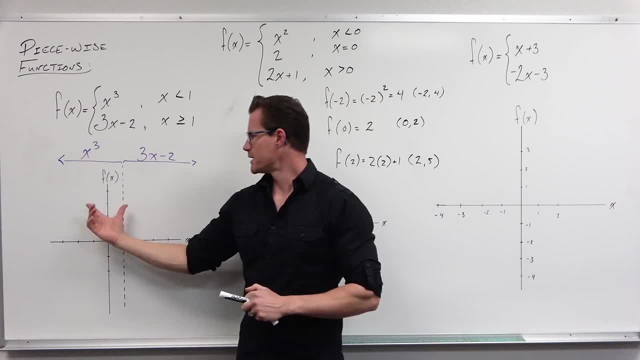 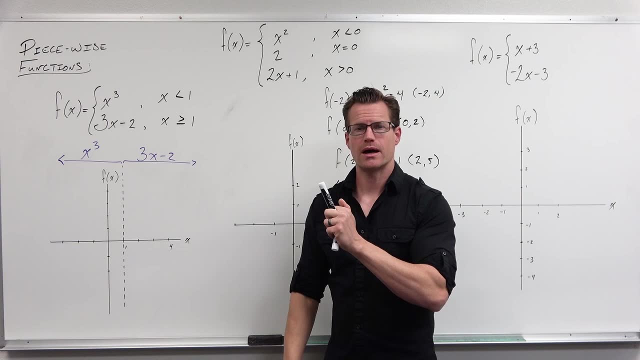 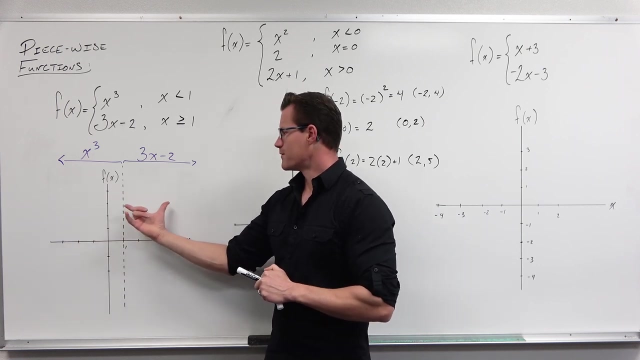 doing this, what I always do- I always graph the left interval first. Well, I always graph the side of- how about this? the side of my boundary line where my y-axis is. So my y-axis is on the left-hand side. I'm going to graph this interval first, then I'm going to graph this interval. So I'm 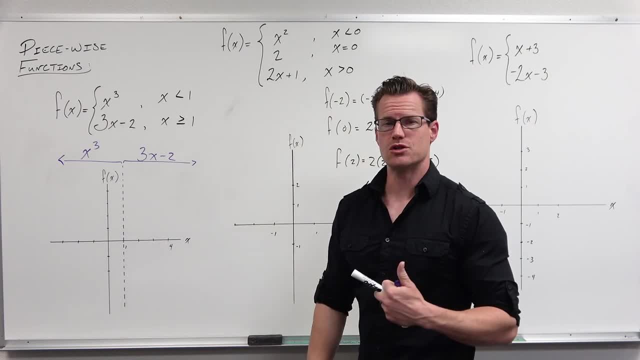 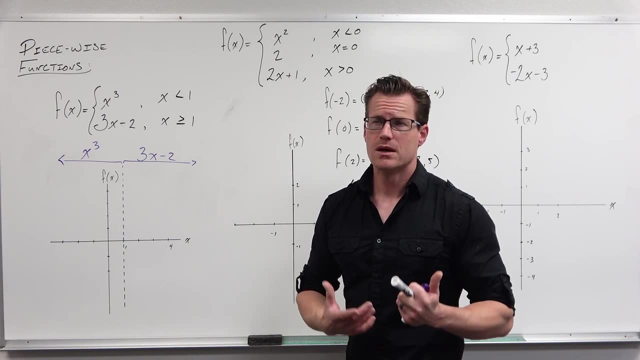 going to look at x cubed. What I'm going to do is I'm going to understand what x cubed looks like. I'm not plugging in points if I don't have to. There's only pretty much two values, One value. 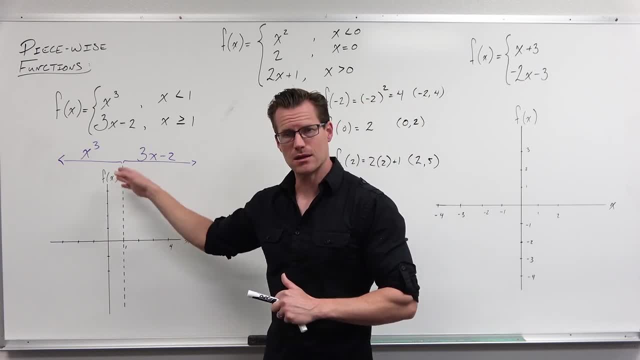 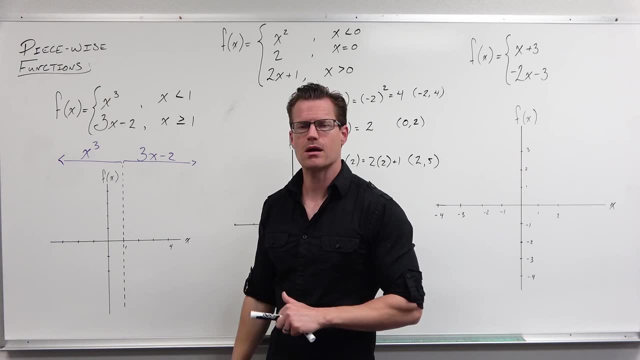 I'm going to plug in for two different functions. I'm going to plug in my boundary line number, so my 1.. I'm going to plug that in. I'm going to understand what less than and what greater than equal to actually mean there, And that's the only value, though I'm not plugging in a whole bunch. 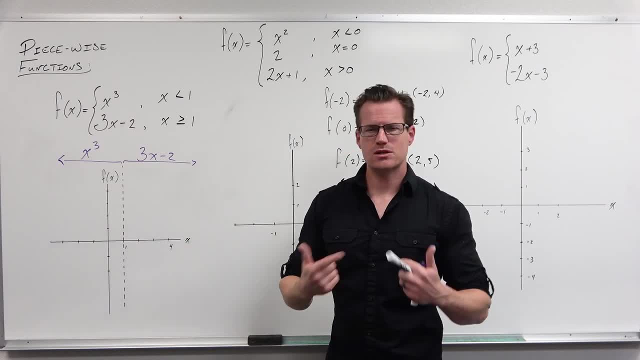 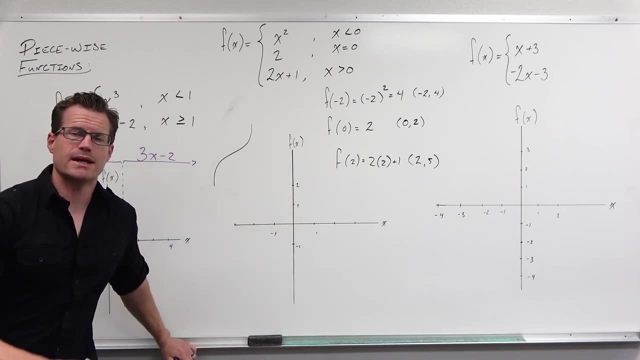 of points. I'm basically understanding what x cubed is, though x cubed is this s-curve graph. It looks like this. There's a few key points to it. Right now, I'm trying to teach two things. Number one is how to 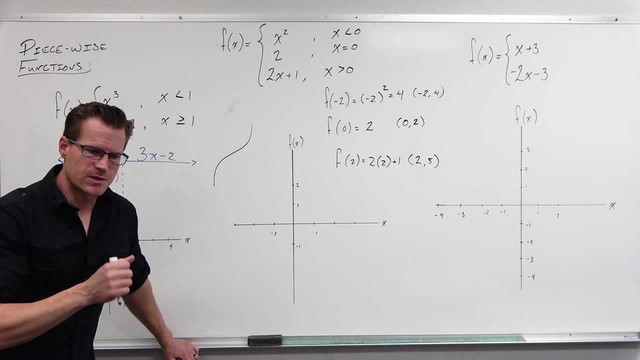 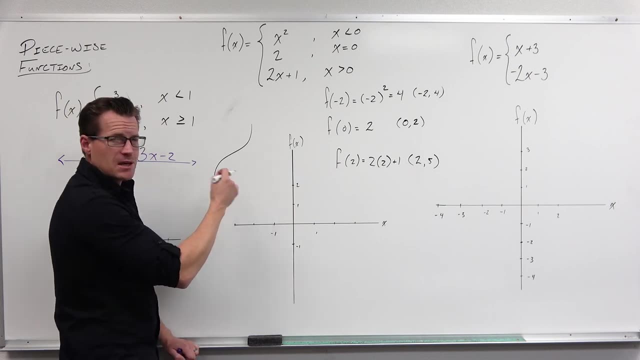 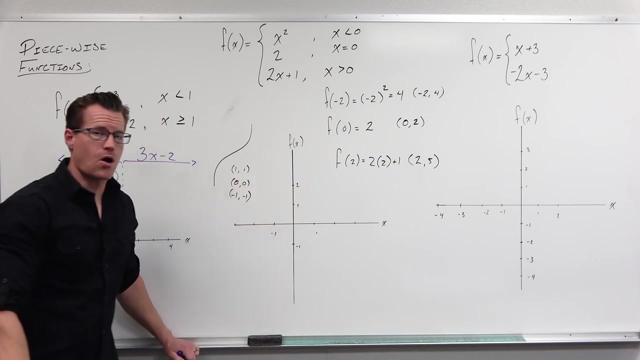 graph piecewise functions. but number two is that when you're graphing some of these basic shapes, it really helps to have an understanding of what x cubed looks like. The x cubed has three key points on it: 1, 1, 0, 0, and negative. 1, negative 1.. That stems from it being an odd. 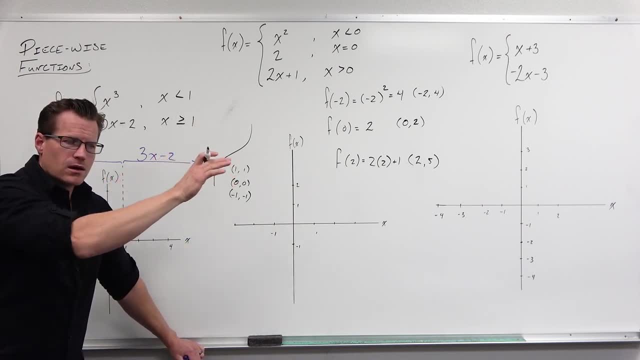 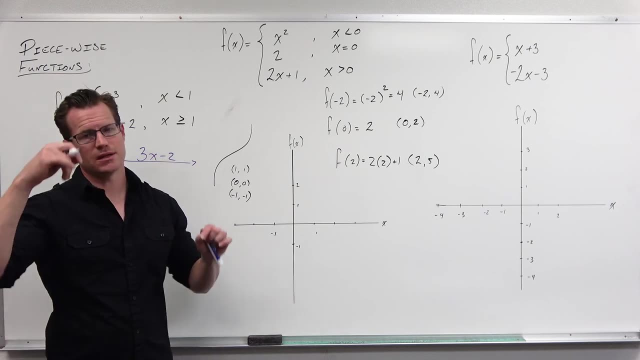 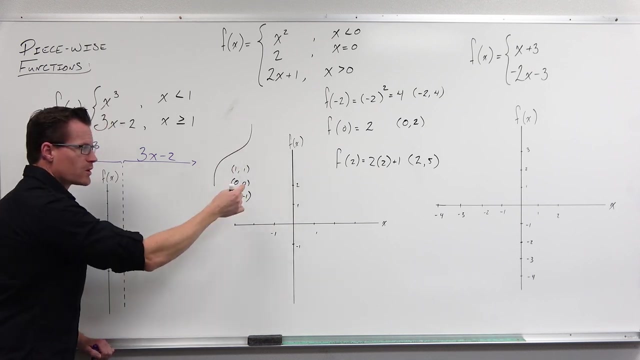 function. We talk about odd functions. This is kind of revolvable around or has symmetry about them. Negative 1, negative 1 have opposite inputs and therefore opposite outputs. So when we graph that and we say, all right, x cubed looks like this: It has some key points: 1, 1, 0, 0, negative. 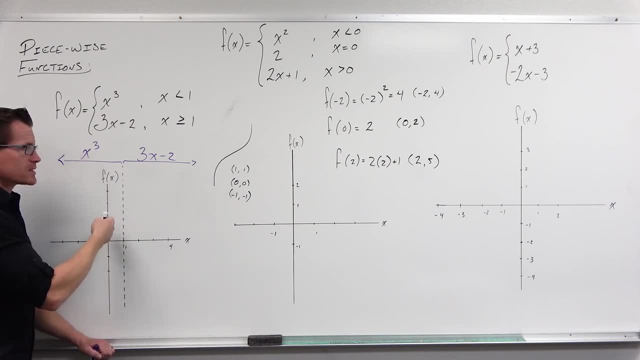 1, negative 1.. Yes, I can plug those in. I can plug in 0, 0.. I can plug in negative 1 and get out negative 1.. I can plug in 1.. Whoa, hang on. I can plug in 1 and I can get out positive 1.. 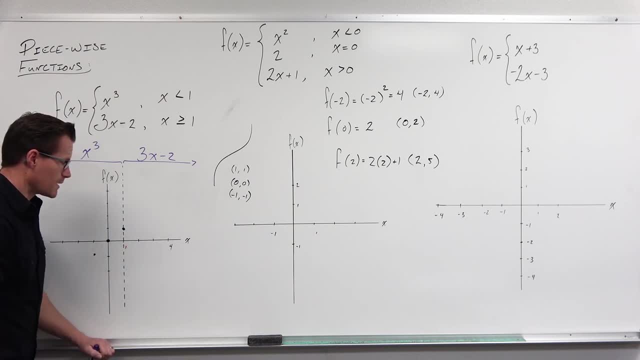 There's a mistake on the board right now, but I'm going to fix it in just a second. So this is the way my graph x cubed looks. X cubed is only defined for this interval of our x axis. It's an s curve. It's going to say, all right. well, I'm going to leave my origin. 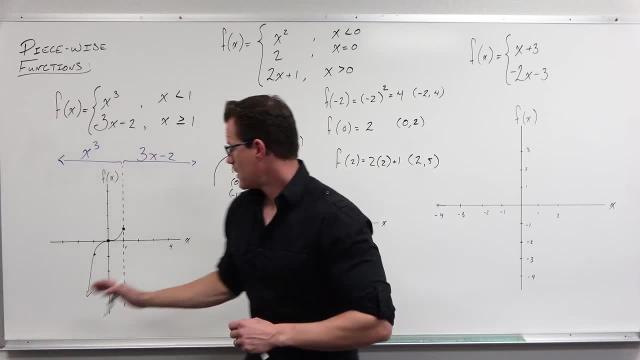 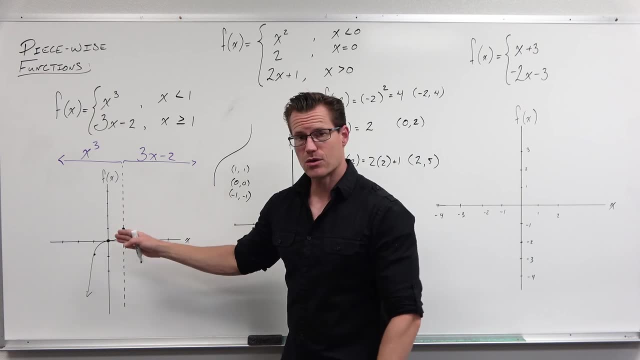 on my left-hand side of the y-axis. I'm going to drop to negative infinity eventually. I'm going to go all the way up to this point, but I cannot cross it. I can't let it go into the interval for which 3x minus 2 is defined. That would break the fact that this 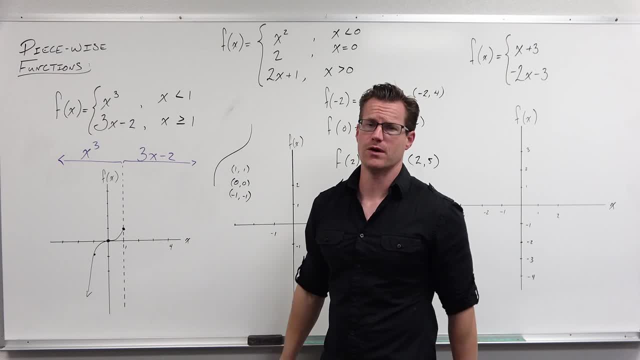 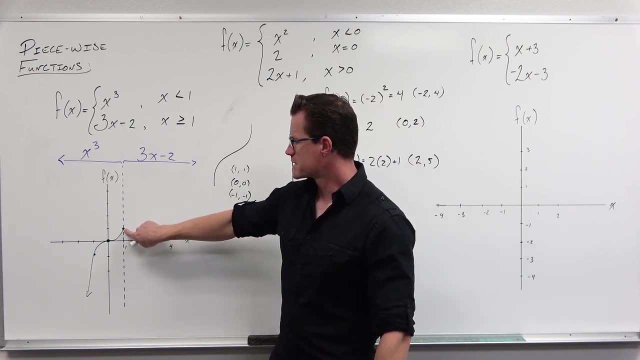 is a function. You can have only one piece of the graph on one interval of your function. Otherwise, you have two outputs for one input. That's a big problem. Now the next problem. What about that point? This is the mistake I was talking about. This is wrong. Why, Why is that wrong? 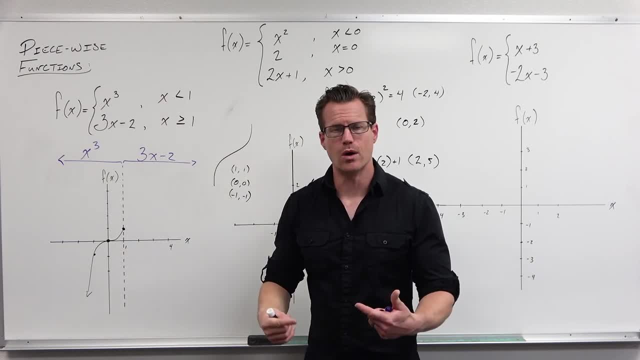 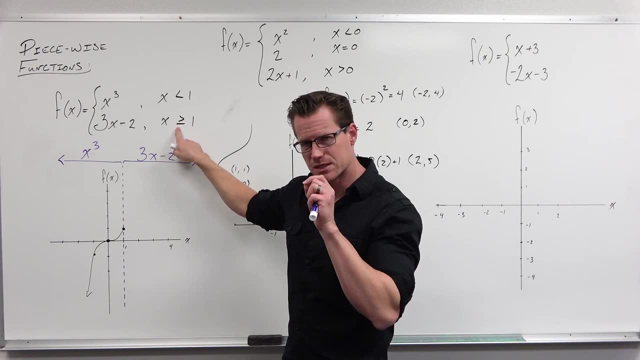 Because while this says you can go up to 1,, it says you can't include the 1.. So here's the deal: Whenever you don't have an equal sign, you must not include that specific point. Now please don't say: well, I can only go up to 0.. No, no, no, You can get all the way up into. 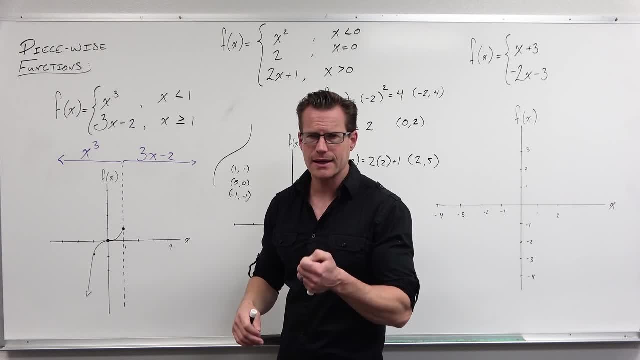 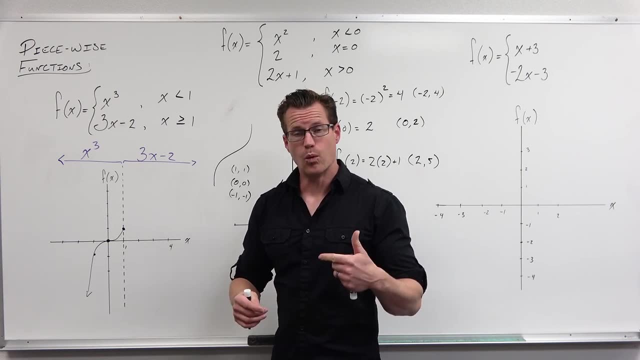 almost 1.. You can plug in 0.999999999999.. If you plug that in and cube it, you're going to get almost 1, but it's not quite there. For that reason, what we do if you do not. 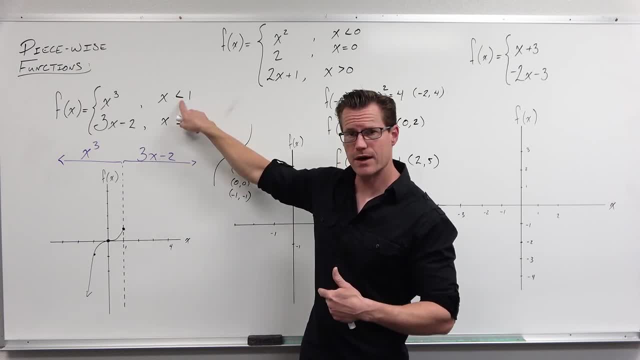 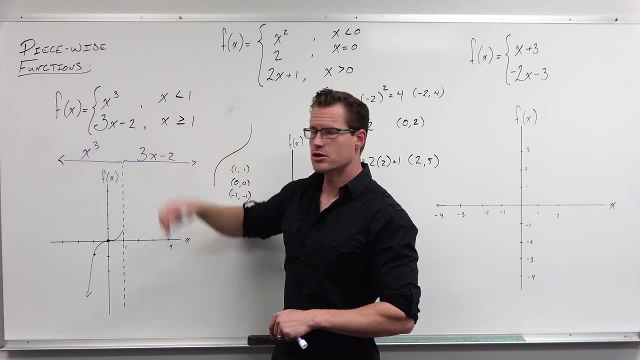 have the equal sign. do not include this value as an endpoint. How do we show that? You're just going to say all right. well, you know what I'm still going to plug in: 1.. 1 cubed is 1.. That gives us almost the point 1, 1,, but we're going to show this as an open circle. 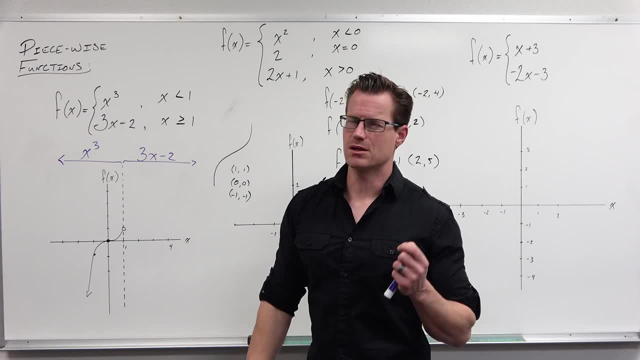 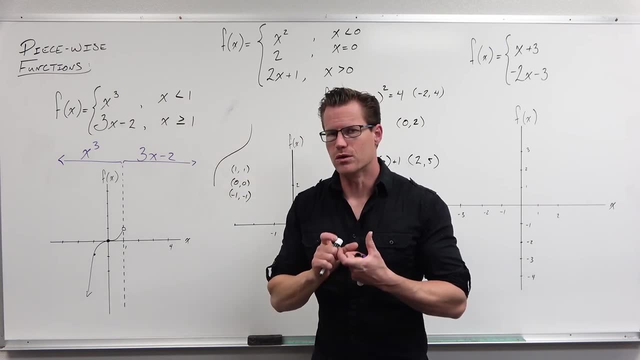 Saying that just that specific point is missing. you need to remember this from some of our previous videos that we just did that when I don't have the equal sign, I just don't include the point. How we don't include the point is with an open circle like the parentheses idea. It says: 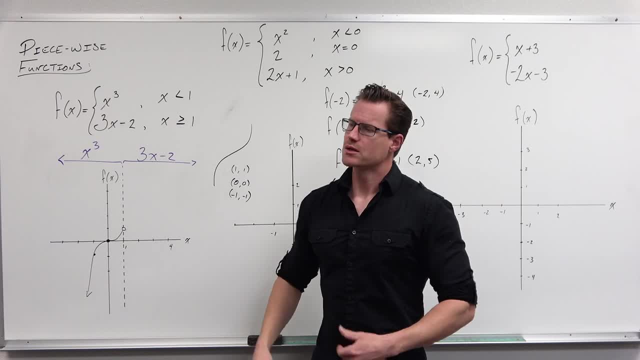 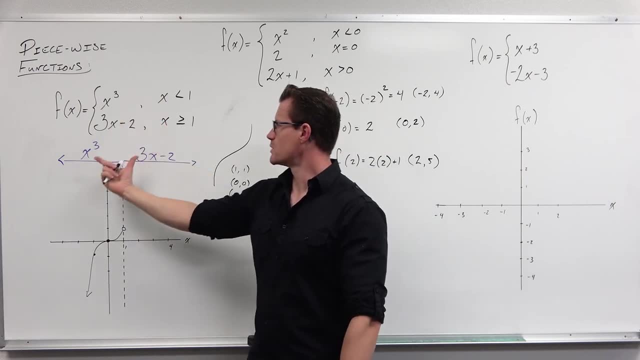 all the way up to it just doesn't include that point. It's missing one point. So a long story made really short, hopefully, is find your domain, separate your x-axis, identify what piece goes in what interval and graph the piece If you don't have an equal sign. 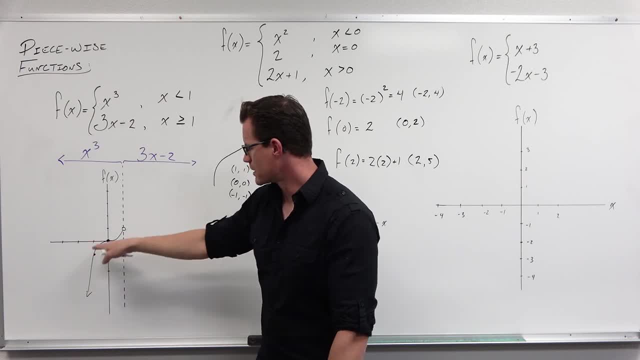 use an open circle for the endpoint. So here I said: okay, x cubed, I understand what that looks like. I understand my three key points: negative 1, negative 1, 0, 0, 1, 1.. So I put that: 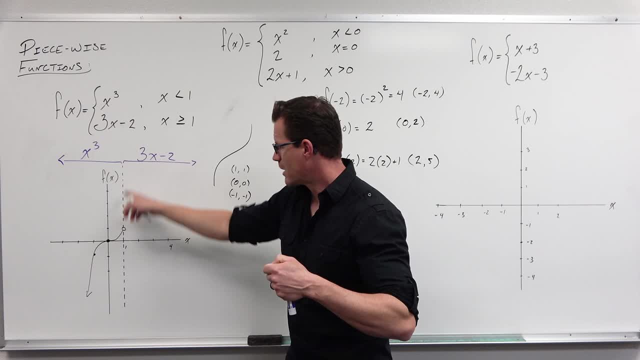 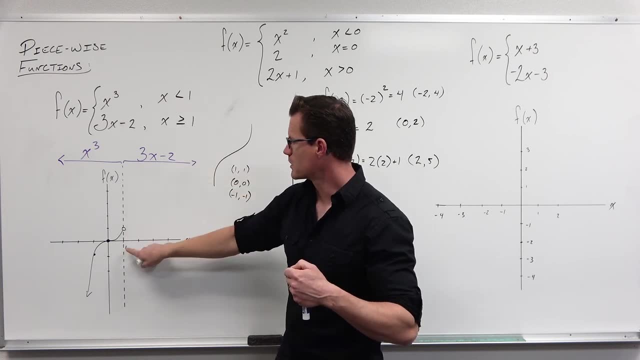 on my graph and then say, all right, I'm going to look at my boundary line. I'm going to look at that value on my x-axis and say, okay, 1 should not be included. So this point is an open circle. 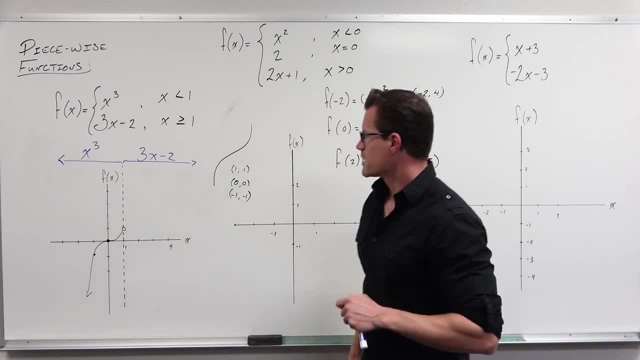 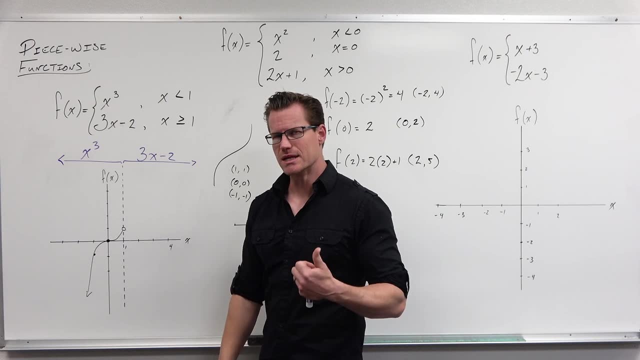 That needs to make sense before we go any further. Next I'm going to look at 3x minus 2.. Now I'm going to look at the y-axis side of my boundary line. It's because it's a little bit. 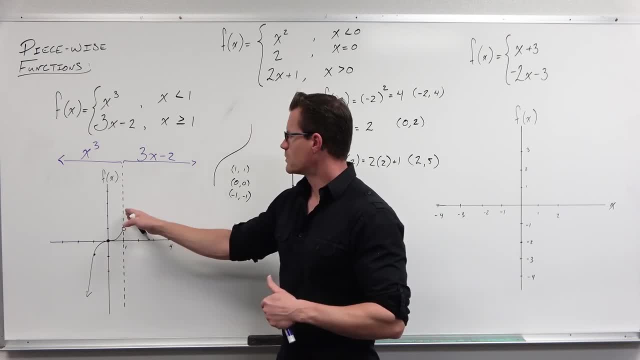 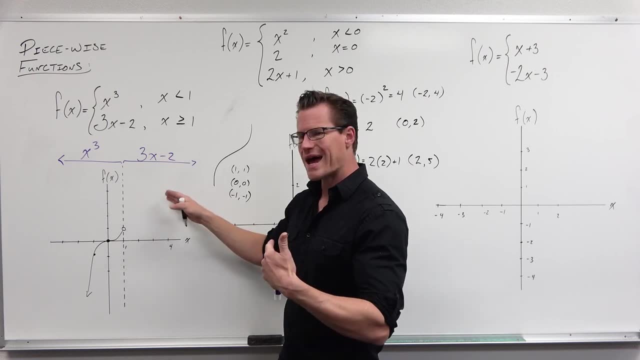 easier for me. I have a y-intercept. that's very easy to find. I don't have that on the right-hand side And frankly, it doesn't matter which you graph first. On the right-hand side, I think it's a little more difficult because there's no y-axis, There's no y-intercept over there. So here's what. 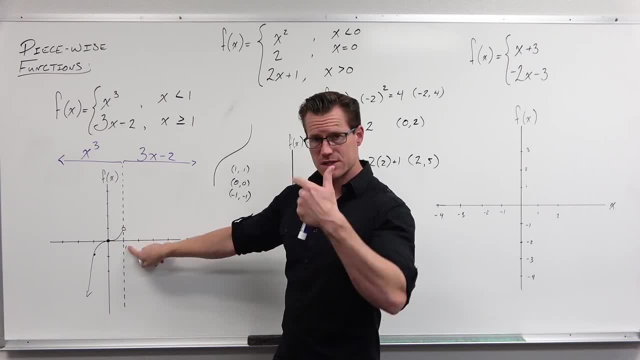 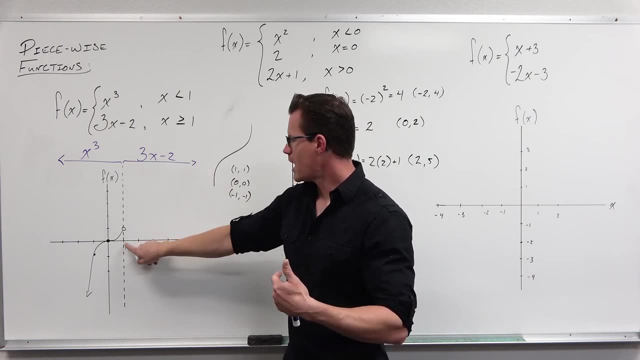 we do? What we do is we take our boundary number, our separating number, that 1, and we plug it in. So we say, all right, well, since this piece is defined for this interval, I'm going to plug in. 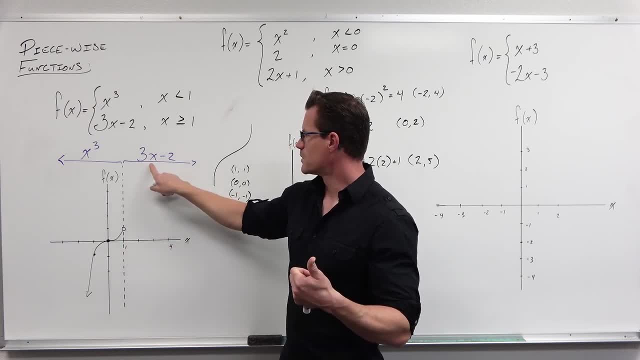 where I start. I'm going to go all right, I'm going to plug in where I start. I'm going to go plug in 1.. 3 times 1 is 3.. Minus 2 is 1.. 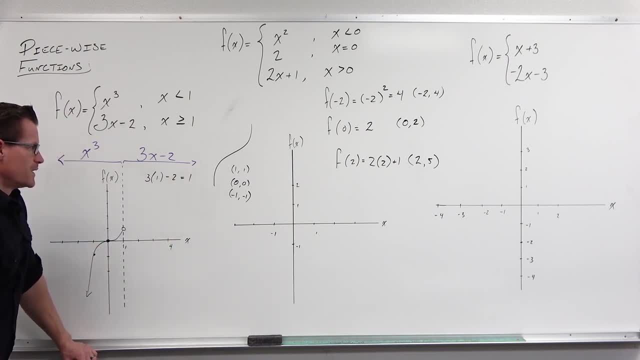 So if I find f of 1, that says all right, this is giving me out the point 1,1.. Hold that, Wait a minute. That's interesting. That's this value right there. So wait a second. This cubic was. 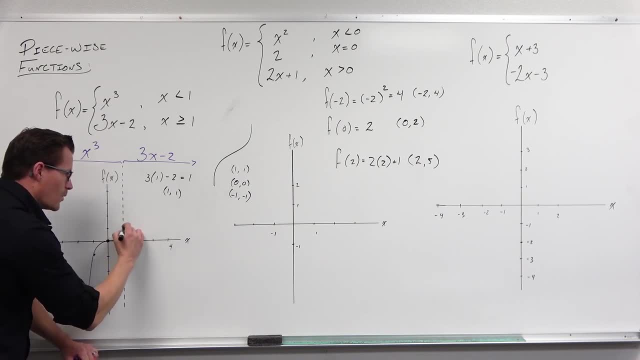 missing that point. It's missing that point. It's missing that point. It's missing that point. This value, this graph, has that point. So we're going to graph this in just a second. We're going to graph it, And what we're going to do is we're going to say, all right, the black line, right. 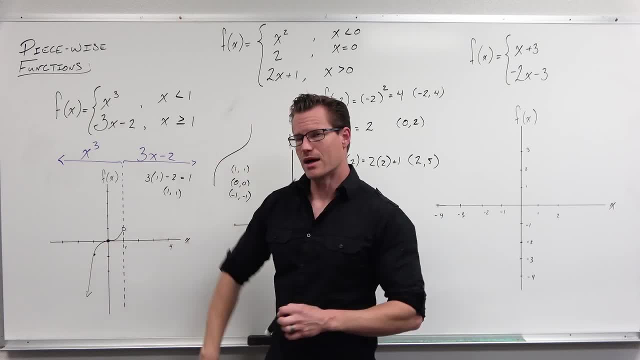 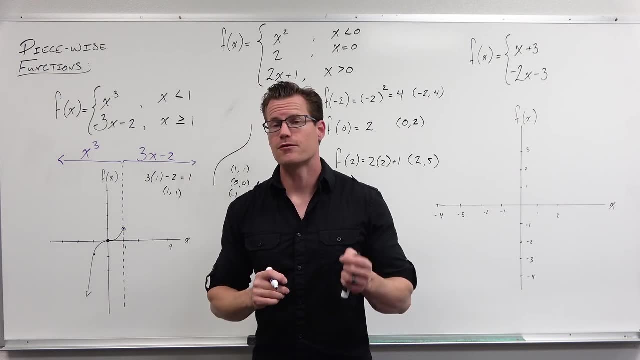 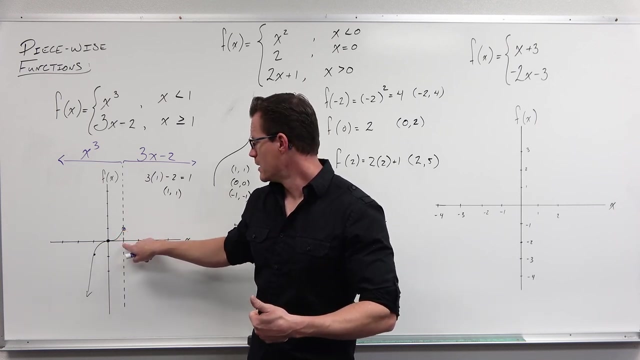 here. I hope you can see the colors. The black line is x cubed. The purple line I'm about to graph, says this point starts right there. It starts there. Notice how this does not fail to be a function in that there's not two points for that one input value of 1.. This value of 1 is not. 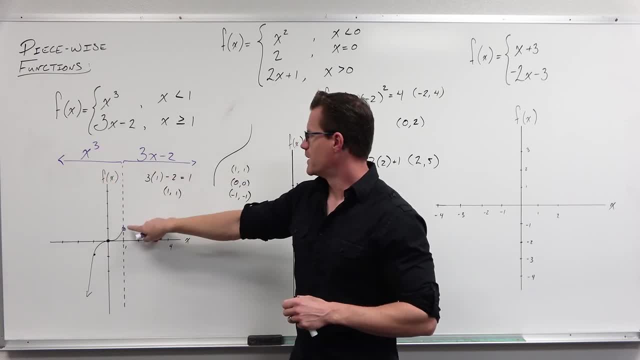 defined for x cubed. There's only one input value of 1.. There's only one input value of 1.. There's a hole. This value is defined for 3x minus 2.. It fills in the hole. It's not breaking the fact. 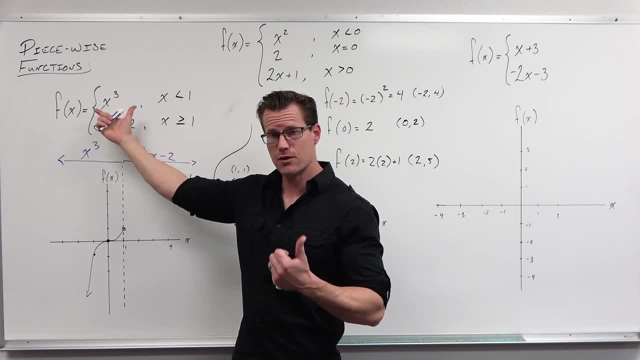 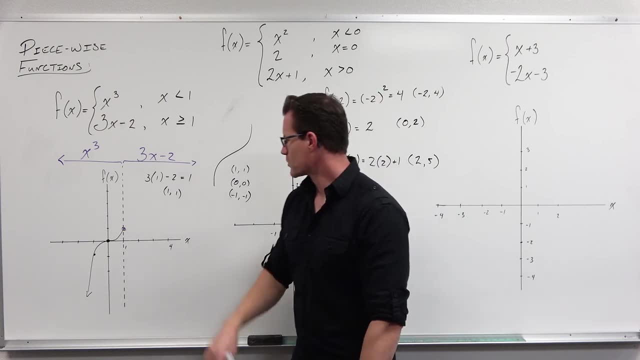 it's a function, because x cubed does not have an output for that input value of 1.. This does have an output for the input value of 1, which so happens that it fits in that hole. That's pretty neat. Kind of a cool little graph that we did. Kind of made it up in my head but worked pretty. 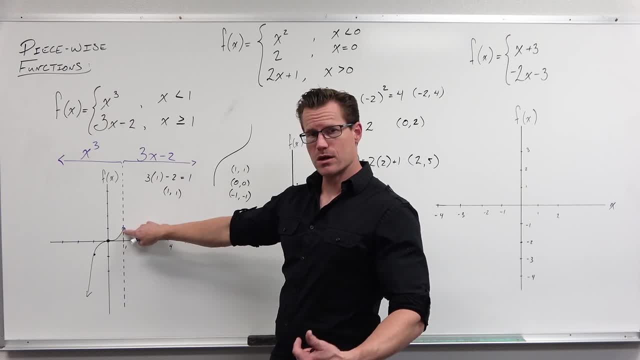 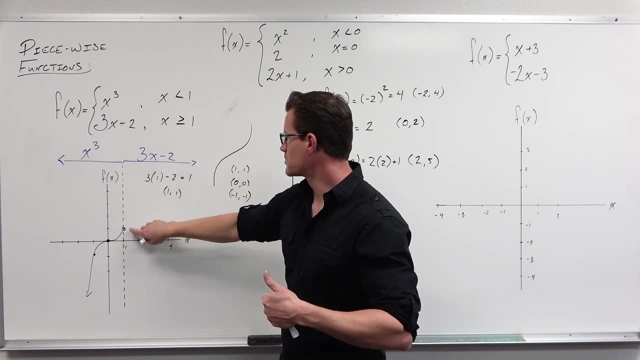 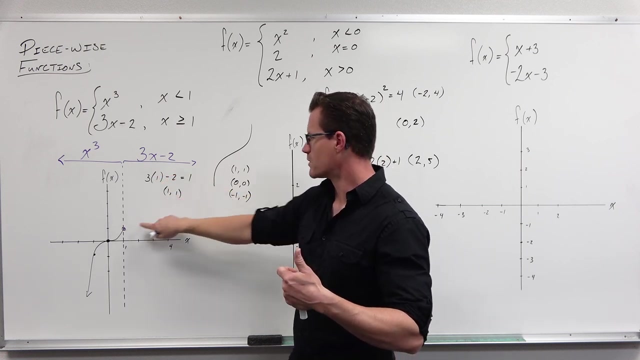 well, Now for the rest of it. since we have now a starting point, we know that our output value is actually on that step, that boundary line. So this is defined for x cubed. So we're going to plug in 1.. I did 3 times, 1 is 3.. 3 minus 2 is 1.. Okay, here's the plugged in 1, got out 1, right. 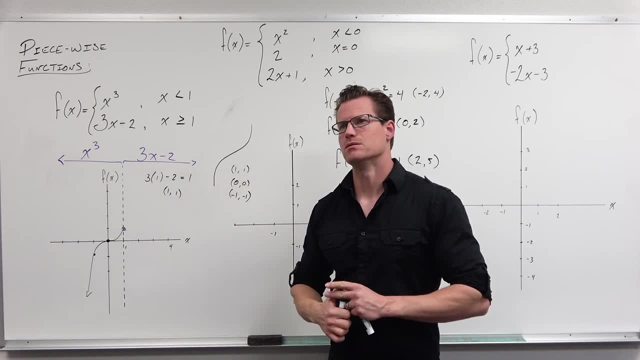 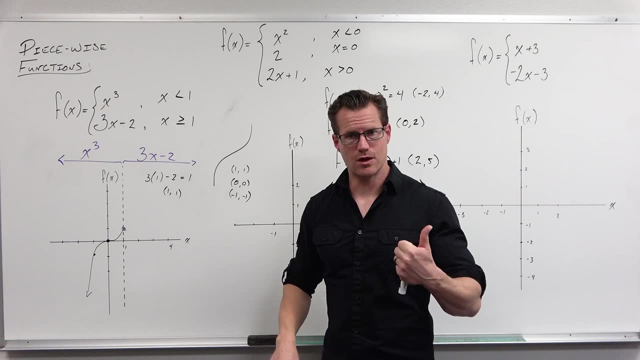 there. Now what is that? What is 3x minus 2?? Well, it's not a cubic, It's a line. Lines have a starting point. We've got it. They also have a slope like 3 over 1.. So it says from that point: 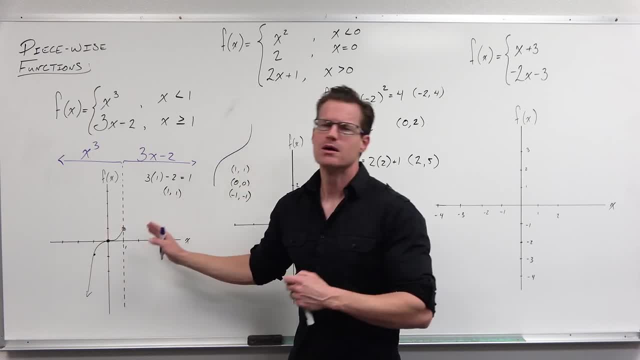 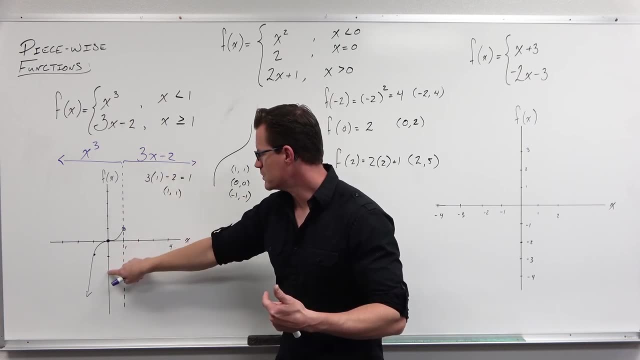 from that one starting spot on your boundary line, not before it. don't go to the y-axis, Don't go to a y-intercept of negative 2.. Why, If you went to a y-intercept of negative 2, and started graphing this, you're going to have a whole bunch of points right here for which you 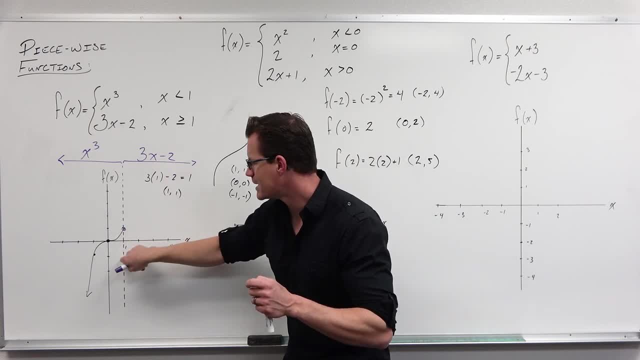 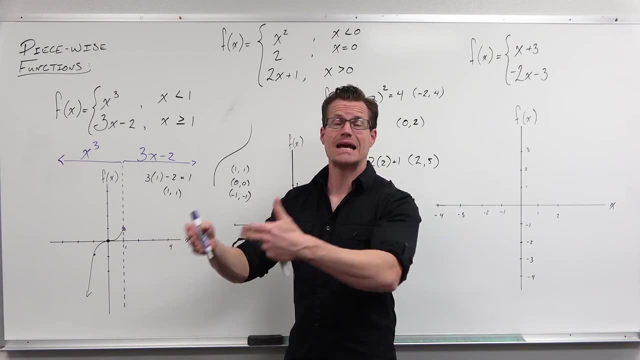 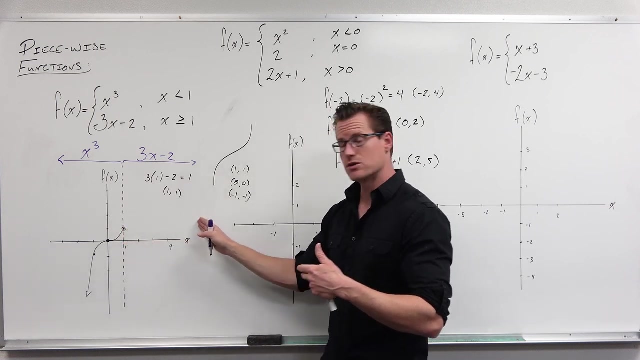 are breaking the rules of your domain. This is not defined on this side. You can't go to the left of that boundary. That's why I choose to graph the y-axis side first, Then go all right. I cannot cross that, I can't touch that. This is the boundary. This is the only place where my functions. 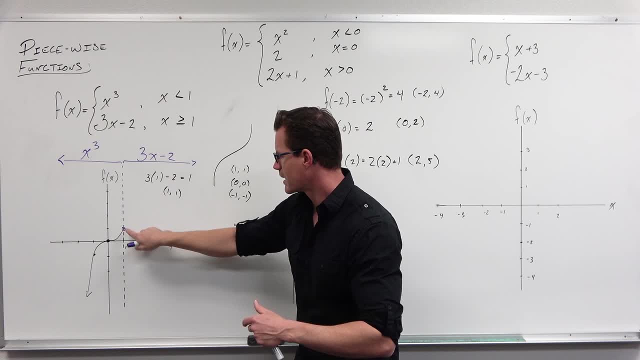 are defined. I've done that. I've plugged in the boundary number. I plugged in 1.. I got out 1.. Now I'm going to use the fact that this has a slope of 3 to go from that boundary and say: all right, how slopes work, is we go? 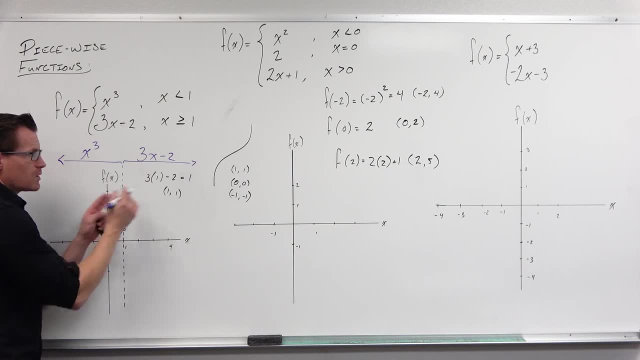 up 3, 1,, 2,, 3.. We go to the right one because the slope is 3 over 1.. And this gives us a line. So we're going to graph that piece of the function on this interval of the x-axis for which we're going to define the domain. 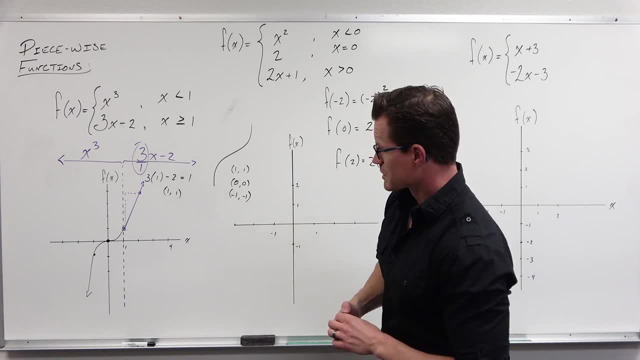 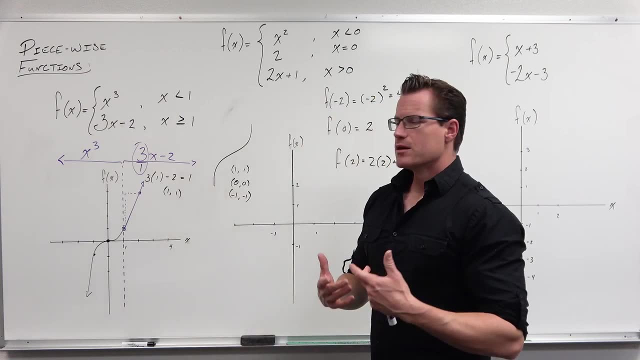 That's the way that this graph. it almost looks like a cubic, but it's not. This is a straight line. A cubic would have gone very steeply through here. This is the way that piecewise functions are graphed. What you do is you look at your domain, You separate your domain into 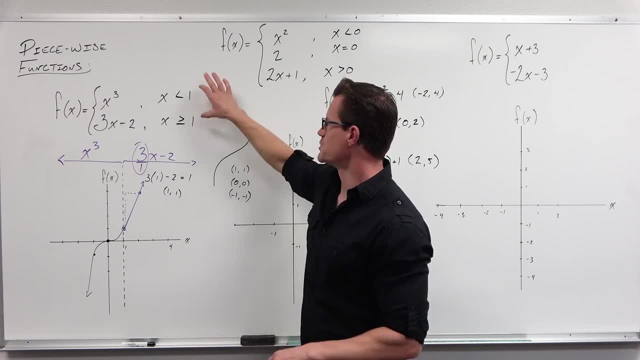 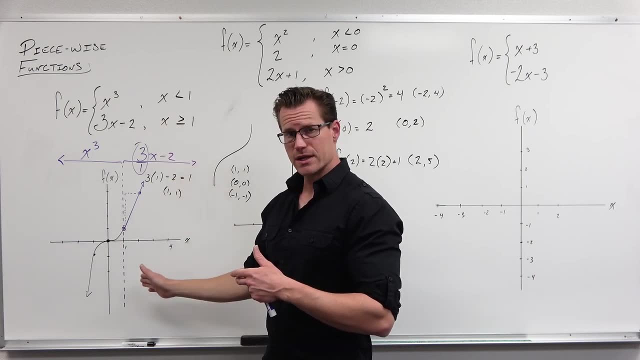 an interval. I call it a boundary number or a separating number, No problem. This tells you what intervals of the x-axis for which these pieces are defined. Don't break the rule. Just make sure that we're understanding where that separator is. We're understanding where our 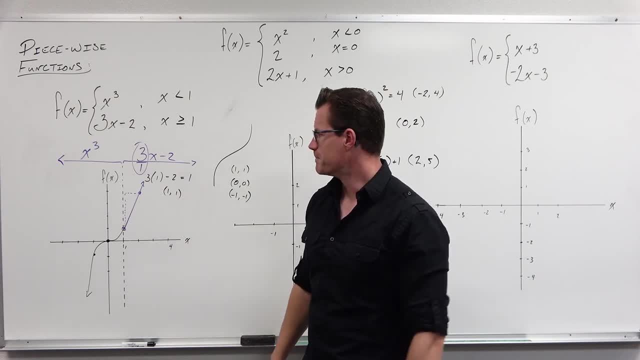 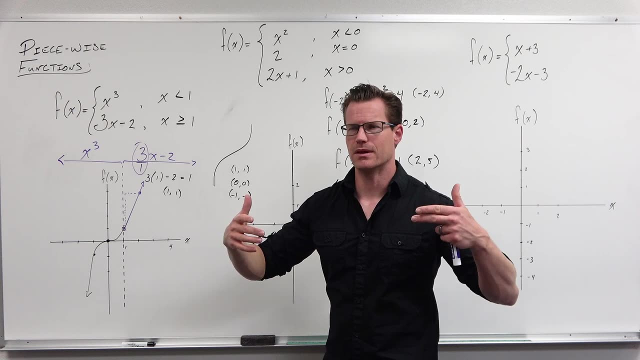 pieces work on the intervals for which we just defined. So that's the way that you're going to have a defined domain. Let me graph: this for one interval, this for another interval. You can do it by plugging in points. But again, my secondary motive for teaching you this is to understand what 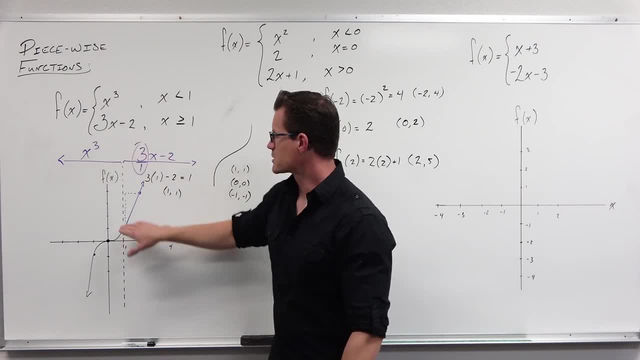 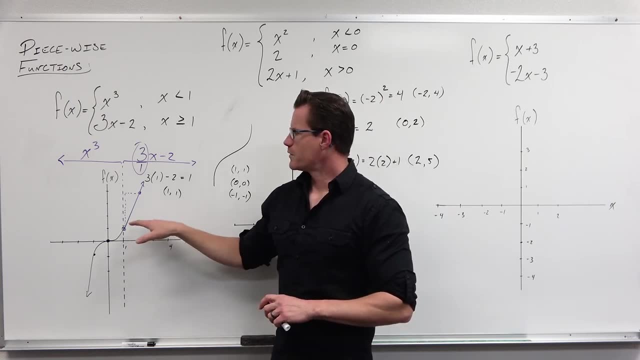 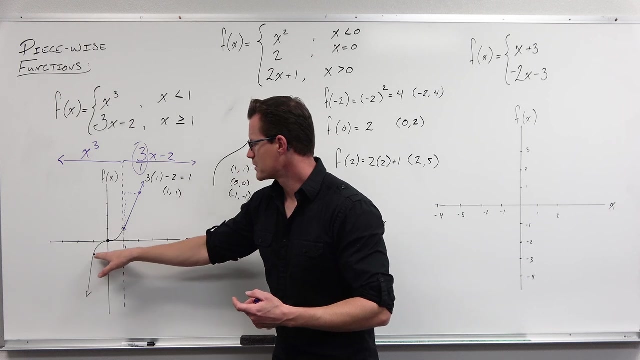 cubics look like, to understand what lines are with slopes and to understand these things do not cross over. The last thing I want to mention here is that not all of your piecewise functions look like this. This is kind of a special case where one interval we had this cubic that left. 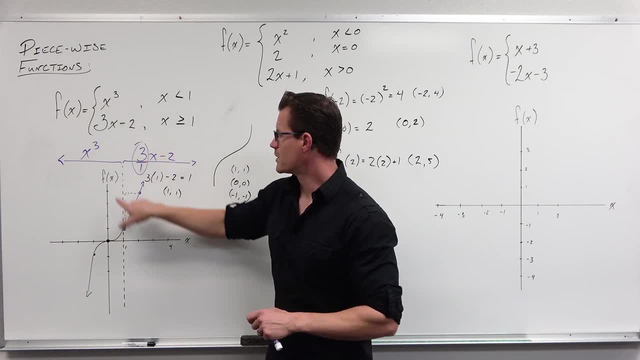 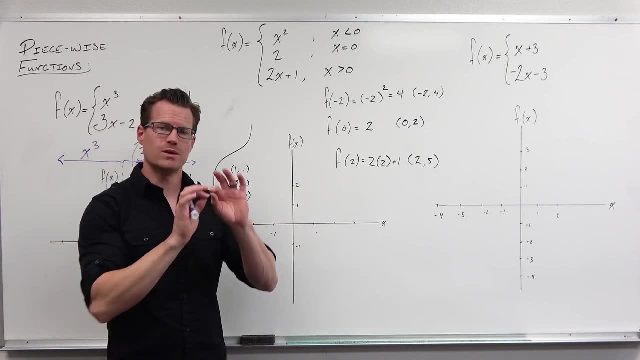 an open Circle, an open point, a missing value- This one filled it in. That's kind of a cool little graph. That's not going to happen on this. We're going to notice how, with piecewise functions, often we get these jumps where we don't have a continuous function. So I'm going to talk about 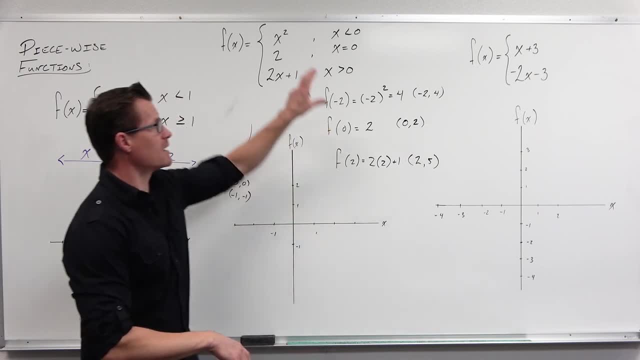 continuity here real fast and then we'll move on. So we're not going to have a continuous function. We have this- I'm sorry I'll talk about after we do this and then we'll move on. So we're not. 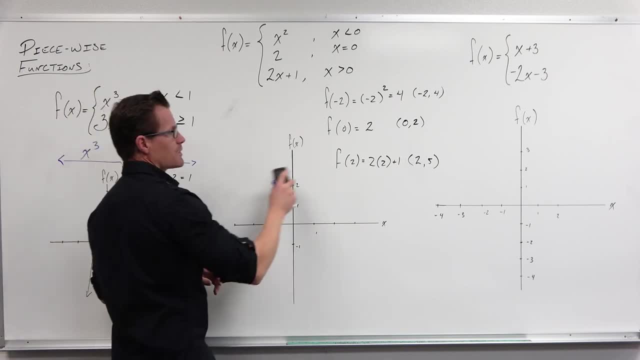 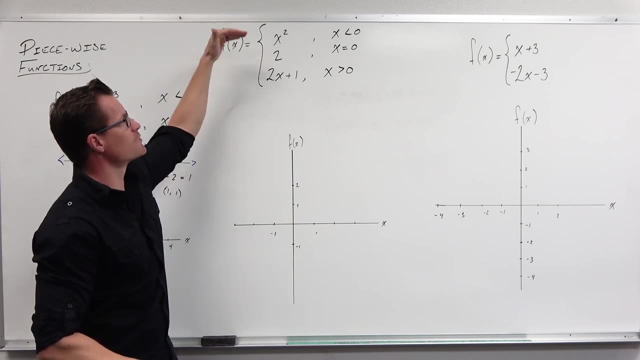 going to have a continuous function. We're going to have a little gap here, So I'm going to show you how to deal with that. So, starting out, we look at our function. We go: all right, here's a piecewise function. We. 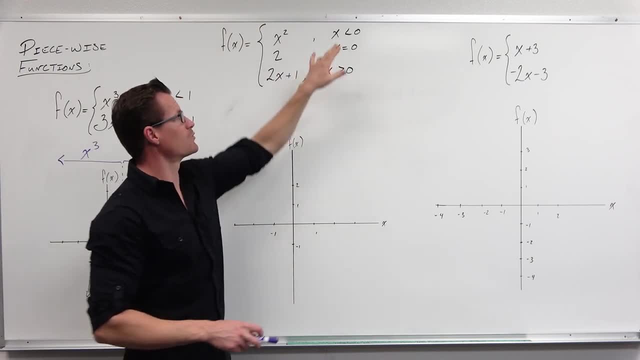 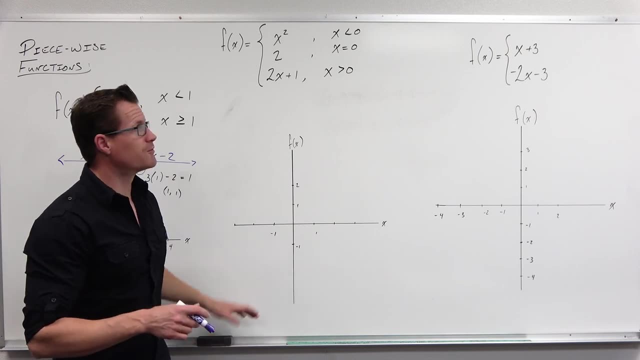 basically have three pieces and three different domains. It says for what interval in the x-axis these particular pieces are defined. So I'm going to go to my separating value of: well, what's separating these? What's the kind of boundary for when we use these particular pieces? 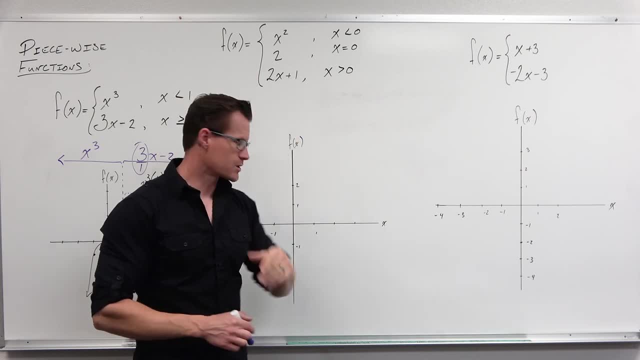 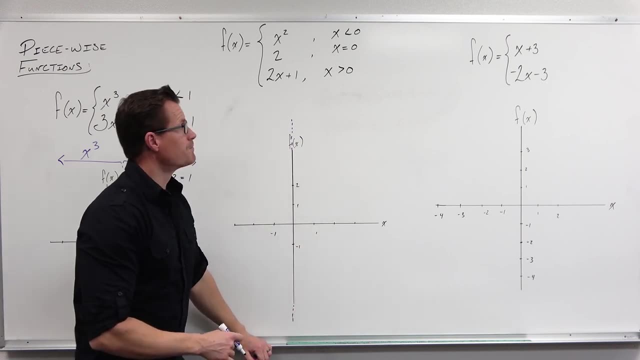 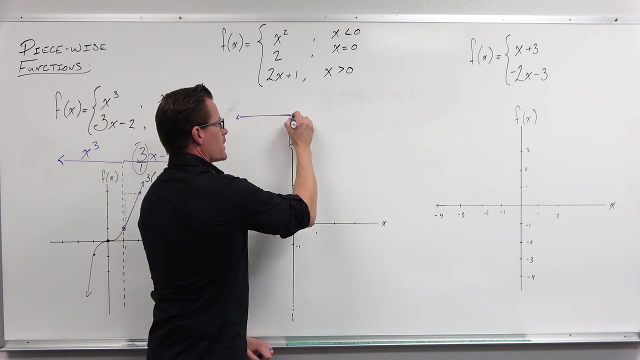 That's zero. Well, x equals zero. That's the y-axis. So we're going to go to the y-axis and say, all right at, x equals zero. That is my boundary To the left. I'm going to be using a certain function To the right. 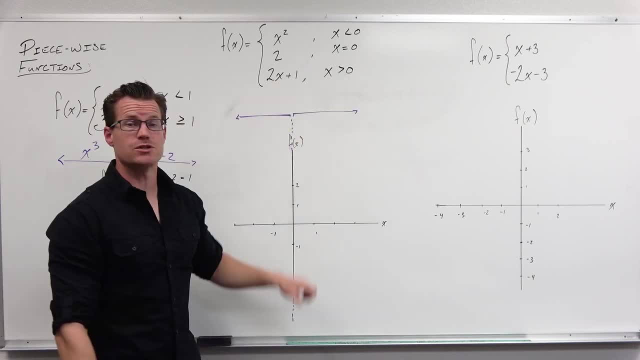 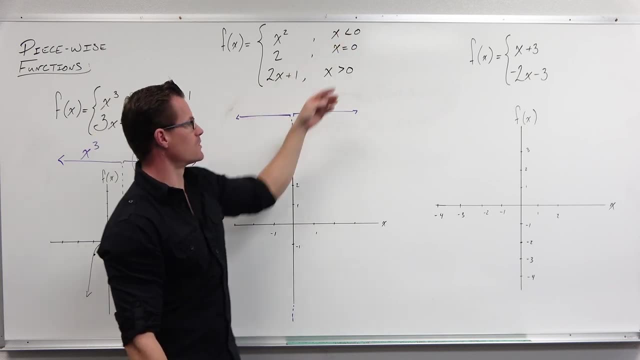 I'm going to be using a certain function At it. I'm going to be using a certain function. So, to the left of zero, this is saying: for greater than zero, use this piece For equal to zero, use this piece For less than zero. So, on our x-axis, our domain always separates our x-axis. 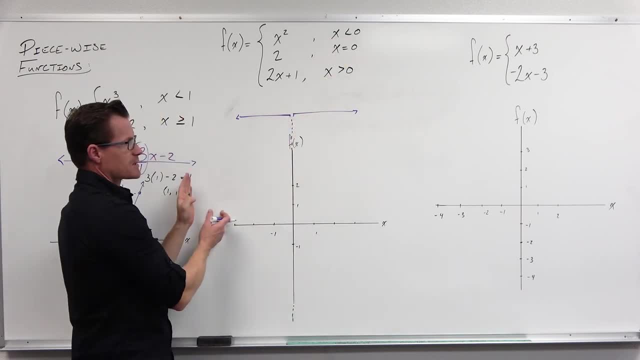 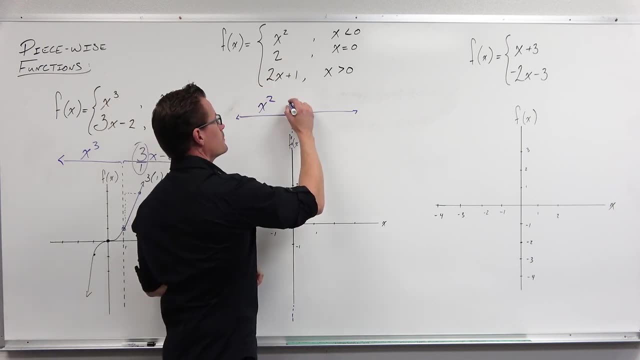 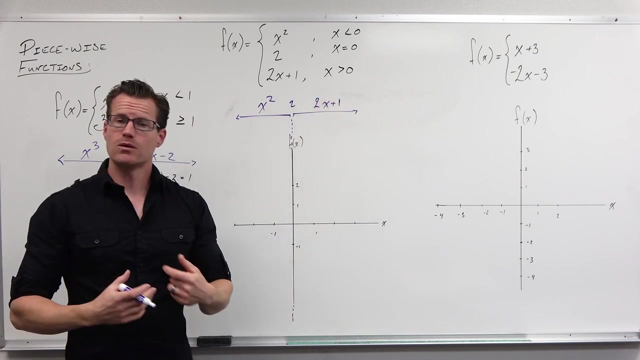 into little intervals. It says: for anything less than zero to this side, I'm going to use x squared. For anything at zero, I'm going to use 2.. For anything greater than zero, I'm going to use 2x plus 1.. That's exactly what the domain for piecewise. 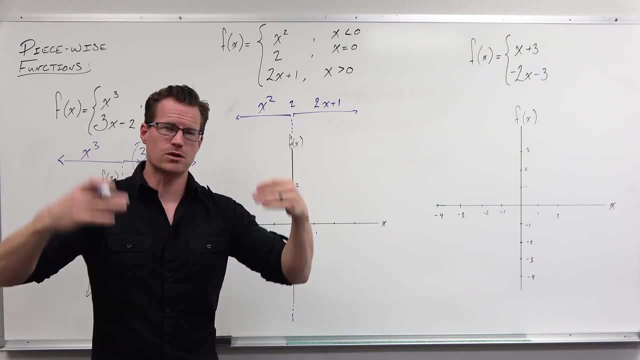 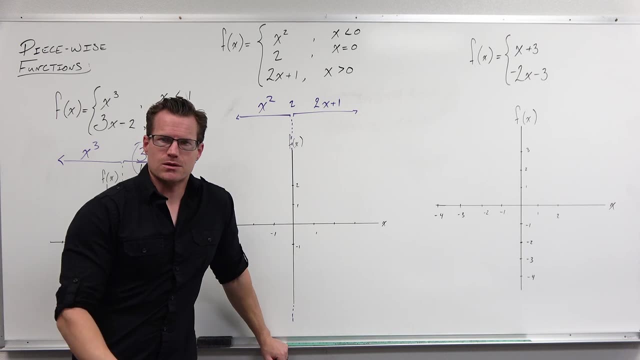 function does Separate your x-axis into little intervals on which you're going to graph specific pieces of your function. So let's do it. You know what? probably the easiest one to do right now is at the x equals zero. So at x equals zero, it says hey on x equals zero. on that line. 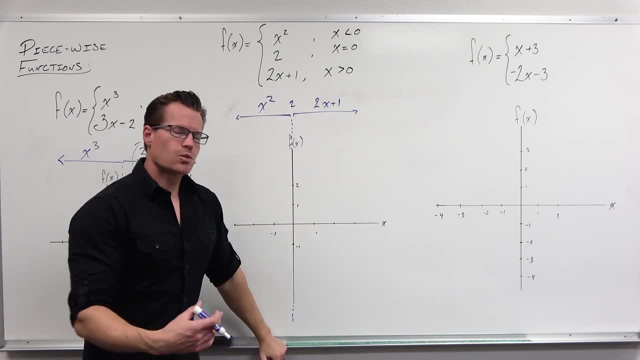 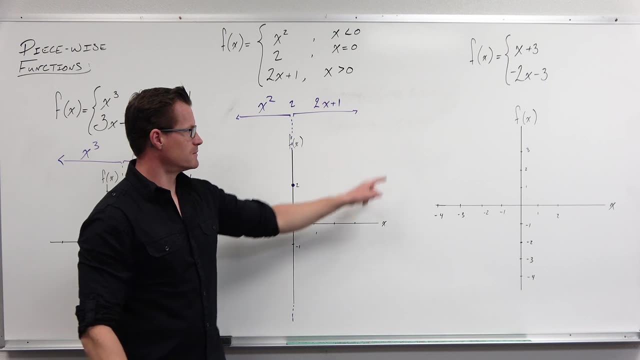 on the y-axis, you're just going to have output value of 2.. So we're going to go to 2.. All right, output value of 2.. Done, That is the point, If you remember. I erased it, but it said it's right there. It says: when you plug in 0,, you get. 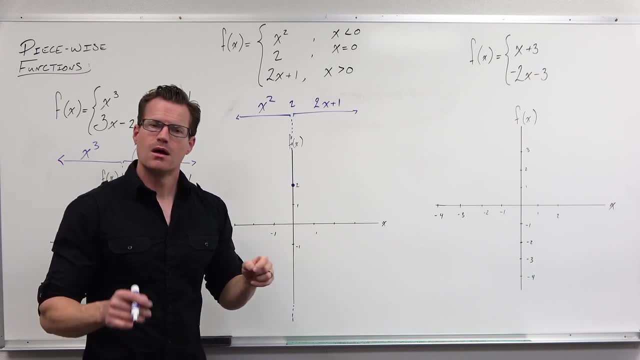 out 2.. Hey, we plugged in 0, we got out 2.. That's all that means. The only point on the y-axis needs to be an output of 2.. Plugged in 0, you get out 2.. What that means is that for this function and 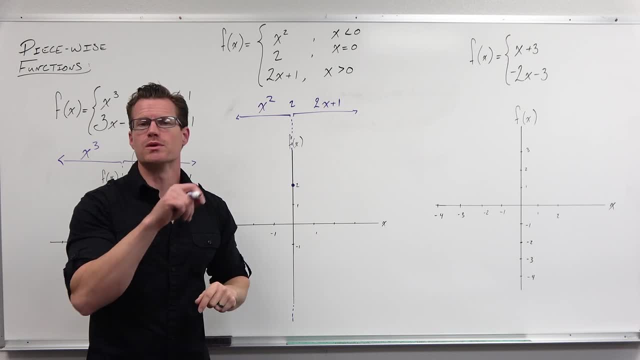 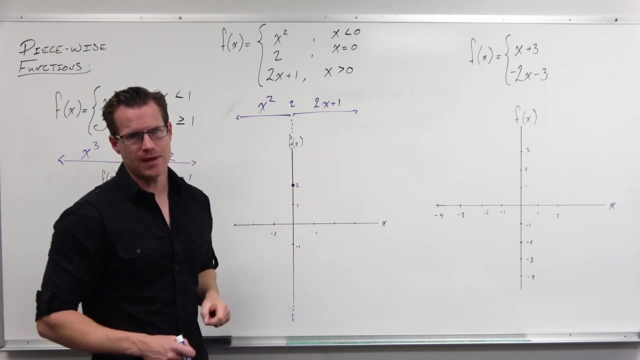 this function. when I get to my boundary line, I'm going to use an open circle signifying that I don't have an output there. The output for 0 is 2, but it's going to go right up to that output. 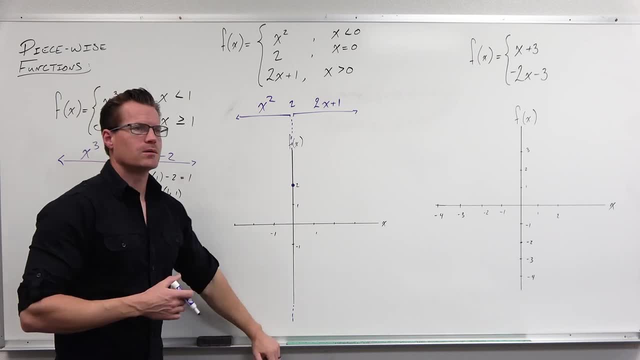 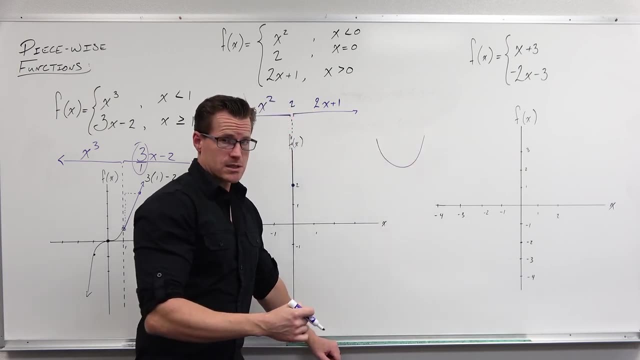 value that we're missing. So x squared. Do you remember what x squared looks like? Do you remember that it's a parabola? Parabolas look like this and they have some key points. They do have 0,, 0,. 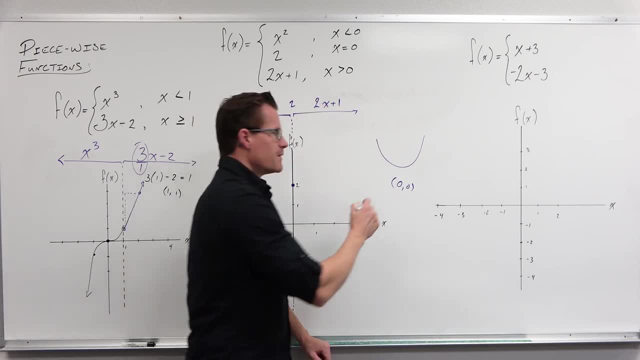 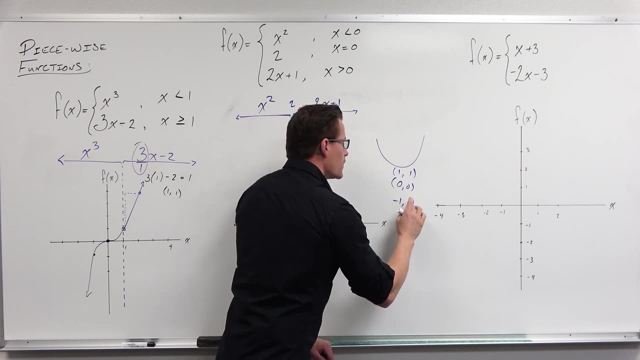 but because if I plug in 0, 0, squared 0, they have 1, 1.. If I plug in 1, 1, squared is 1. They have negative 1, positive 1.. If I plug in negative 1, 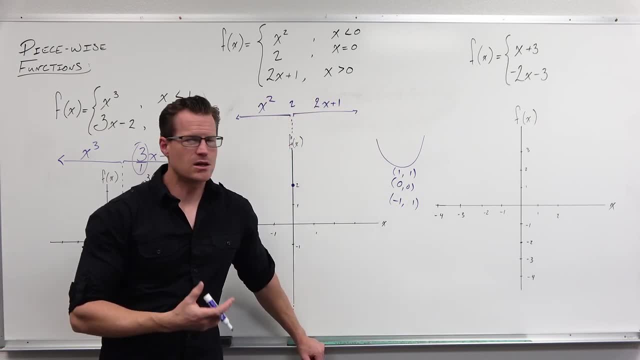 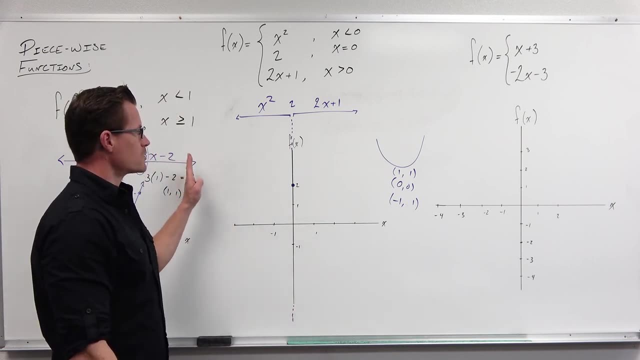 squared, I get positive 1. It's an even function and we need to know what even functions mean. They have symmetry about the y-axis. So I'm going to look at this and go: all right, I'm going to graph x squared, but I'm only going to graph it up until this boundary, So I'm going to be able to. 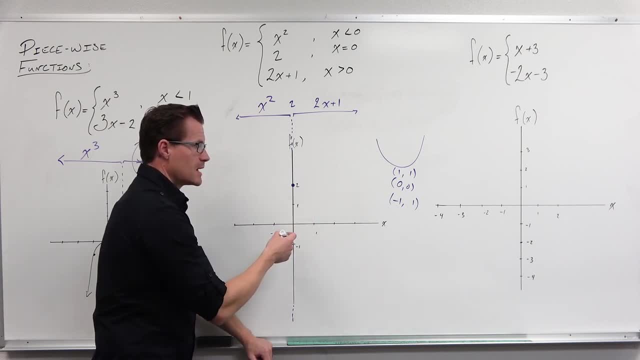 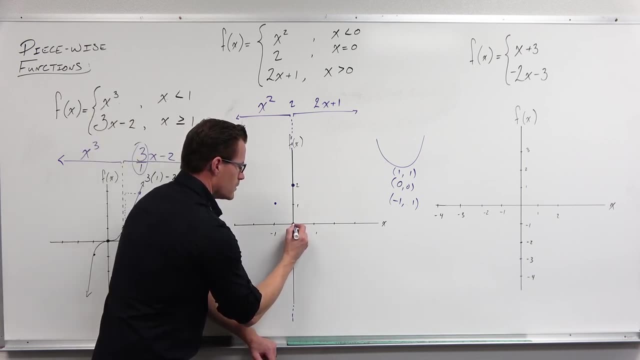 graph the 0, 0.. I'm going to be able to graph the negative 1, positive 1.. Here's negative 1, positive 1.. Here's 0, 0.. My parabola looks like: well, it can't cross over to here. I used 2x plus 1 over. 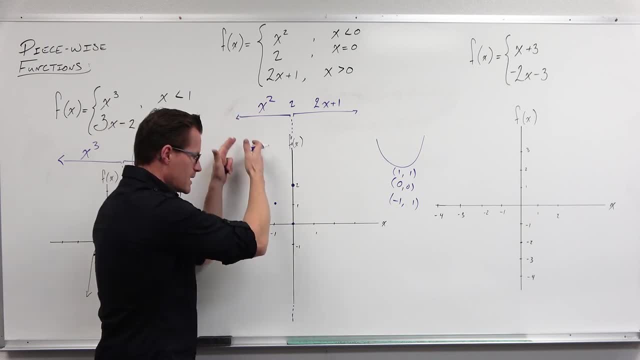 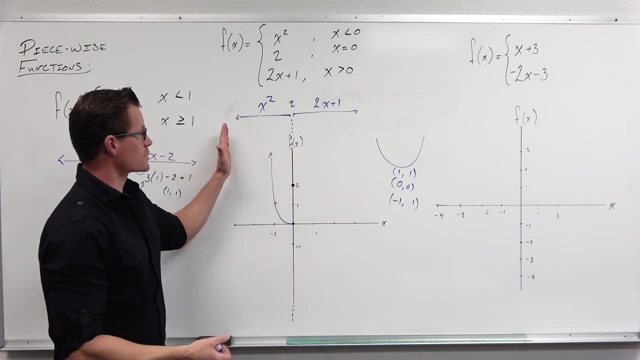 there. So for my parabola, I'm going to graph it, just like a parabola always is, and it's going to stop right at our boundary. So our parabola looks like that: I've graphed x squared. I've graphed. 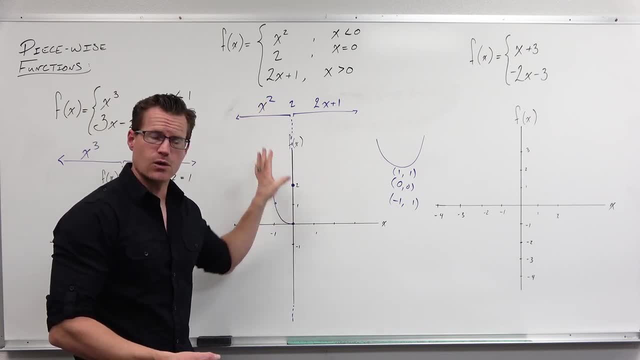 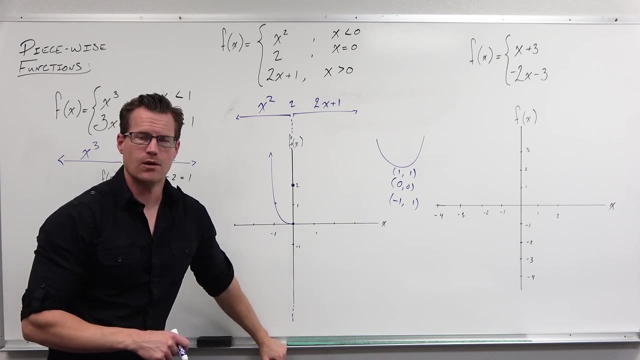 a parabola, but I've only done it in the interval for which it's defined, only on that particular domain, all the way up until our boundary. You should see the mistake right now. Man, I'm really hoping you see the mistake right now. 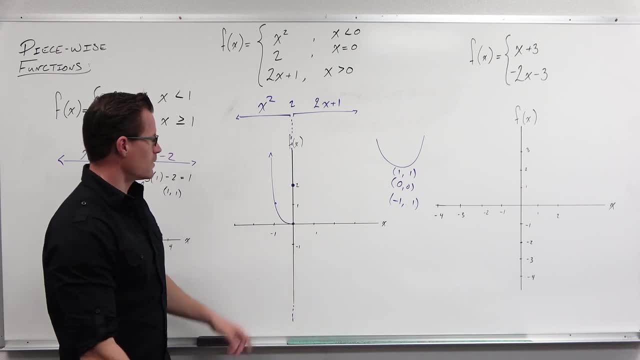 Right now is this a function? Right now, if you look at it and go, hey, is it a function up until this boundary? Yep, Yeah, For all these input values of x, I have one specific output. You can plug in negative 2 or negative whatever, and you get these output values. Mine's a little bit too. 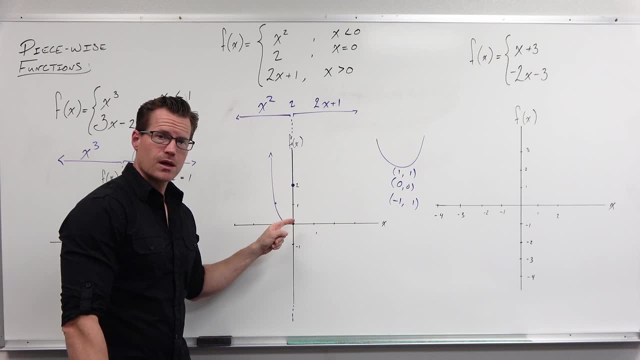 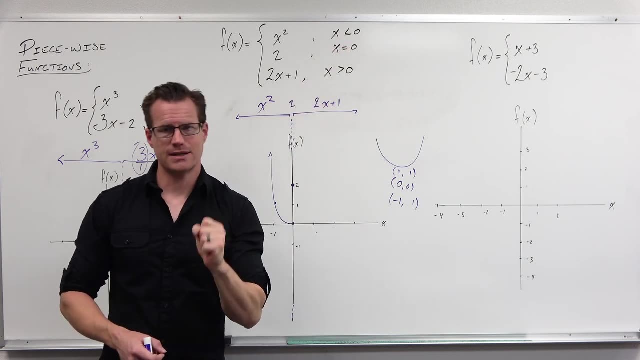 steep here, But at 0, this is a problem. So we go back to what I talked over here: For every single boundary that does not have an equals, you must not have a solid circle. So what this says is that you're going to graph a parabola. Yeah, 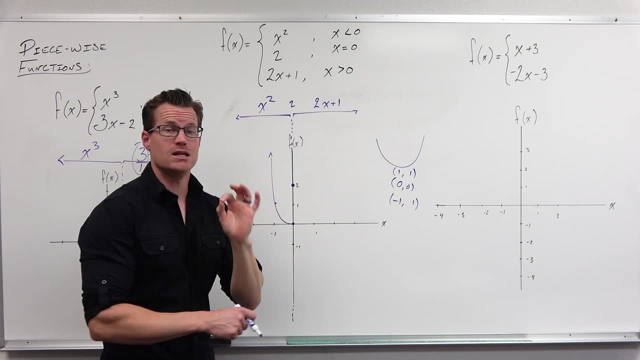 You're going to graph it on this interval, No problem, But when you get to 0, you need to not include it. So I've graphed my parabola. I'm on this interval, But when I get to 0, I'm going to. 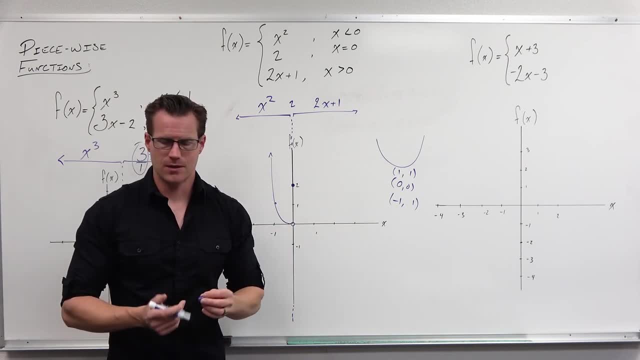 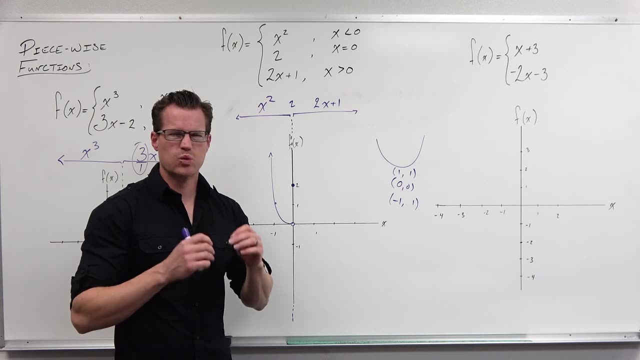 not include that as an output value. It's not there. Now you can plug in negative 0.00000000001, and you can square it. It's going to be really, really close to 0.. It's going to be right there. 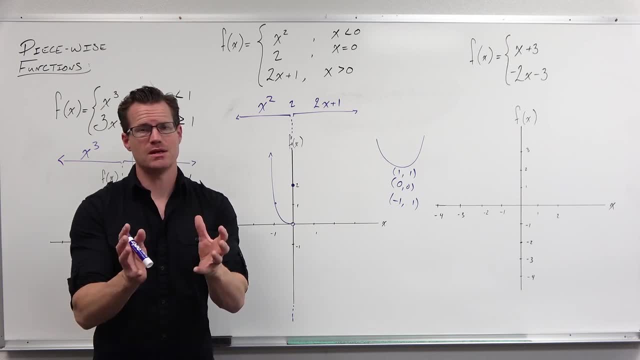 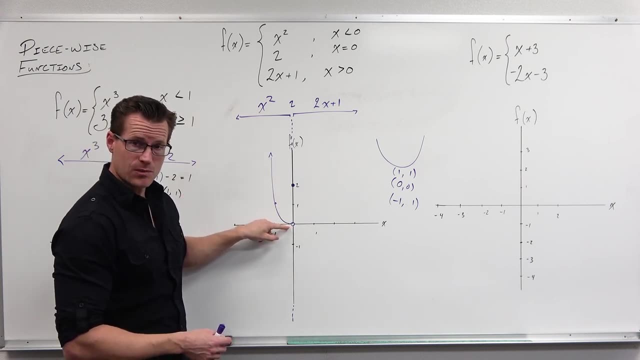 but we're just missing that output value. That has to be there in your head right now, if that makes sense. So we go. all right, I've graphed x squared. I've graphed it to my boundary. I am not including that endpoint because it's not included. Be like a parentheses The endpoint. 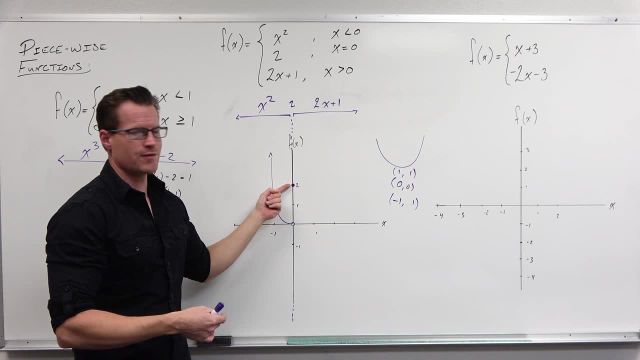 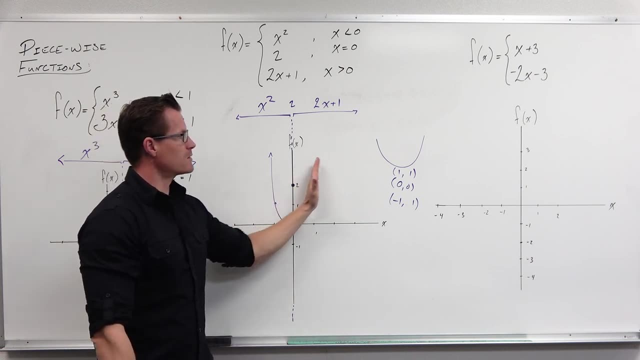 is not included there: 2, 0, we're taking care of that. where that point is what that output is for that value of 0.. Now the last one. I'm going to graph: 2x plus 1.. For everything greater than 0 on. 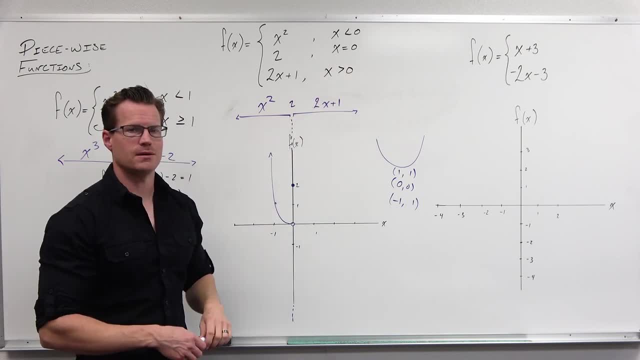 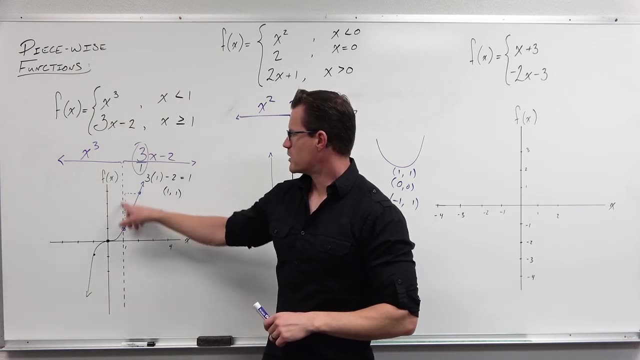 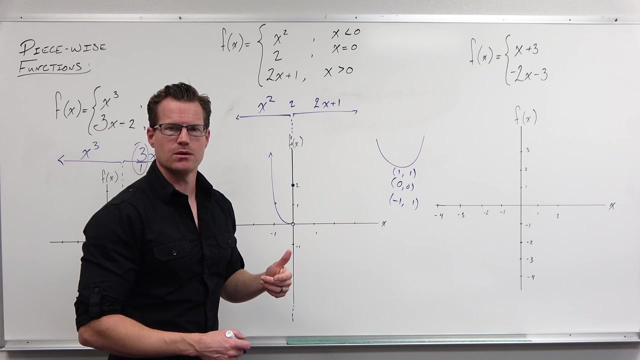 this interval x-axis, for which this function is defined on my domain. I'm going to graph this. So how to do it? Well, what I told you is plug in the value of your separation or your boundary number. So I'm going to plug in 0.. Well, I thought you couldn't plug in 0.. Well, we're going to outsmart. 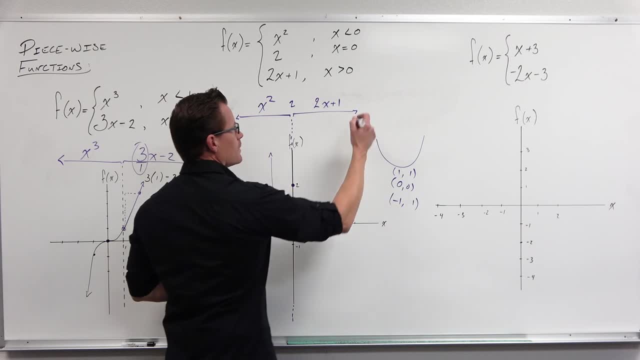 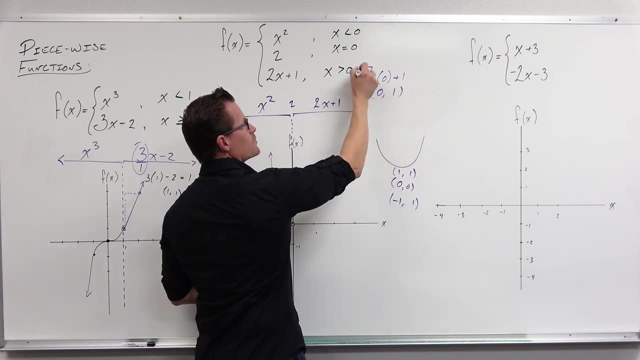 this thing. We're going to plug in 0 to this, 2 times 0 plus 1, we're going to get 1.. So if I plug in 0 to this function- which I know that I can't do- I'm going to get a value of 1.. Here's what. 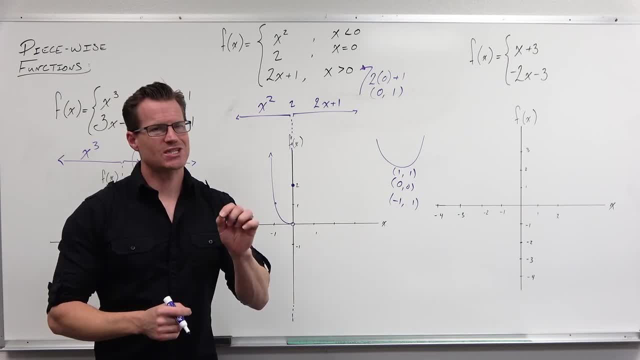 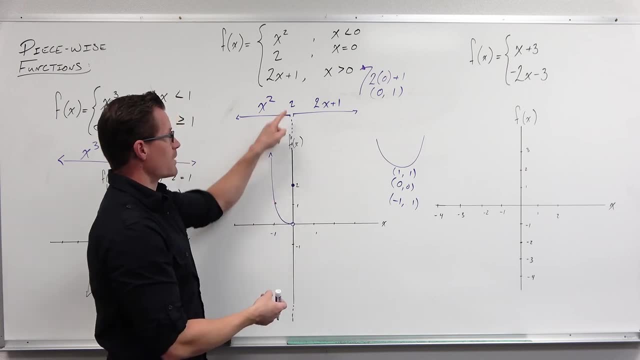 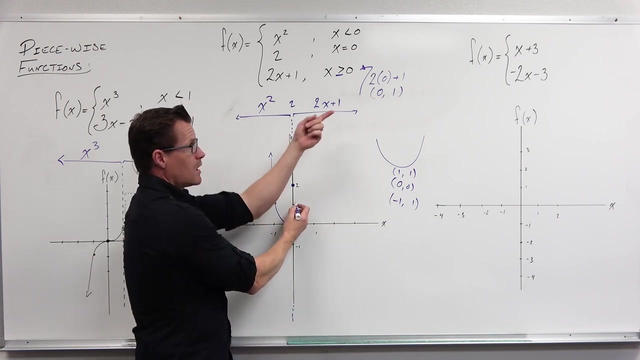 that means That gives you a place to start. It just says: just don't include the actual output value- What, What? Plug it in. But then when you say, all right, I would, normally if this was here, if that was there, you'd be here at 0,1.. Obviously. 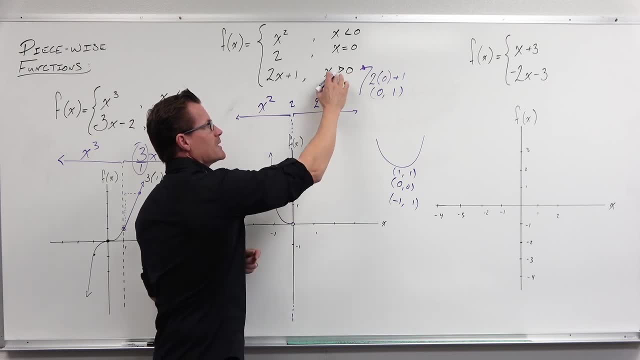 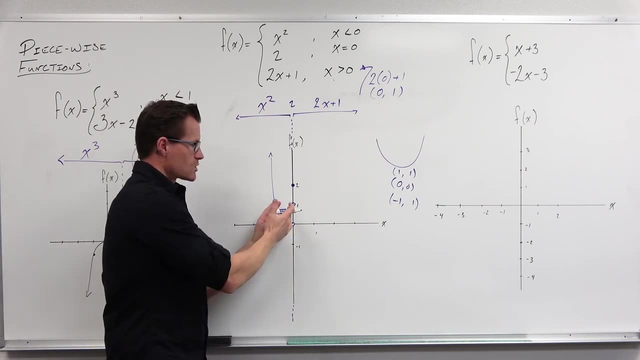 you'd be there. Since it's not included, we're saying, yeah, I would start there, but I'm just going to disinclude that little endpoint. Just give it an open circle and say my line is going to start just after that point, not at 1.. It's still. you plug in 0. You're just not including. 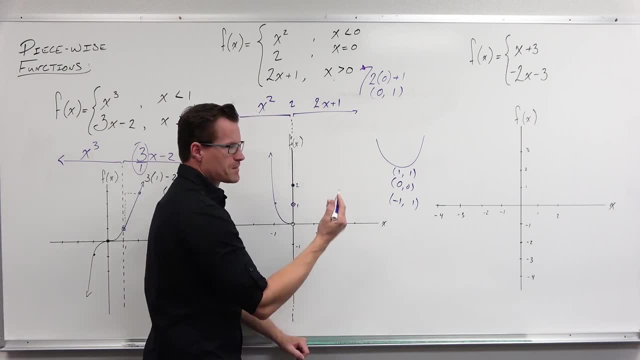 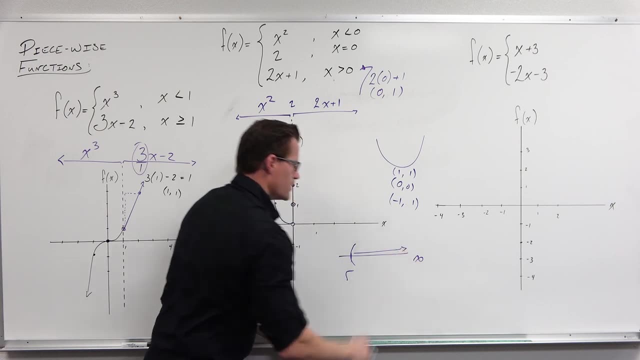 the endpoint, Kind of like a parentheses. if you said on a number line, here's 5 to a infinity, I'd say, well, I want to. I want to show this interval of my x-axis. I'm making up. 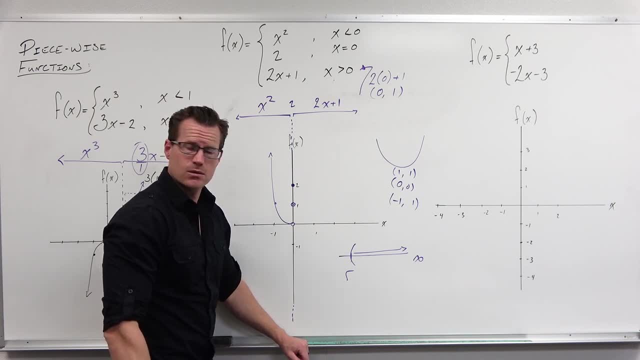 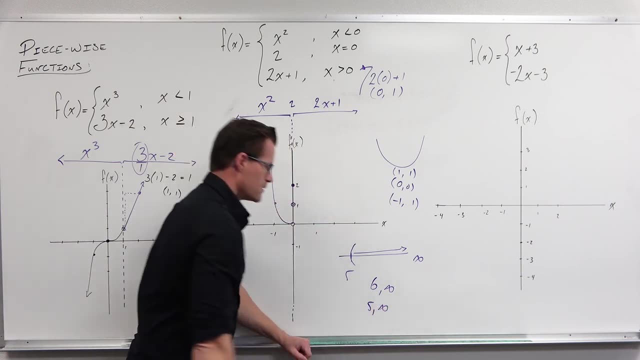 the 5. It's not coming from anywhere. Well, would you start at 6?? Would you say: oh, this goes from 6 to infinity. No, no, that wouldn't be right. You'd say: I'd start at 5 to infinity. but I can't. 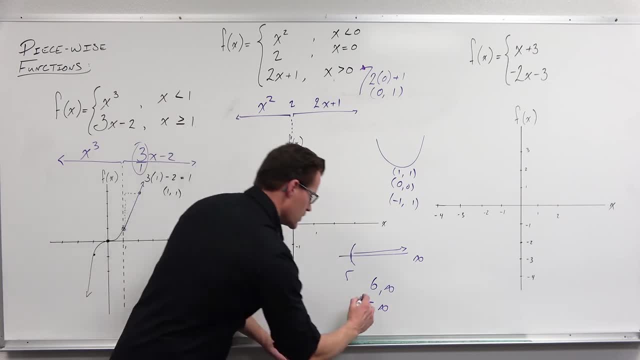 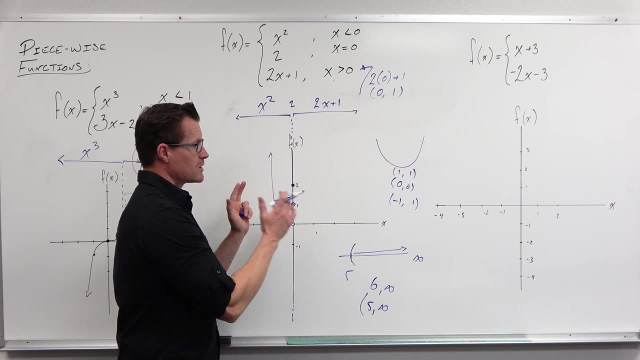 use a bracket because the 5 is not included. This says: oh, I would use, I'd use parentheses, I'd use kind of this open idea. That's what that open circle says. It says I want to, I want to make. 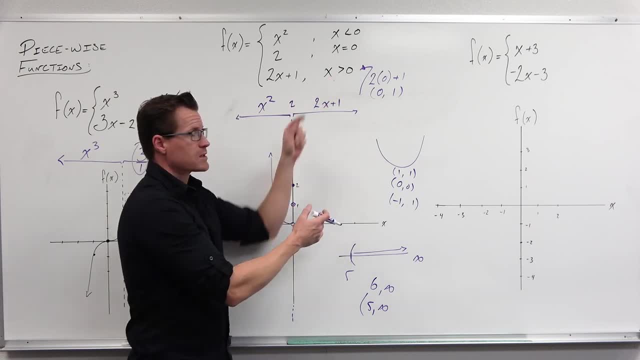 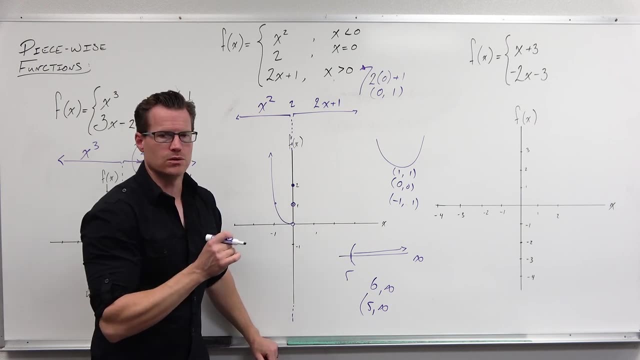 my x-axis for greater than 0 is defined, But greater than 0 is a parentheses idea. Greater than 0 is an open idea. Greater than 0 is a. yeah, you're just missing the endpoint. Just don't include the endpoint. Use an open circle. So for here, I'd say up to 0, don't include the endpoint. 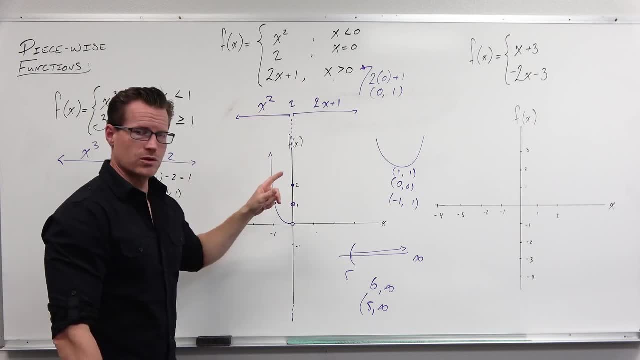 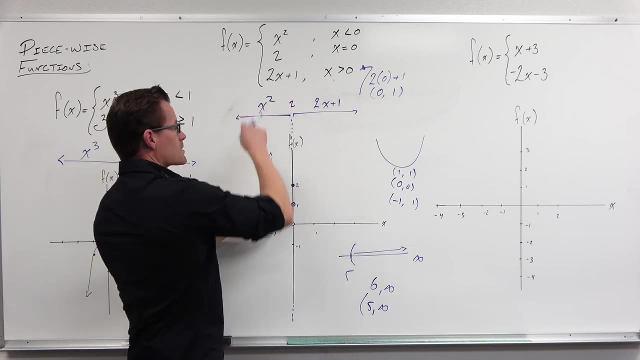 At 0,. I'm including the point After 0, don't include the endpoint, But I still basically plugged in 0. So that's where I'm starting, at 0, 1.. Now we understand, hopefully, that that's a. 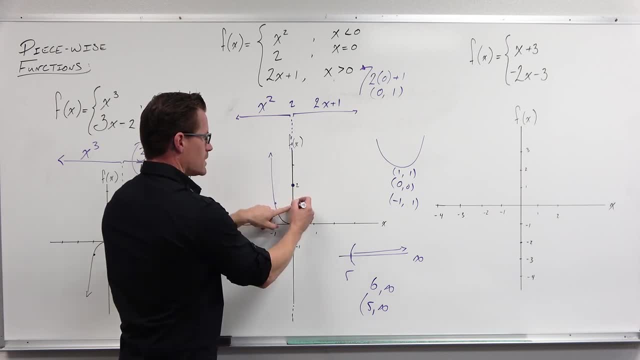 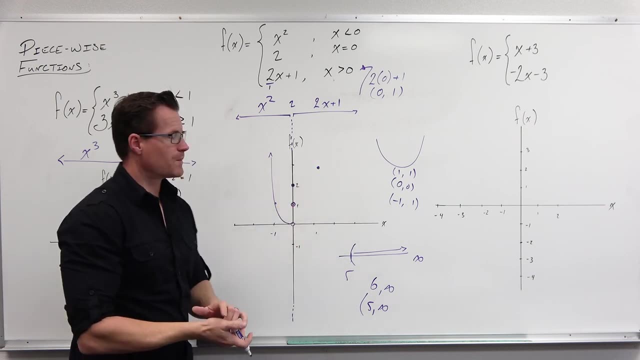 slope. The slope is 2 over 1.. So from 0 to infinity- I'm including the endpoint, So I'm that point. I would go up 2 over 1.. That point is there. On that value of 1, I am certainly. 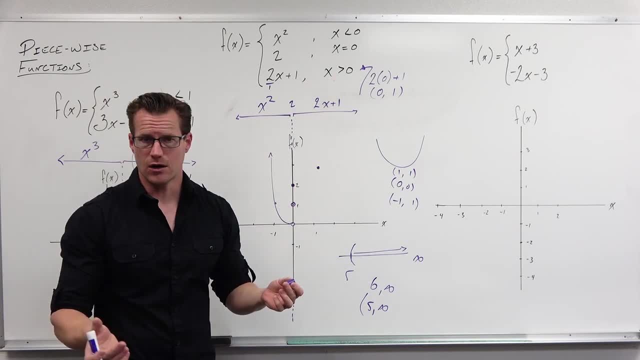 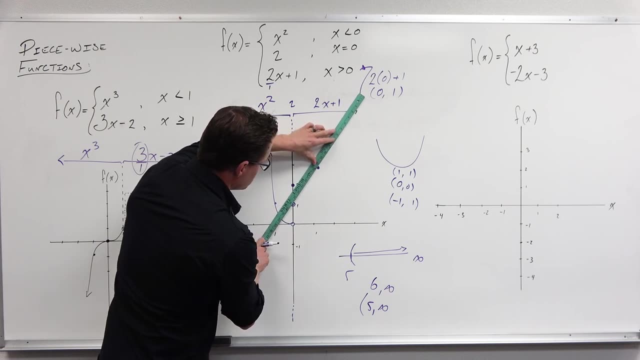 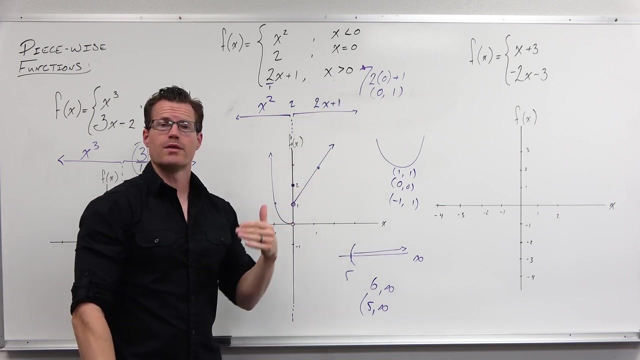 defined Everywhere after that open circle. I'm defined on my interval, So the only place we got to really worry about is the values that are on our boundary lines. Are they included or not? In this case, because I don't have an equals right here, I cannot include the endpoint or 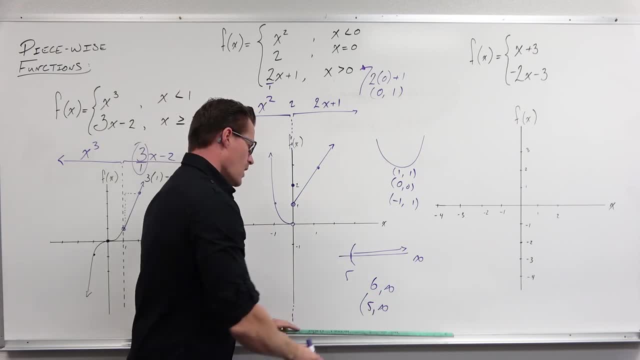 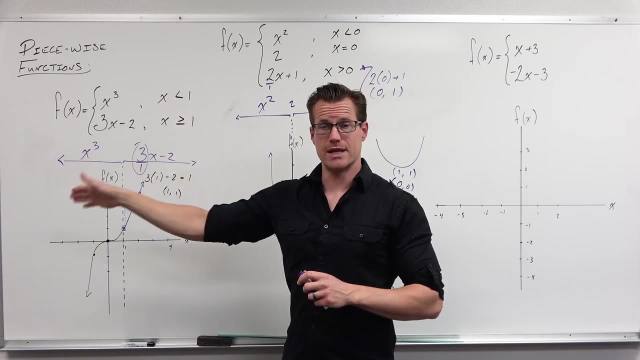 that value. that's on my boundary line, on my separation. I hope that makes sense. I hope you're understanding, or that I've taught you well enough, that our domain for our pieces show you intervals in the x-axis. What we do is we graph. 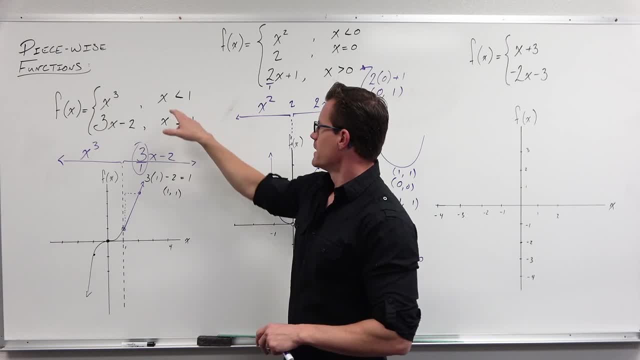 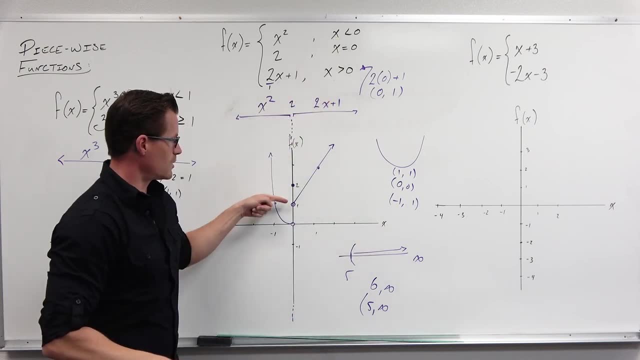 the pieces on those intervals. make sure that it fits. make sure that if you have no equals sign, you just have an open circle on that boundary. If we have no equals sign, we just have an open circle on that boundary. Equals sign: give us fill-in points. Sometimes we have these values. 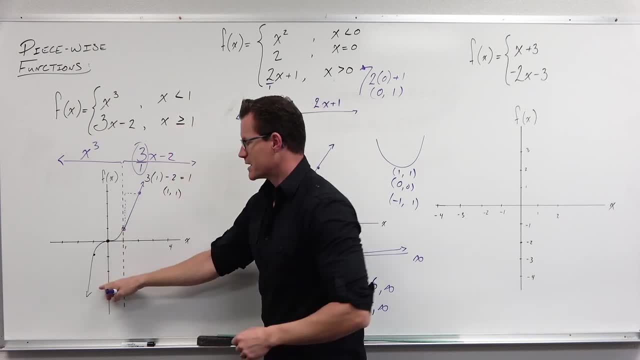 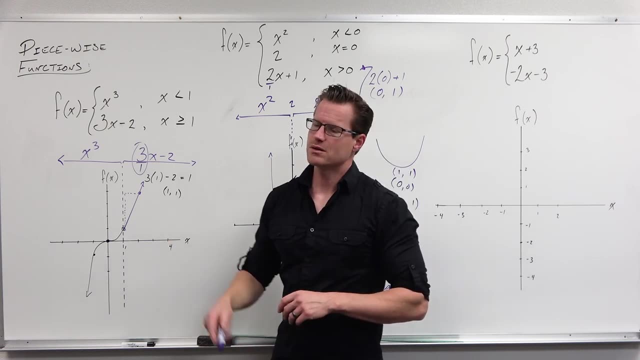 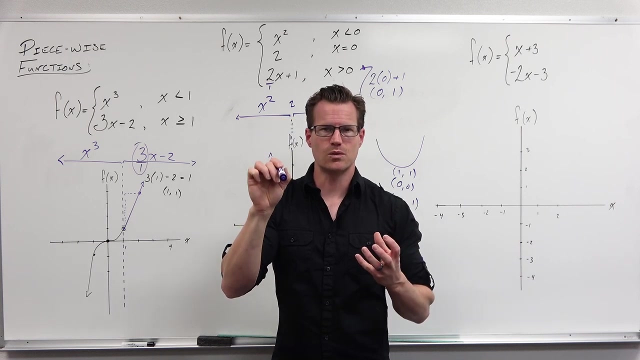 these lines, that are these sorry functions that work together and give us what's called a continuous function. This is a continuous function. What's continuous mean? Continuous means that for your interval, you can put your pencil on graph and you can graph the whole thing without picking it up. That's a really loose way to say continuous. 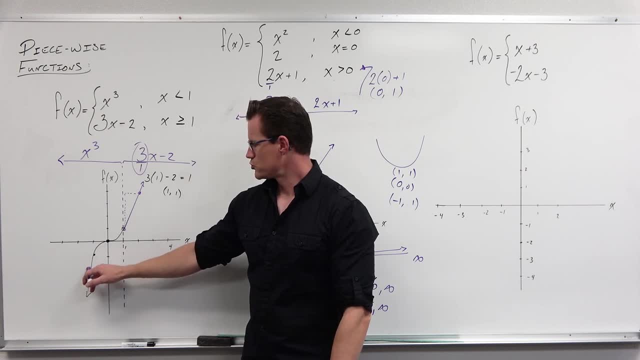 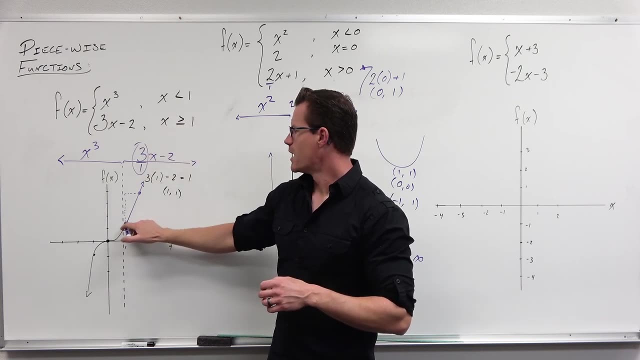 Do you all right. Can I graph this whole graph without picking it up? Oh, what about there? Oh, it's filled in. The one single missing point here is filled in by that graph. I can graph that whole function without picking up a pencil. 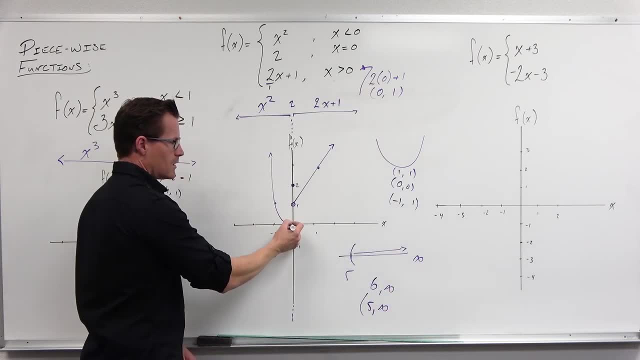 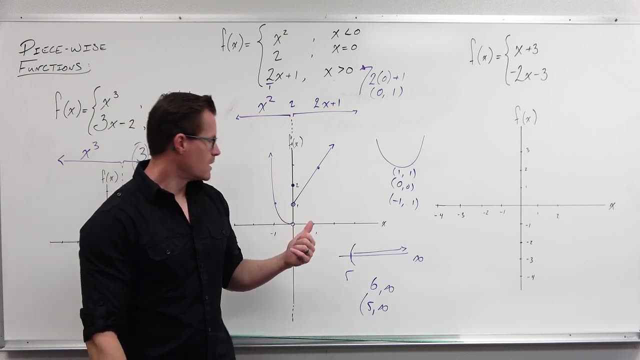 Can I do that here? Well, let's see I go this way. Oh man, Then I would jump to here, fill that out, jump back down to here and finish my function. This is not continuous. Notice how the piece or the point that's defined is not in this circle. Even if it was, it would fail to be. 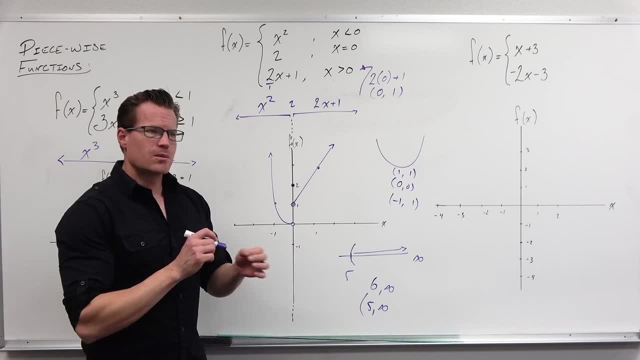 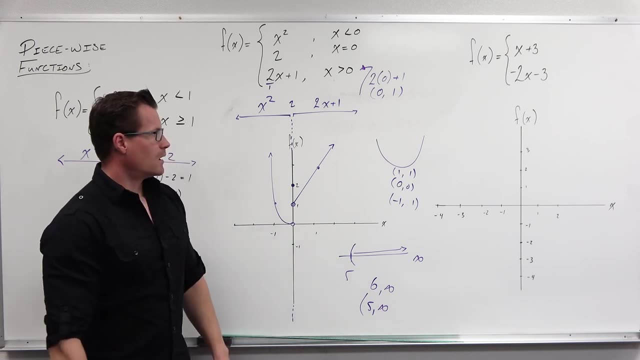 continuous, because that has an open circle and it's not. You're not able to graph this without picking your pencil off the paper. That's one way to think about continuity. All right, the last one. There's obviously something missing. I'm missing the directions here. Let me go ahead and make. 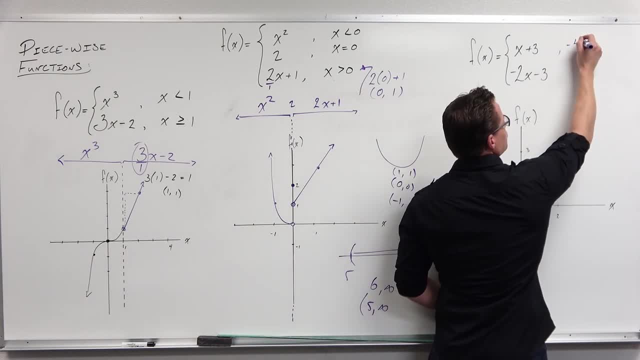 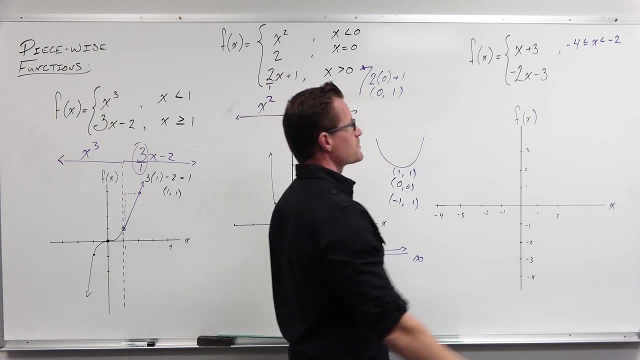 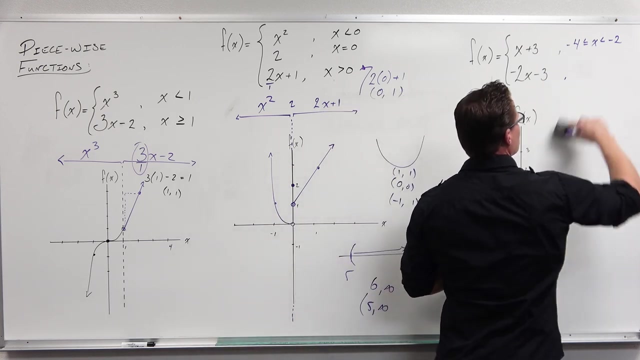 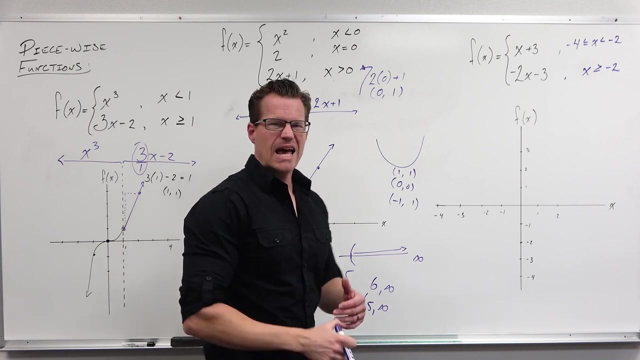 them up. Let's say that this is defined from negative four to negative two. This piece is defined from negative two onward. I'm not going to ask you to plug in values or evaluate, but you should be able to do that right now. You should be able to say: all right, if I'm plugging some. 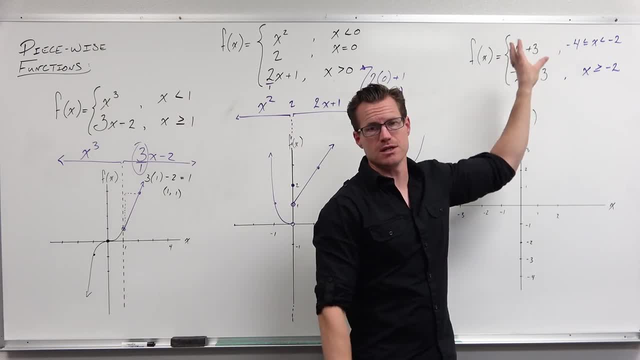 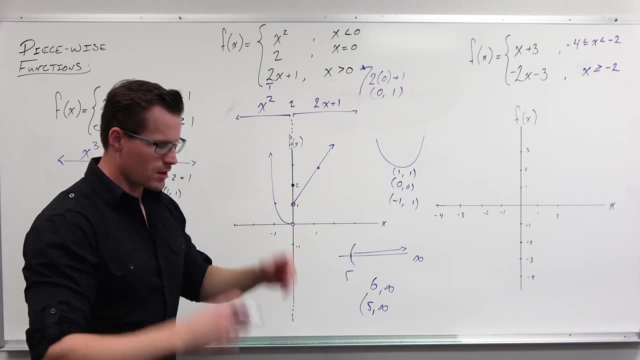 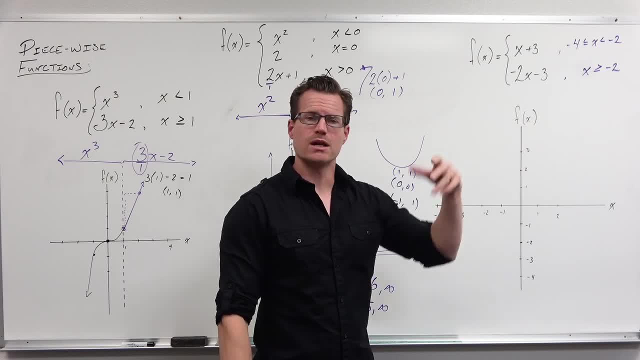 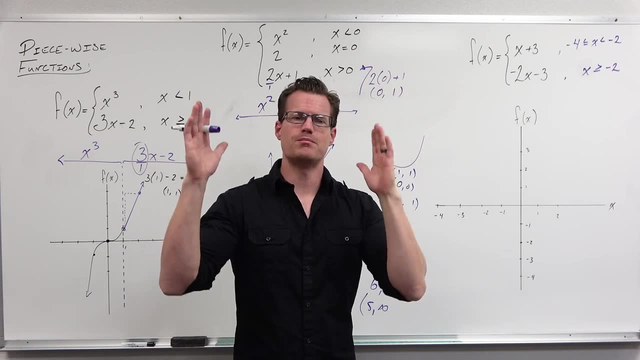 thinking. The way I'm thinking about it is: I'm going to look at my boundary values for each section of my domain. for each of these pieces I'm going to put a vertical dotted line saying this is the boundary for the interval, My function. that piece is going to fit on these. 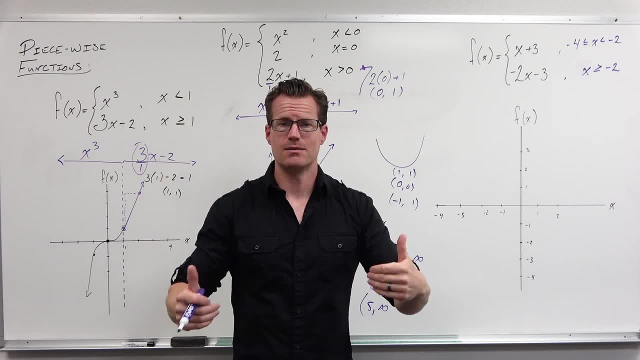 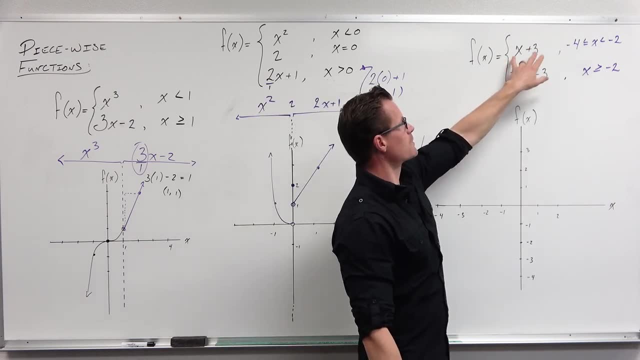 intervals, for which I'm now kind of delineating my intervals on my x-axis. I'm going to say where the function fits. That's what I'm going to do. My first piece: x plus three. this is defined on the x-axis from negative four to negative two. I'm going to put a vertical dotted line saying 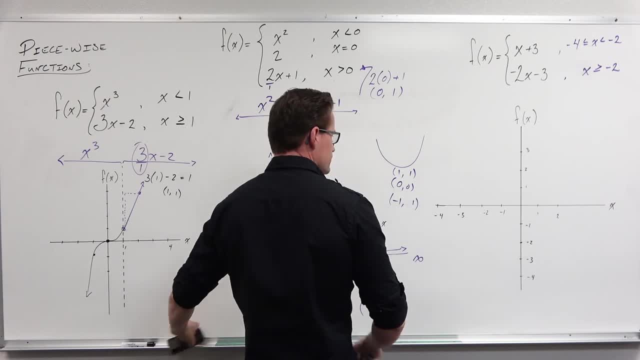 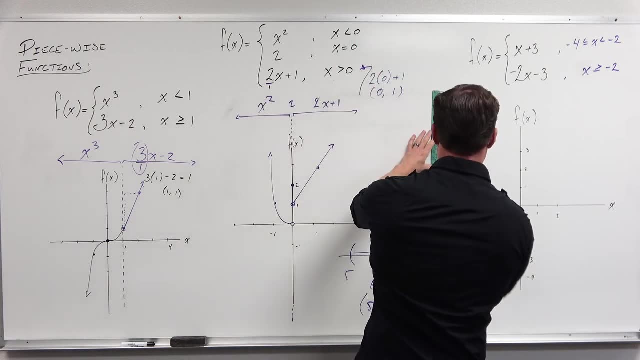 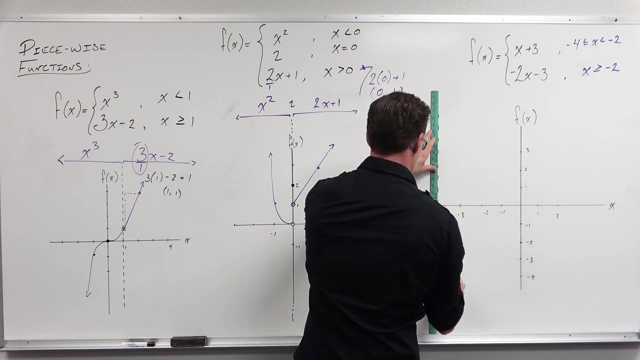 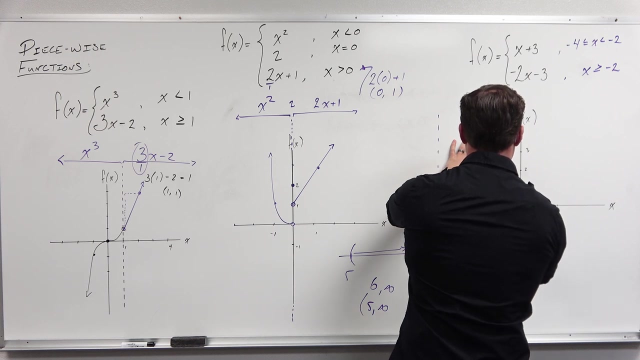 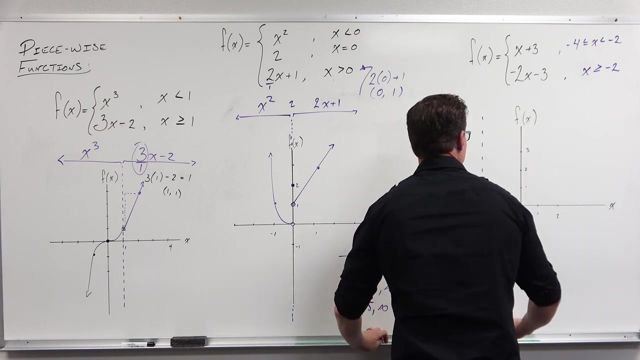 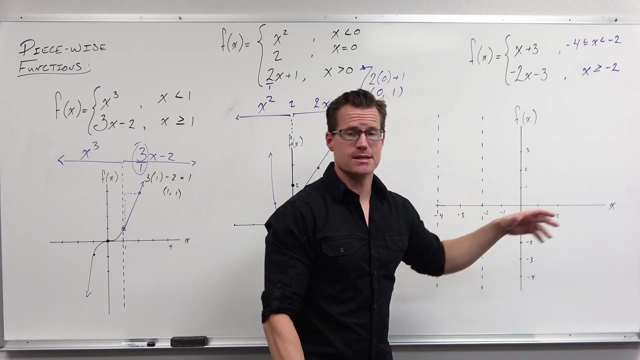 negative two: I'm going to go to those boundaries. Here's negative four. Here's negative two. I'm going to put a vertical dotted line. So I've looked at it and said this piece has this for a domain. Our domain always separates our x-axis. 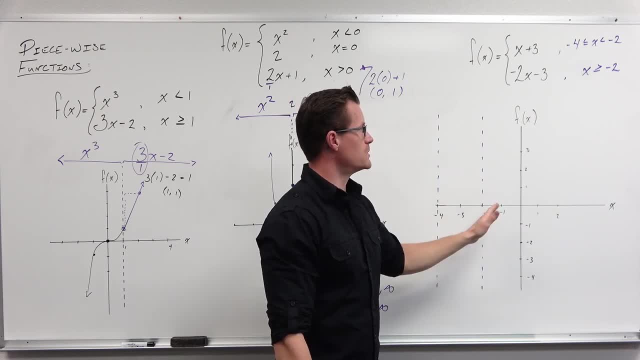 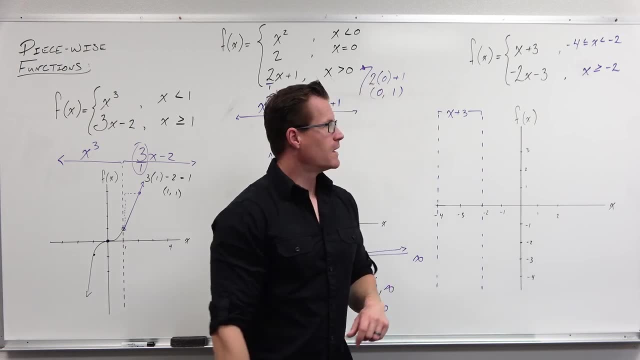 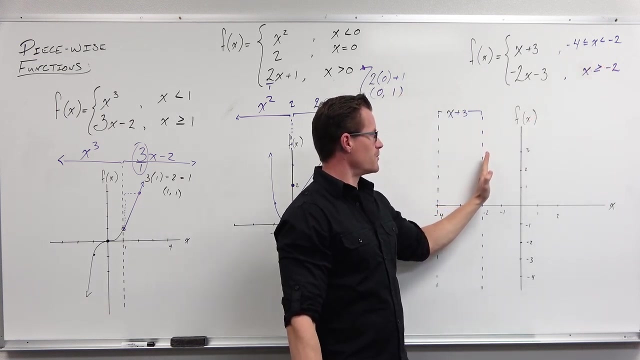 in the intervals. The interval is negative four to negative two, And I know that x plus three is going to fit in that particular interval. Now the next interval. well, because this has the same boundary number, I'm going to say that from everything from negative two onward, x is greater. 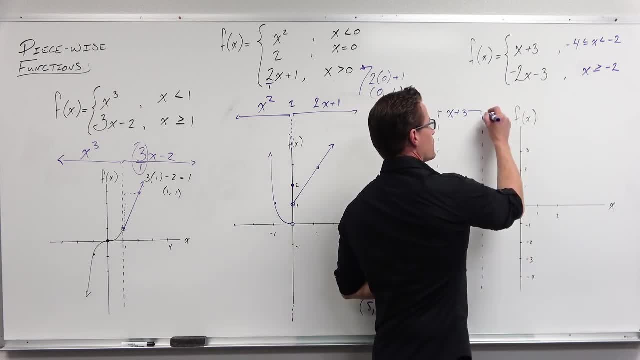 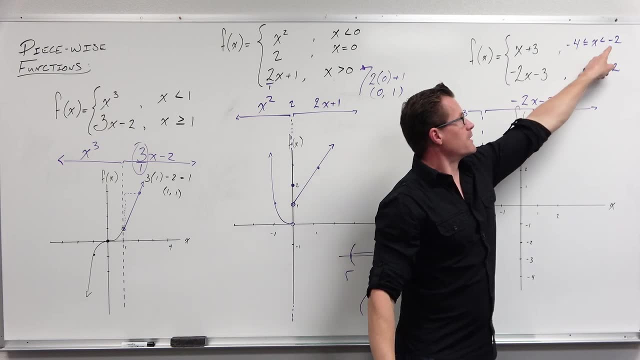 than that. I'm going to be using negative four. I'm going to put a vertical dotted line saying negative two x plus three. So from here onward, that's this piece of our function. Notice something? Negative two, negative two. This one doesn't have an equals. That one does. Is it going? 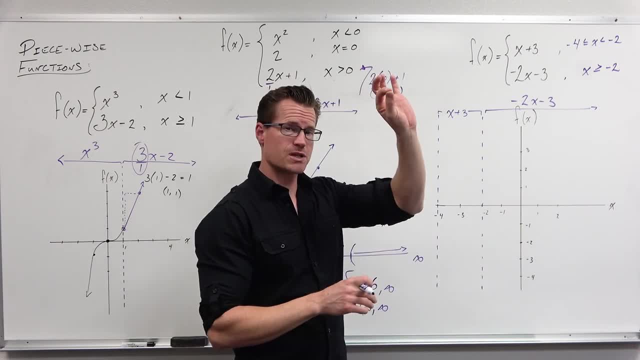 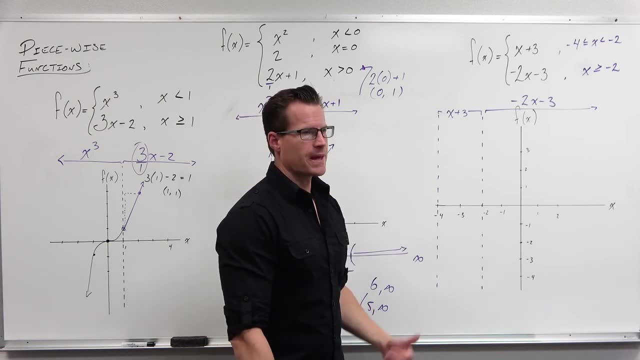 to be continuous. I don't know, We'll see when we graph it. If we have to jump somewhere, then it's not continuous, It fills in the hole. then it is One more thing. I don't have to have a piecewise. 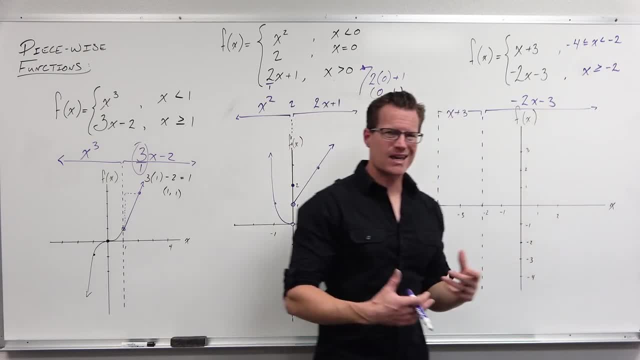 function that has this number the same as this. I could do some weird things. I could do things like go from one to the other. I could do something like this. I could do something like this. I could do something like negative four to negative two. And then what if this was two? What if that? 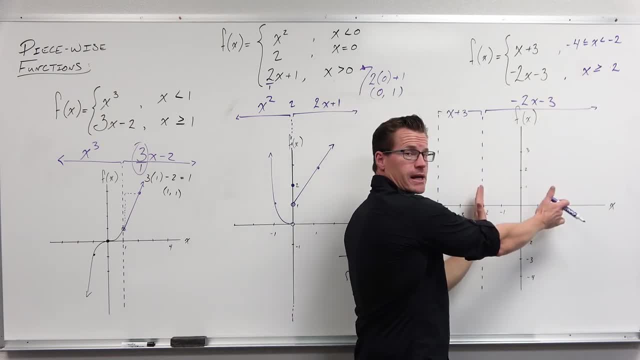 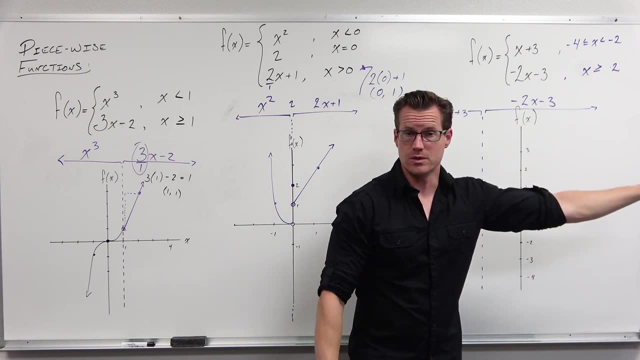 wasn't there, Well then I wouldn't have anything defined. It would say: there's no piece for this interval or function. I can now have a boundary two and then go on to another value or go to infinity. It doesn't really have to have the same numbers as a boundary. This one happens to. 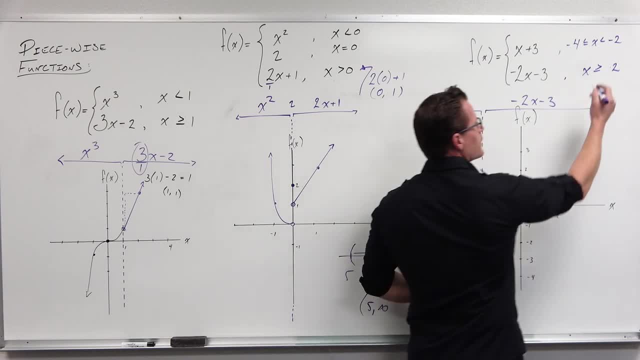 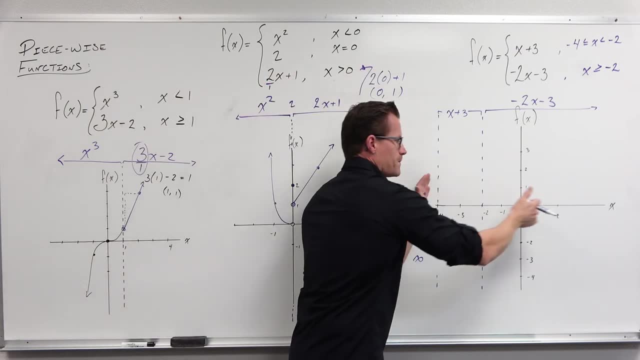 and most of them do. But I just want to make sure that you understand that You don't have to have the same number here and here. So we've looked at it. We said our domain is this for these pieces. We've defined our x-axis as having those particular intervals for which our pieces are. 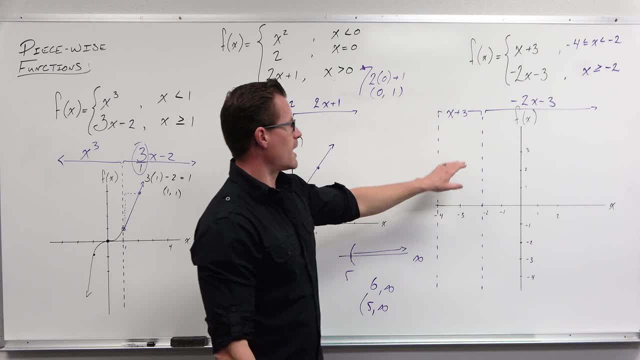 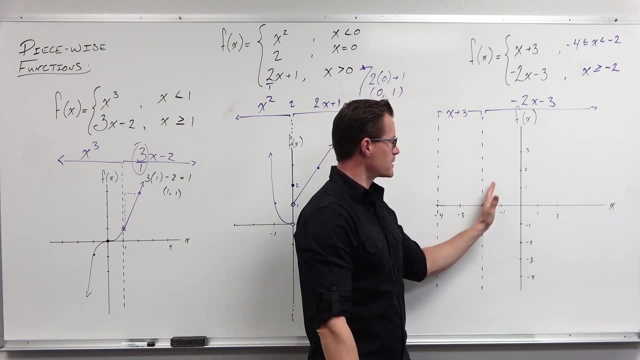 defined. They have a domain. Now what we're going to do is we're going to say we're going to graph. well, I'm going to graph the function that has the y-axis first. It's a little bit easier for me to do that. So I'm looking at this interval and saying this interval right here has my y-axis. 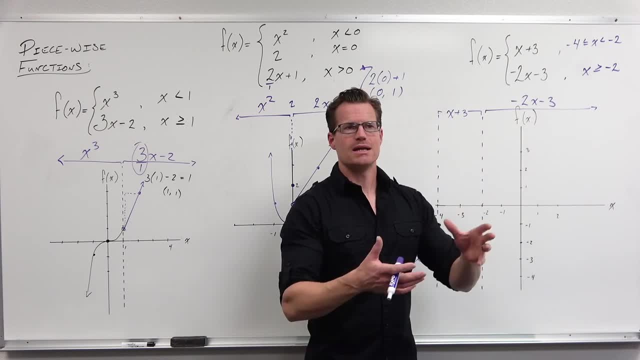 I'm going to use that because it's easy to find a y-intercept. It's easy to go ahead and graph this function, So I'm going to go. all right, what's my y-intercept? I'm going to plug. 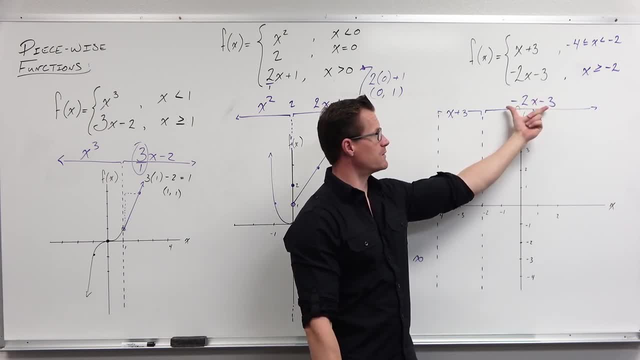 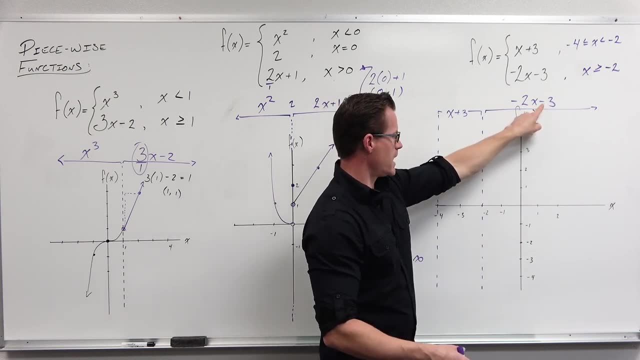 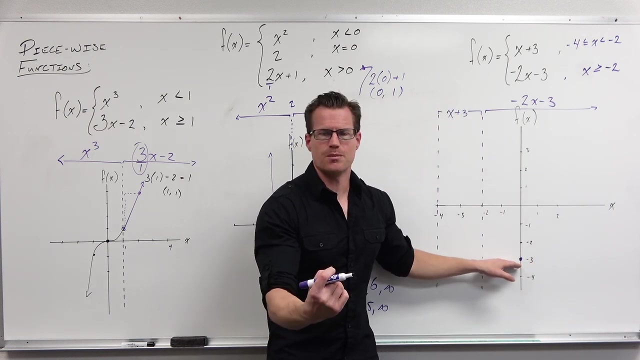 I'm going to understand. that's a line. This has a slope of negative two. So if I have a slope of negative two and I plug in zero- or we understand slope intercept form- this has a y-intercept of negative three. Notice how. that is certainly a point. It's not an open circle, It's clearly. 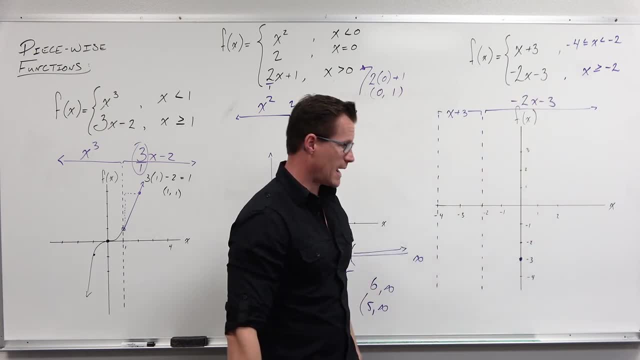 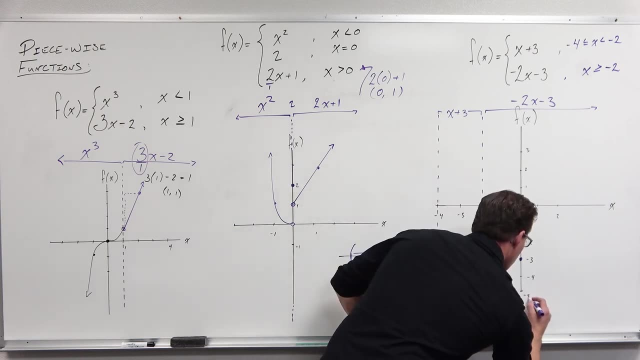 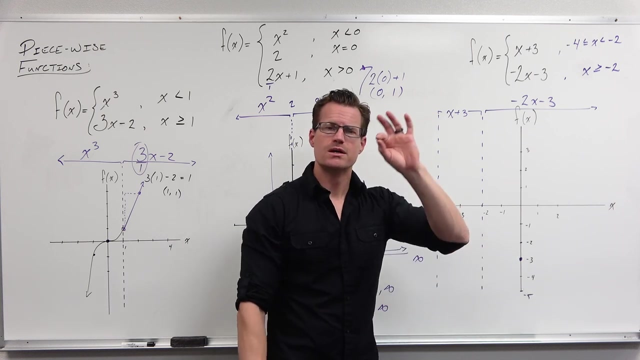 in the defined domain of that function. Its output is negative three. Then I'm going to think, all right, it also has a slope of negative two, Which means that I would go down two and right one, not left one. It's always. slope means a. 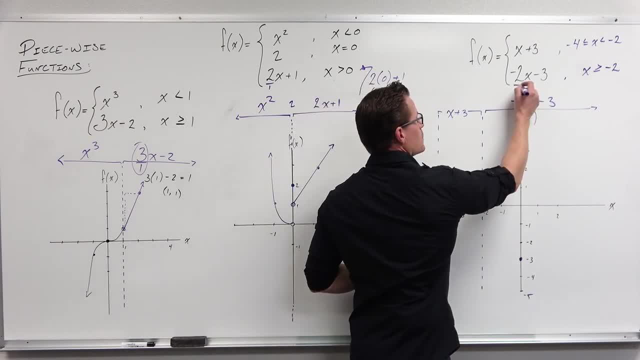 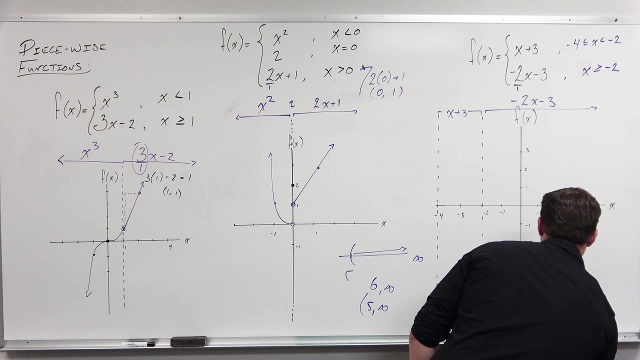 positive goes up, negative goes down. You're run. So this two over one says you're going to go to the right one. So let's see down two right one. That gives us our line, but we want to be a little. 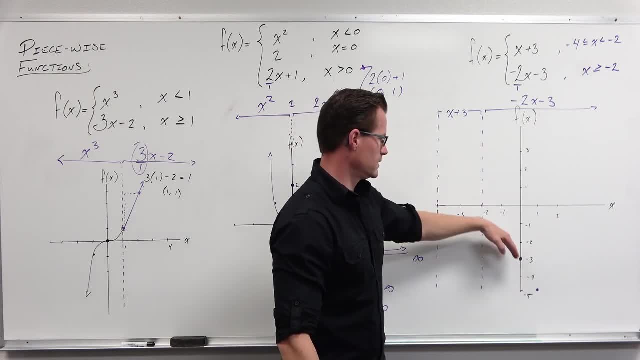 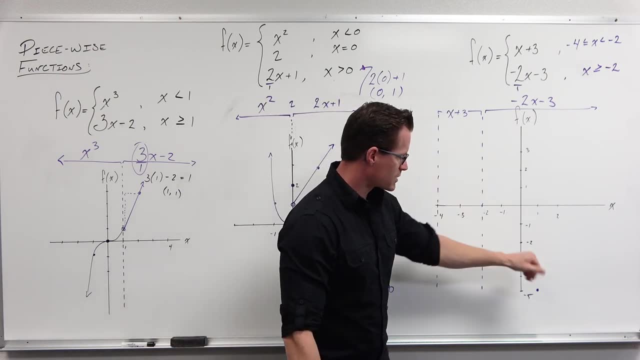 bit more specific. We don't want to just graph this thing and go: all right, I end up about here and I'm going to do one more thing. So I know where I cross the y-axis, I know where my next point is, but I'm also going to take my boundary. I'm going to plug this in the separating value. 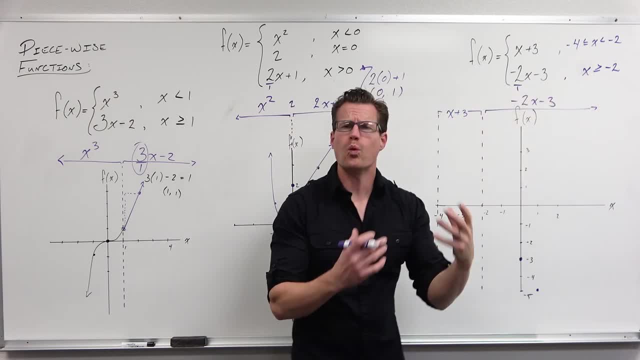 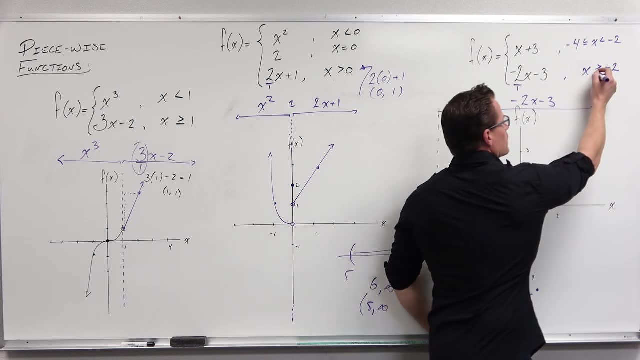 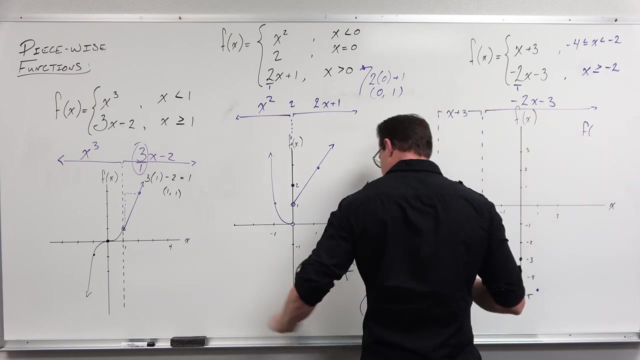 I'm going to plug it in here. It says it's defined. Even if it wasn't, guys, even if it wasn't defined, I would still plug in negative two. So let's pretend about this. for a second. Let's say it's equal. You're going to plug in negative two. So f of f of negative two. 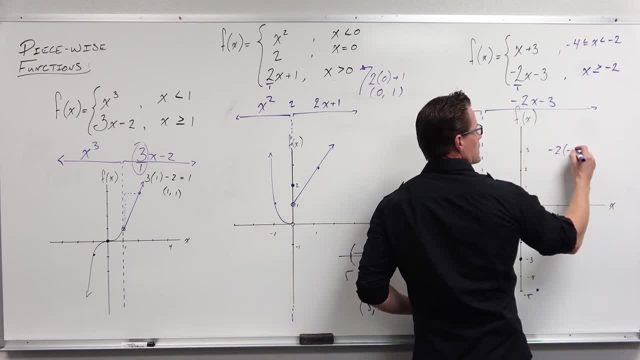 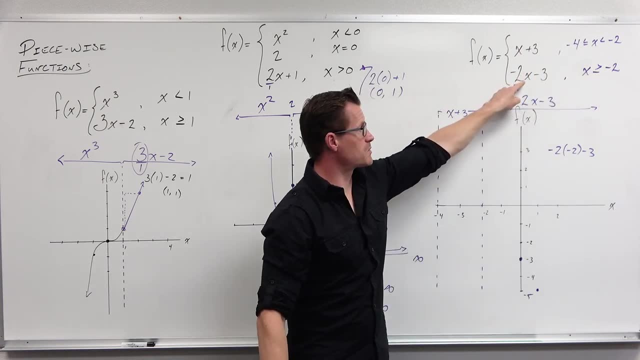 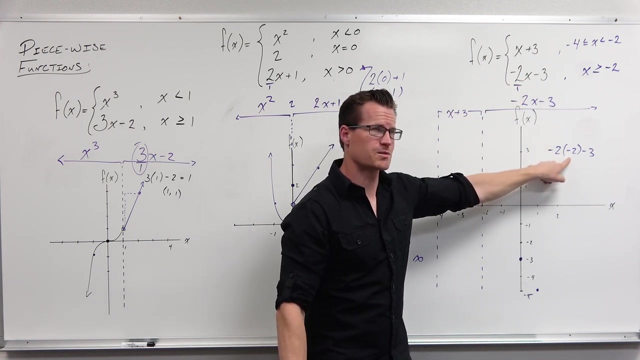 negative two times negative two minus three. So I'm taking my negative two, my boundary, my separating value. I'm plugging into this piece, no matter what, I would do this. So negative two into here. negative two times two is negative two. That's positive four. Positive four minus three is: 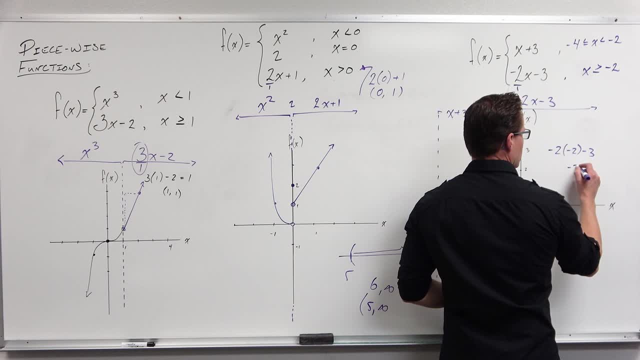 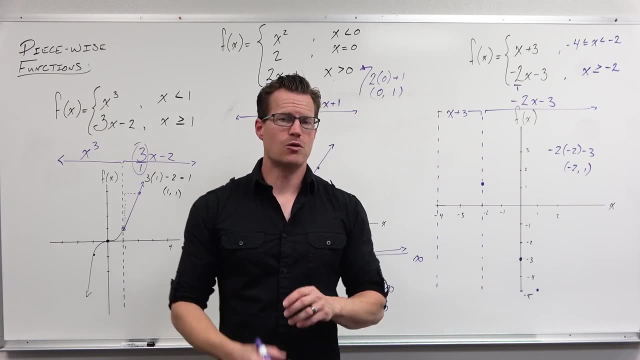 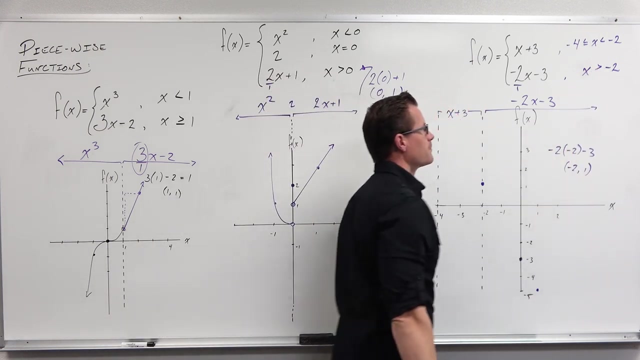 one Negative, two comma one. Now I told you that no matter what, we would plug that in. So please watch here. Let's say that this was not equal. Let's say that was not equal. I would do exactly the same thing. I'd take the negative. 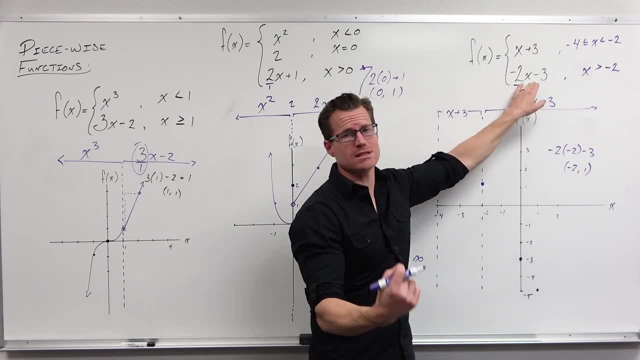 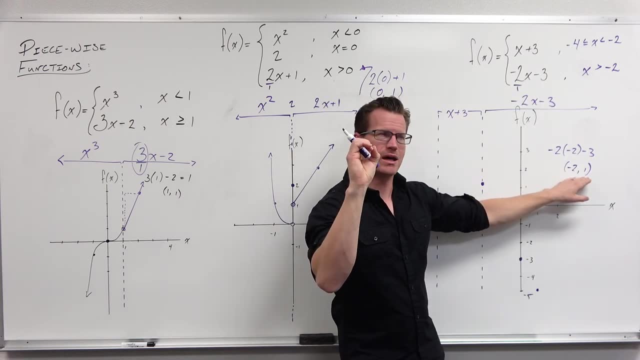 two, I would plug it into this piece. I know it's not going to exist and not have an output of that value. I know that. I know that this would be a point where I'd be missing well, an output where I'd be missing the point. Don't miss the point. So if I plugged in negative two, negative two. 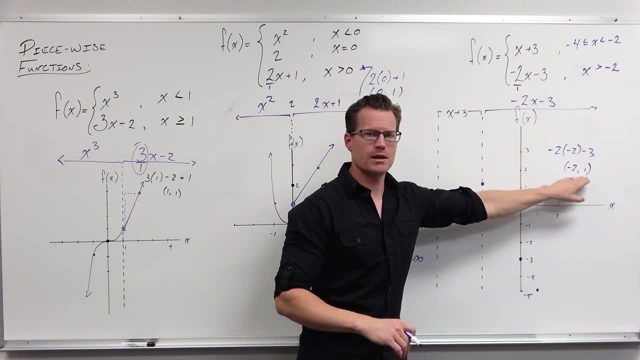 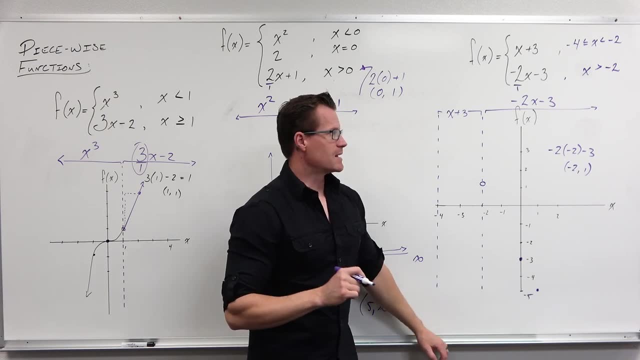 negative two, even if there's not an equal sign. that's it. My output would be one, but now it's missing. We'd still put that open circle. It would say that if that was included I'd have that value. 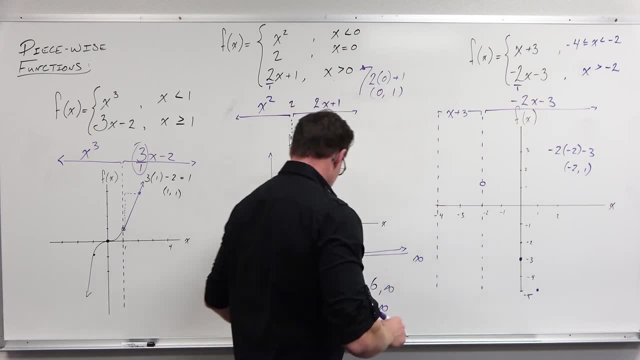 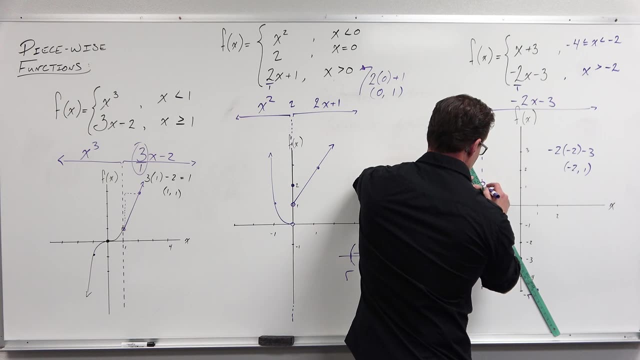 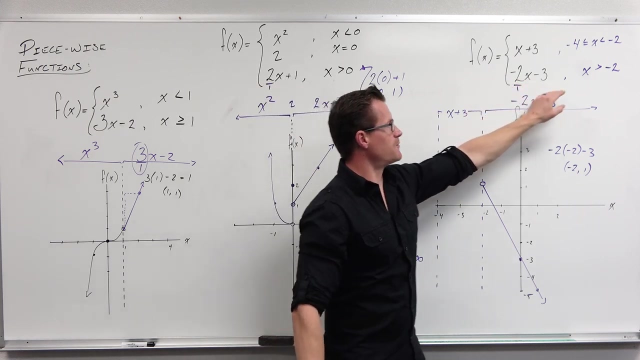 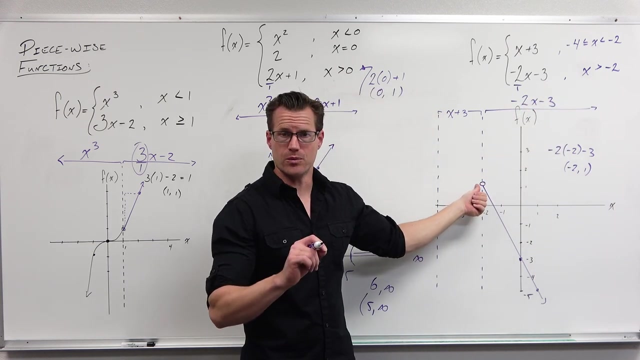 Since it's not included, I just I'm missing the point, But this line would still do this. It says this graph: this piece is defined for this interval from negative two onward. It just. if I don't have the equals, I would not define the output, but use it. Use where the output would be. 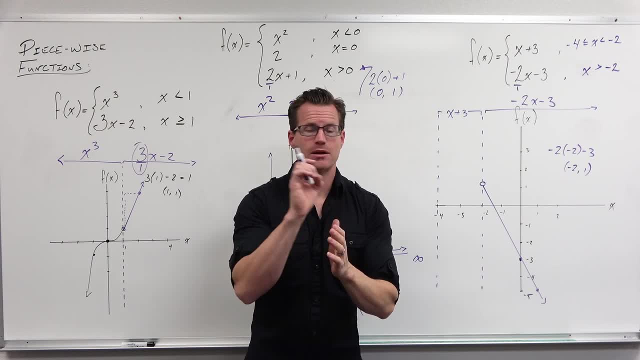 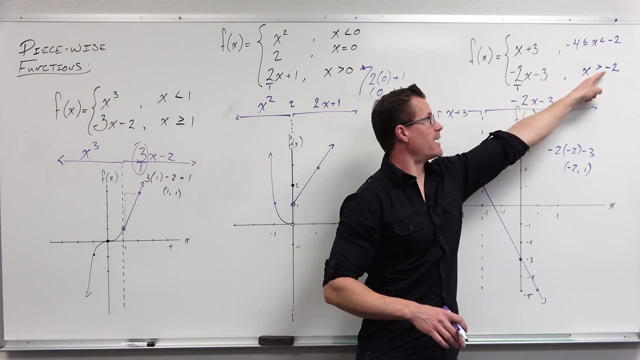 to give yourself an open circle to say: at the boundary, I'm just, I'm just not including the point, I'm missing the end point. That's how to use that. So we graphed the Y intercept, We've graphed our slope, We we plugged in the value, the separation, this boundary value of our domain. 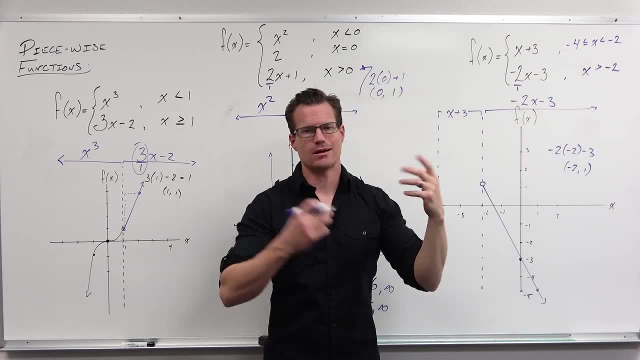 even though it wasn't even there, you still plug it in and say, I'm just not going to include, I'm just going to have it. So we're going to have an open circle instead of a solid circle. Now do we have to actually have an equal sign there? 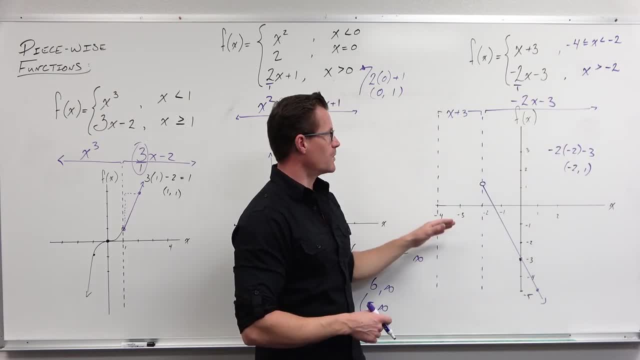 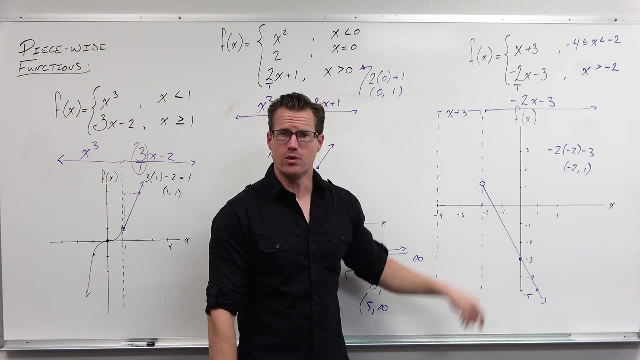 We don't. And if I, if I left it like this, I would have this: let's see, X plus three is going to look like like that. I would just have this, uh, this line, and then I'd have no end point there. 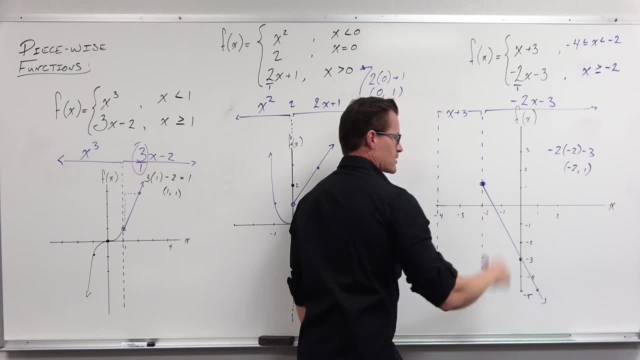 Now, if I do have an end point that just says that, all right, I have an actual value there and you're going to fill it in. That's the only difference there. So so again, equal sign, you got an end. 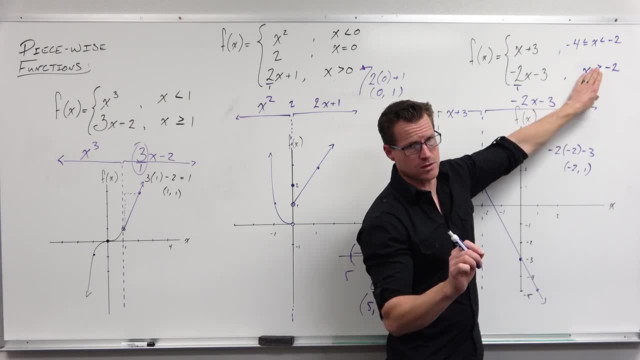 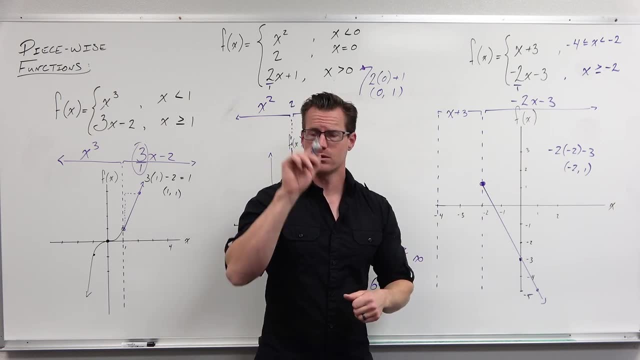 point: no equal sign. You still use the value. You still plug it in. You still get the same exact value for an output. You just show that you don't include it. with an open circle, no equals. open circle equals close it in. And now we're going to go ahead and graph the other. 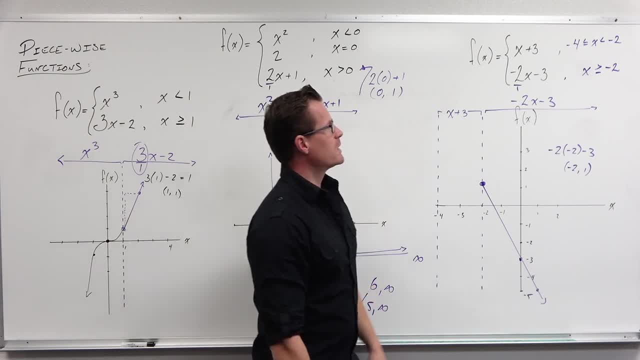 interval that says from negative four to negative two. I've got a line. You know what? We can just plug these values in Um. I'm never going to make it to my Y axis. This is only defined for this little interval, So I'm going to take negative four. I know it's a line. 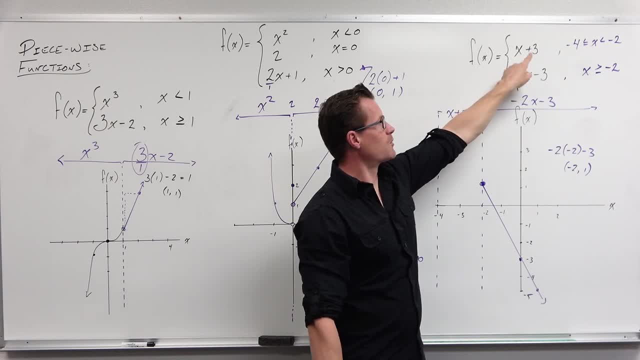 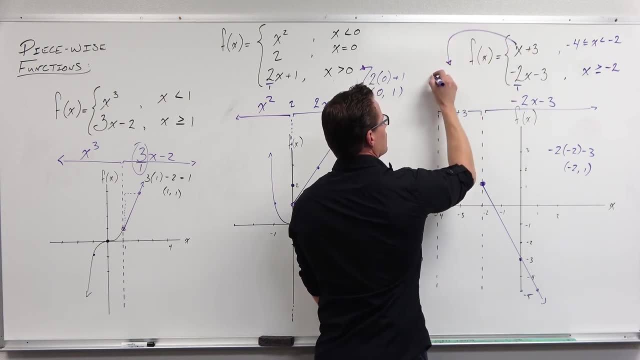 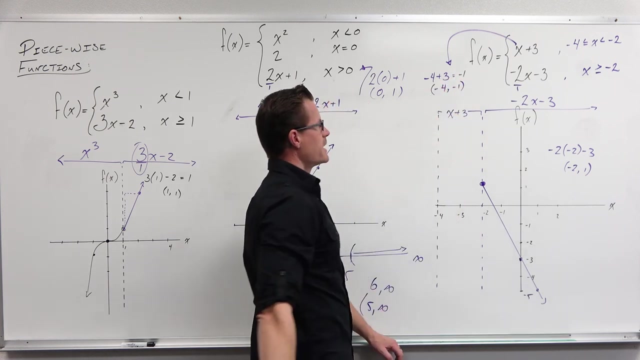 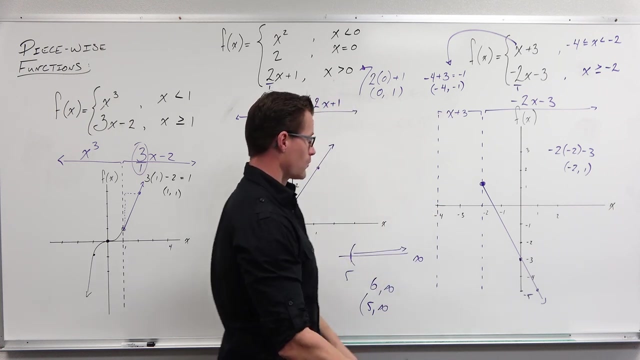 negative four. plugged in or evaluated, It's going to give us negative four plus three. That's negative one. In your head you need to be thinking that because that's equal this value, I can actually have an output at negative four- negative one. So negative four, negative one as a solid closed. 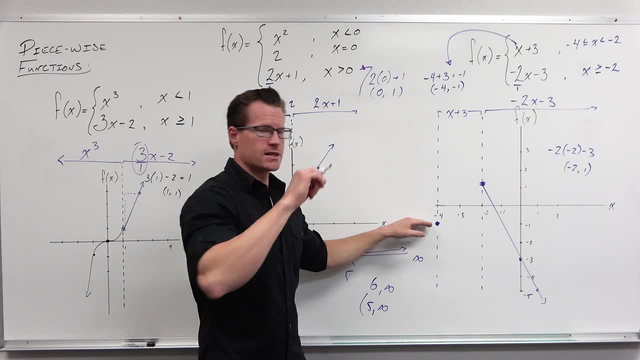 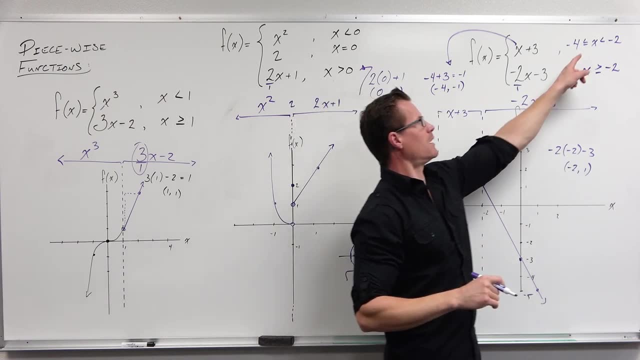 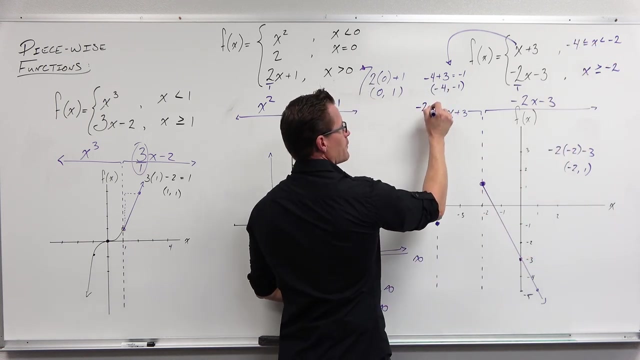 point That exists on the domain. That means that point exists and has an output that we have defined. How about negative two? I said what I don't. uh, I can't actually include it, I know, but plug it in anyway. All right At negative two. if I plug this in, negative two plus three is one. 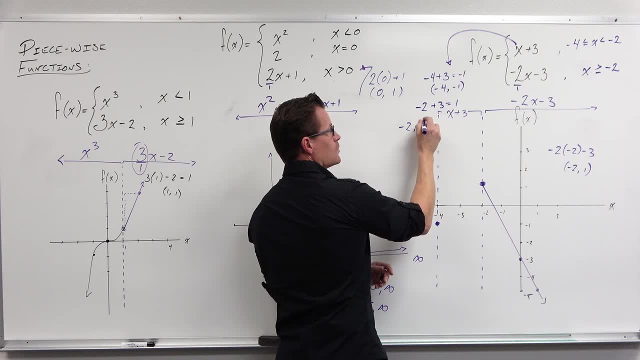 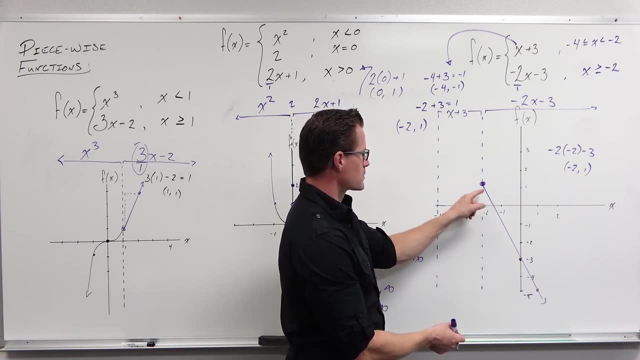 That means that my output value would be negative two, one. So I'm going to use that. I'm going to say, uh, here's negative two, Here's the value one. But wait, oh, there's already a point there. 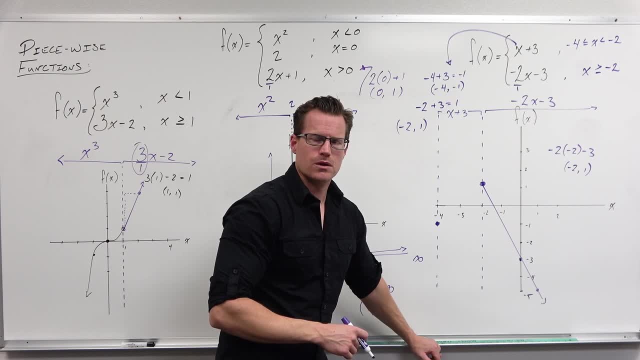 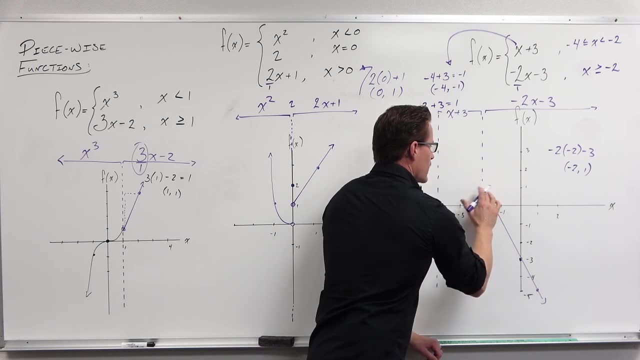 Can I put a point on a point? No, no, no, you can't. For that reason we'd say: oh hey, that's why that was open. That's like a little open circle. So what the if I erase this? what this graph would do is this would say: I have an open circle. 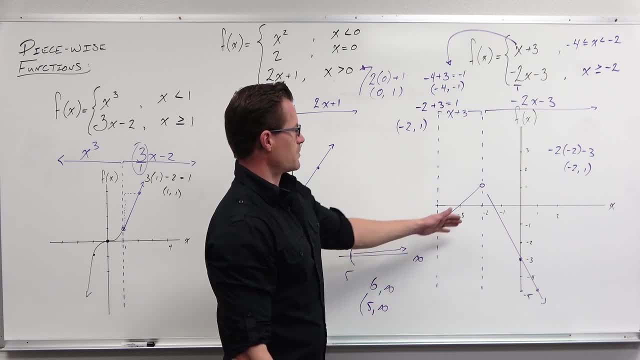 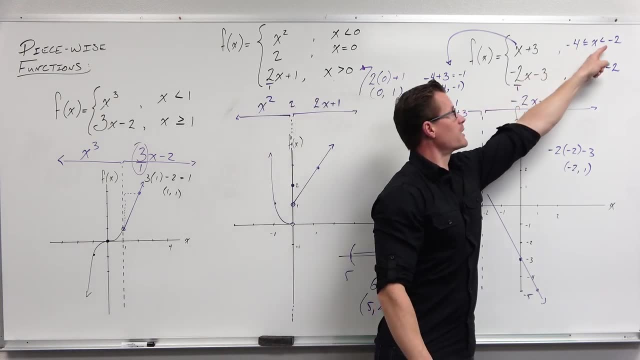 This function would go from here to here. In fact, if I plug in negative three, you get zero. You can see that that's true. But if I plugged in negative two for this particular function function, this would say you plug in negative 2, it's going to give you an open circle. It was. 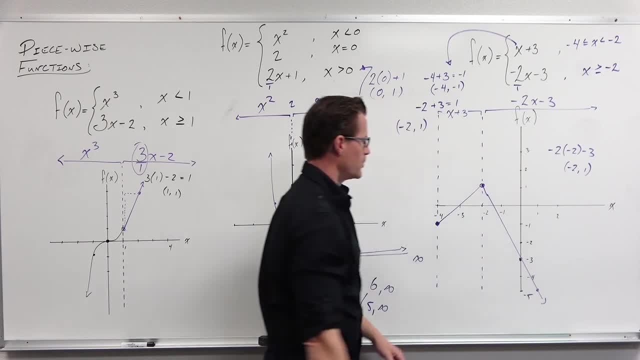 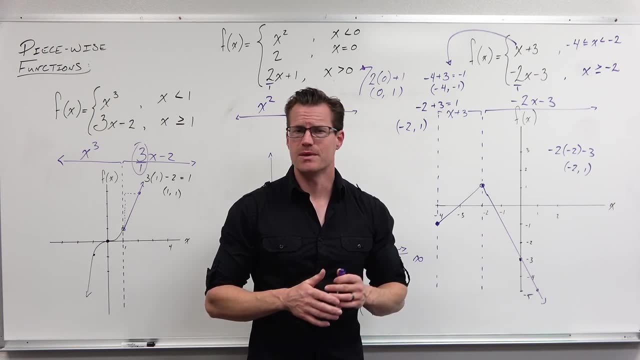 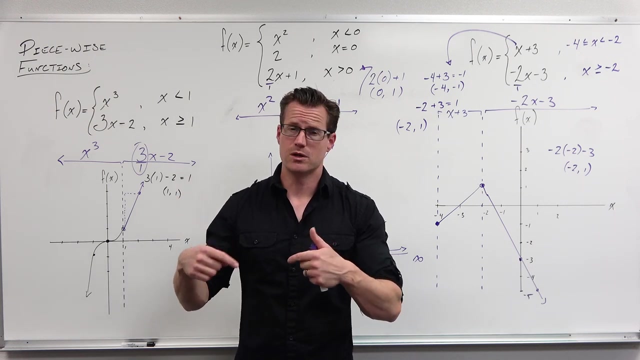 already previously filled in with this output. That's the way this graph would look. I hope that I've explained piecewise functions to you and how you approach them. How you approach them is you look at your domain. Your domain tells you when to use each piece of the function when you're. 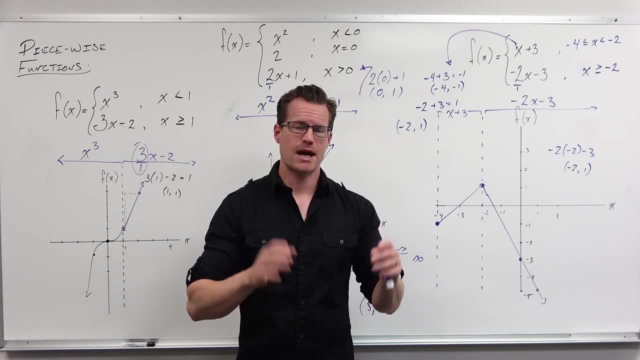 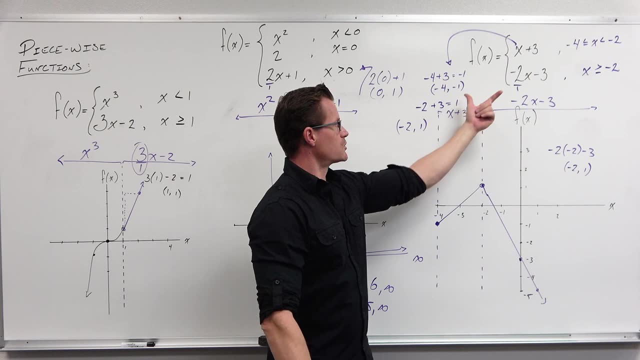 evaluating values. It also tells you the intervals on your x-axis for which your piece is defined, And so, when we look at it, your domain breaks up your x-axis. It shows you when you use each individual piece, Plug in or evaluate your boundary markers, your boundary values, your